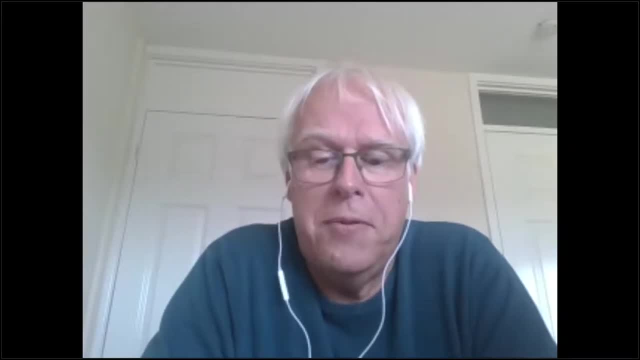 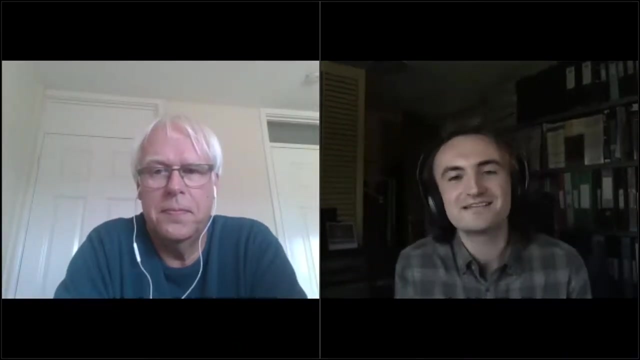 Before I welcome our two speakers, I would like to invite Dan Evans to give a brief introduction about the Society and the host and today's meeting, Dan, over to you. Thank you, Wilfred. The British Society of Soil Science is an established international. 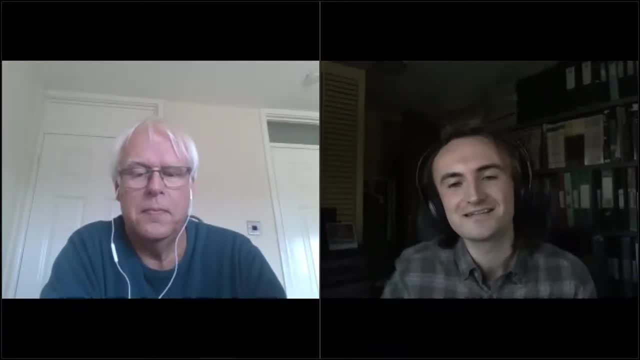 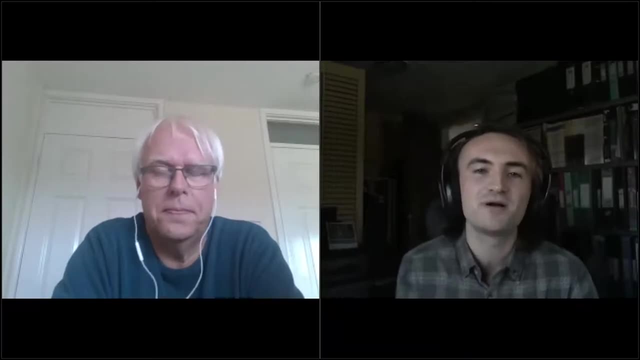 membership, organisation and charity committee to the study of soil in its widest aspects. We bring together those working within academia and have a growing membership amongst practitioners implementing soil science and industry and those with a keen interest in soils. Next month we won't be running a Zoom into Soil event, but we'll 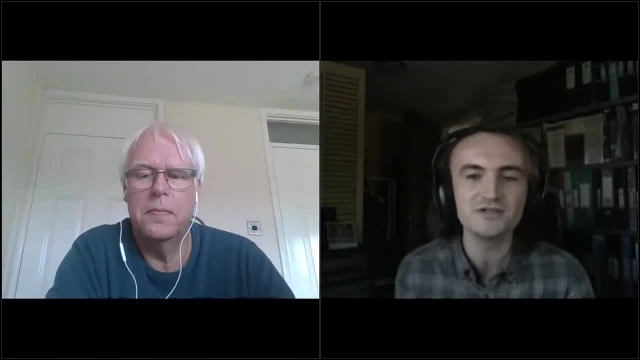 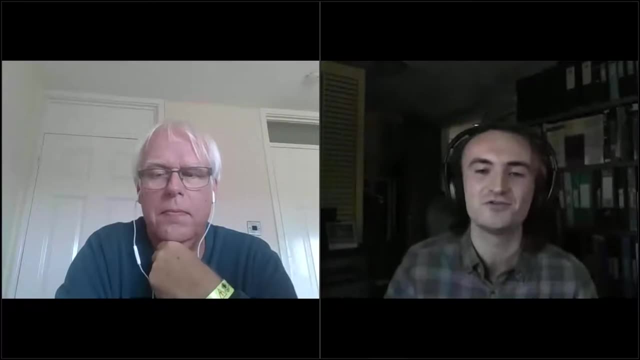 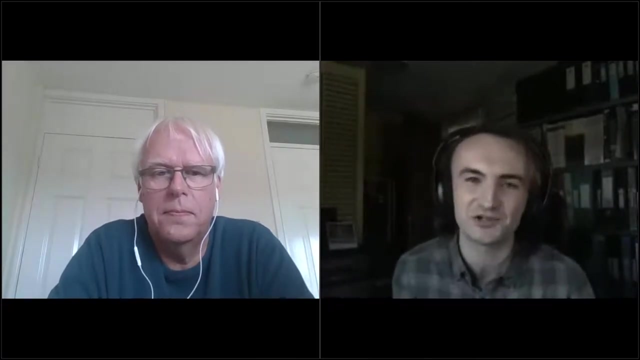 be highlighting the importance of soil to teachers and students in a virtual event hosted by Lord Lucas, and we'll be sharing the details on that on our social media channels shortly. Our final event this year will be our annual conference, Soil in Action, which will take 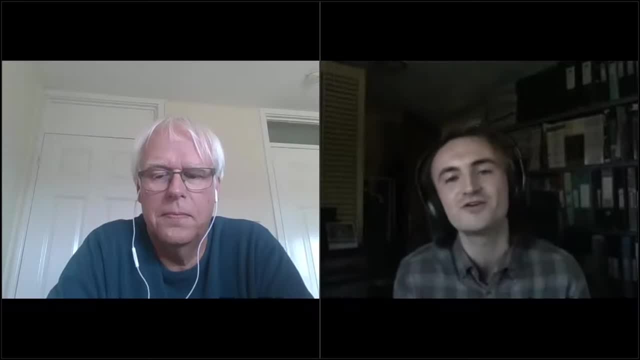 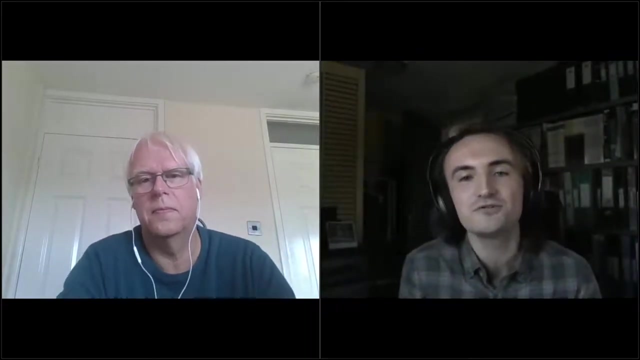 place on Friday, the 4th of December, and that will focus on the links between academic research and industry, And amongst the fantastic programme we have a forensic scientist and an environment manager from a major infrastructure company sharing their thoughts on the role that soil plays in their work. The conference is available free of charge for our members. 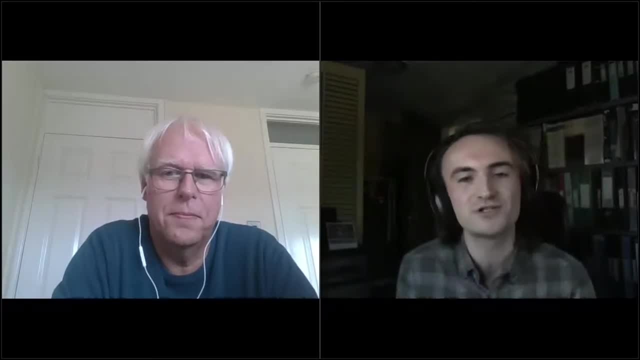 of BS Cubed and to find out more about the membership, which starts at 31st December 2021 pounds per annum. please highlight this in your response to the event survey. Next year, we'll be running 10 Zoom into Soil events. these events- and I hope that you'll 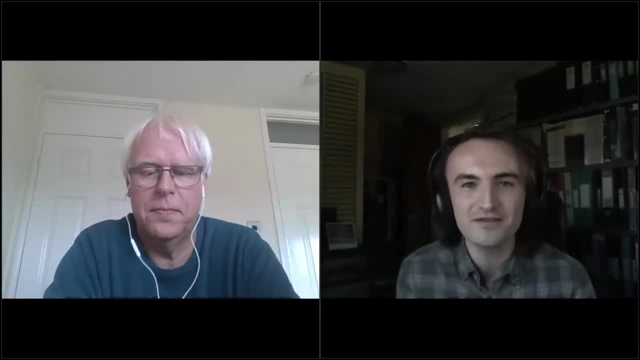 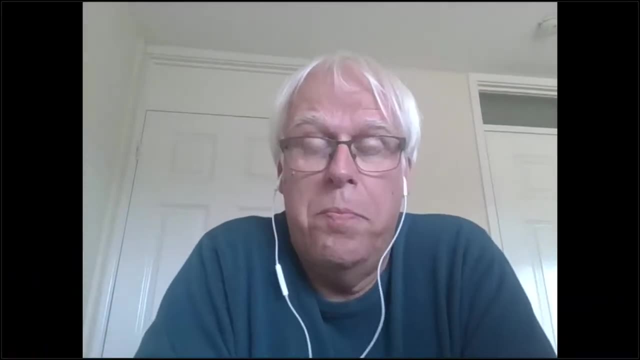 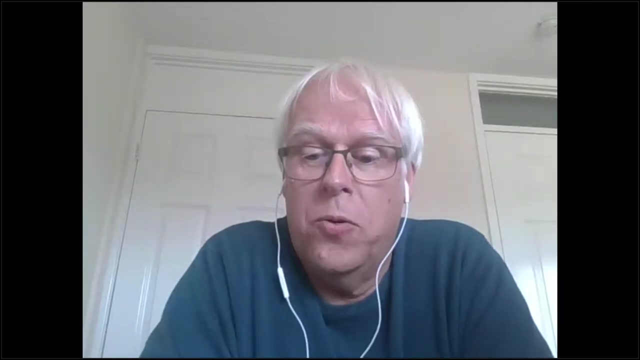 join us from January 2021.. So thank you for attending today and I'll hand now back to Wilfred. Thank you very much, Dan. So, before we begin this session, a few basic housekeeping, As there are so many of you today, all microphones: 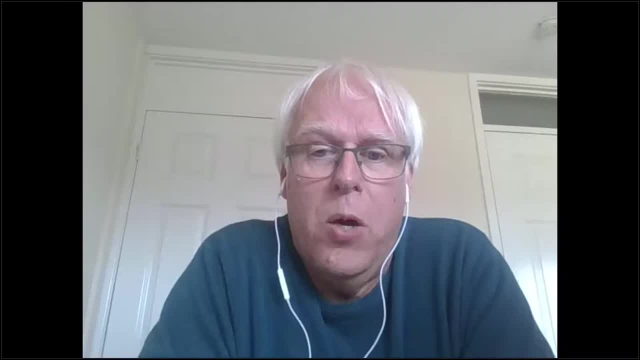 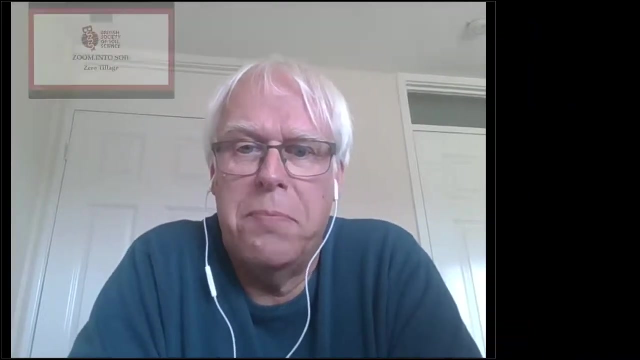 have been muted. You probably have already noted that We will be taking questions, however, at the end of both presentations And my colleague Dan will ask these on your behalf. So please could you submit any questions you have by 12.50, to allow us to get through as many as. 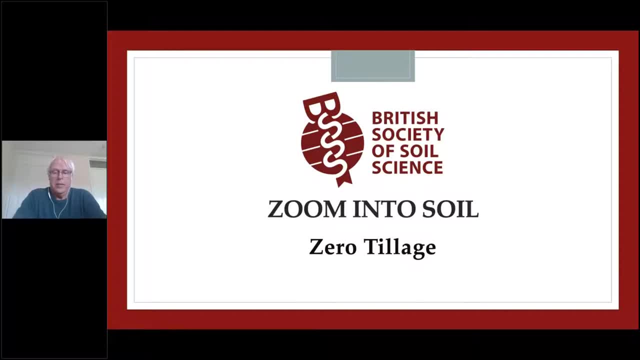 we can and organise them. Although there is a raise your hand button, we won't be using this unless the presenter specifically asks you to raise your hands. Today's presentation has also been awarded BASIS and NRO, SO CPD points If you are registered. 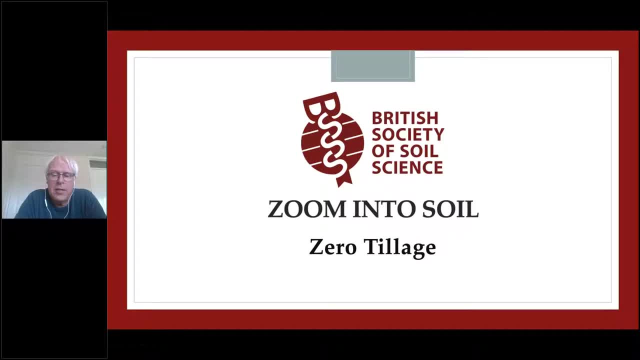 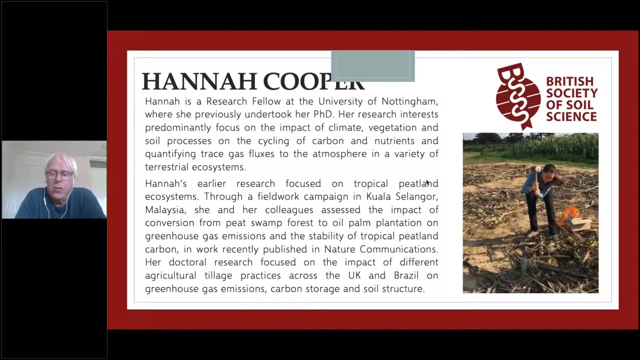 with either body. please contact us directly after the event. Finally, please be aware that we are recording today's presentation. I would now like to introduce our first presenter, Hannah Cooper. Hannah is a research fellow at University of Nottingham, where she previously 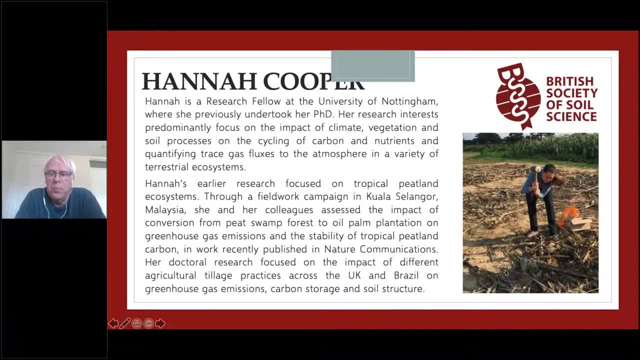 on the, took her PhD. Hannah is a research fellow at University of Nottingham, where she previously, on the, took her PhD. Her research interests predominantly focus on the impact of climate, vegetation and soil processes on the cycling of carbon and nutrients and quantifying trace gas fluxes to the atmosphere. 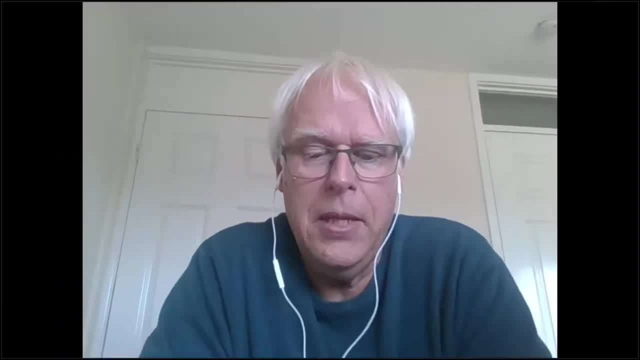 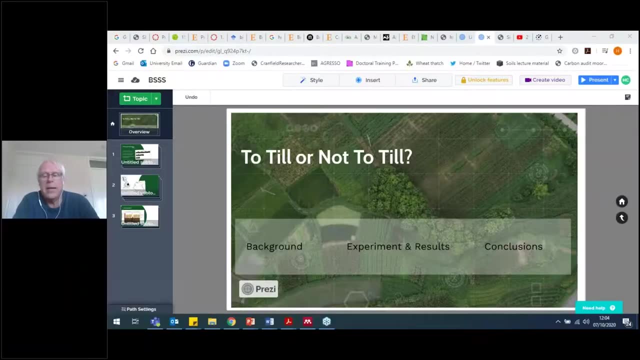 in a variety of terrestrial ecosystems. Hannah's earlier research focused on tropical peatland ecosystems. through a fieldwork campaign in Kuala Selangor, Malaysia, She and her colleagues assessed the impact of conversion from peat swamp forest to oil palm plantation on greenhouse. 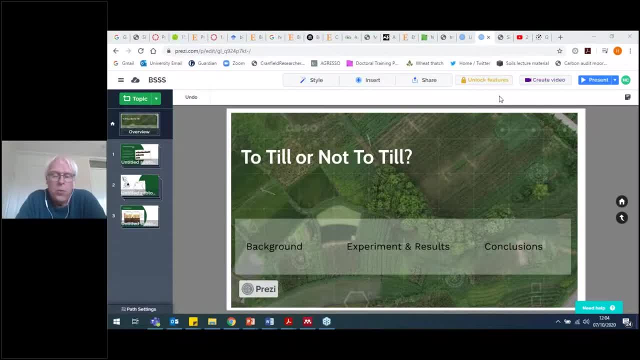 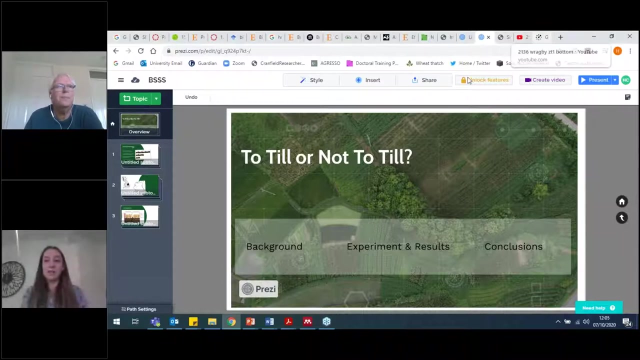 gas emissions and the stability of tropical peatland carbon in work recently published in Nature Communications. Hannah, we are very pleased that you are willing to share your views with us today about till or no. till and over to you. Hoi Wilfred, thank you very much for your introduction and inviting me to speak today. 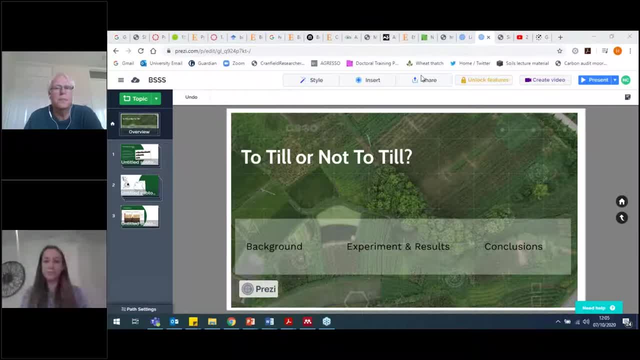 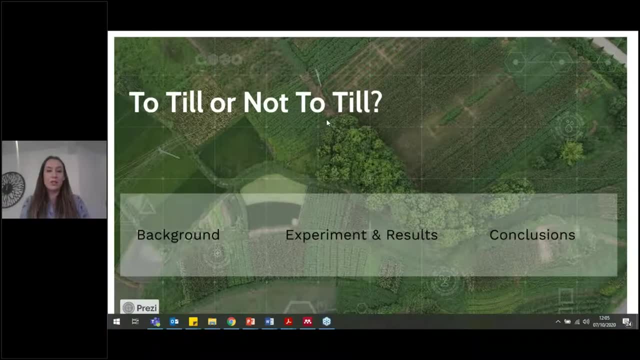 Thank you very much for your introduction and inviting to speak today. Can everyone see my screen? So the topic of my talk to? yeah, perfect. the topic of my talk today is to till or not till. This is due to constant discussion on Başekazan health, as you saw on the TV website yesterday. 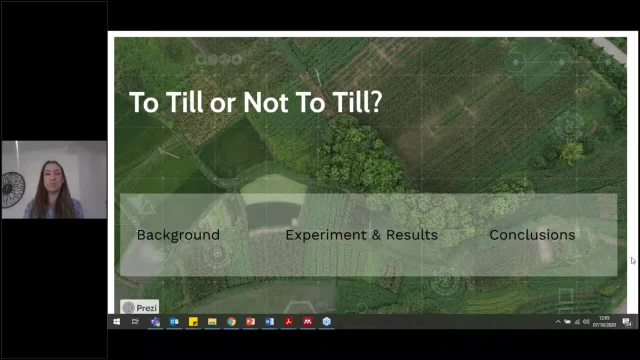 This is due to constant discussion on Başekazan health, as you saw on the TV website yesterday, And this is focusing mainly on my PhD research. My english is not a big deal in any way, but on my PhD research where I looked at the effects of zero tillage and conventional tillage on a 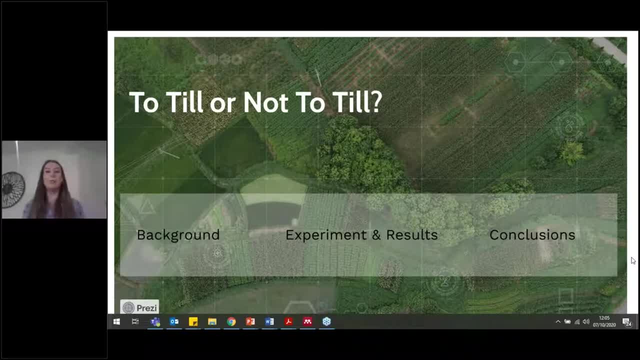 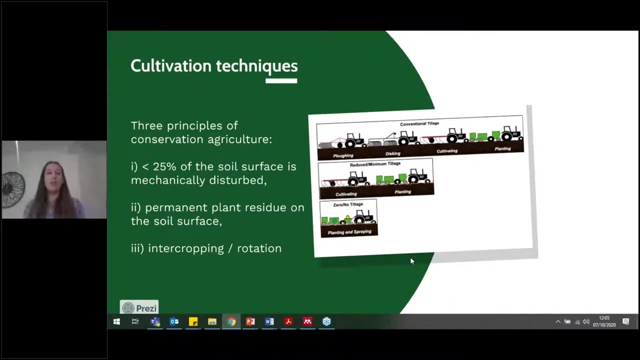 whole suite of soil properties and the potential implications of this for climate change mitigation within the area that I sampled. So just a bit of a background. So what do I mean when I refer to conventional tillage and zero tillage? So, conventional tillage- 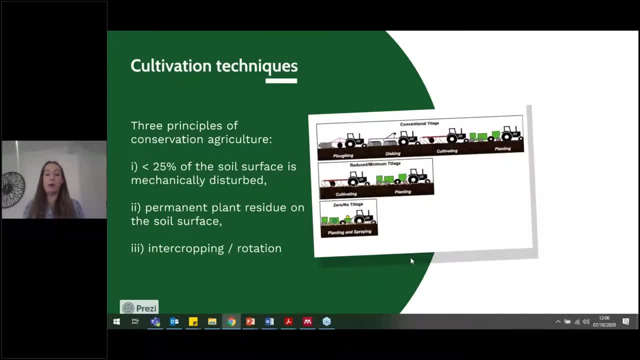 is also known as ploughing, and this is where a farmer will have a sequence of several passes across the same field to create a good seedbed and mechanically destroy any weeds. Now, during this process, the mechanical loosens maybe the top 20-30 centimetres of the soil. However, at the same, 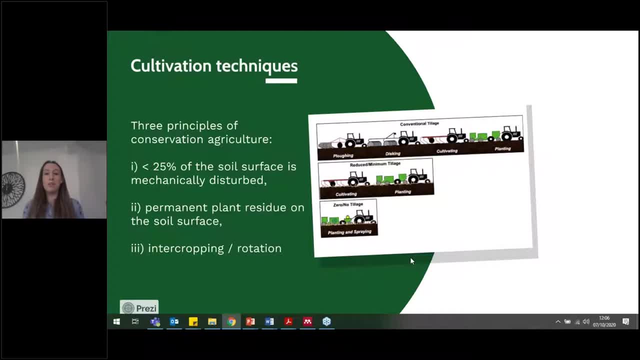 time. as we learned from Jane's session last time, this can cause huge problems for soil erosion. So in the 1930s and 40s the term coined conservation agroecology. It was introduced. There are three principles of conservation agriculture, and that is that. 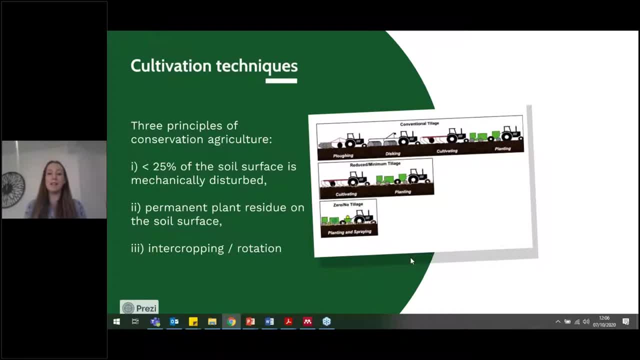 less than 25% of the soil surface is mechanically disturbed. There's permanent plant residue on the soil surface and some form of intercropping slash rotation. So my PhD focused on the extreme end of this conservation agriculture, which was zero tillage or no tillage, and that's where the farmer 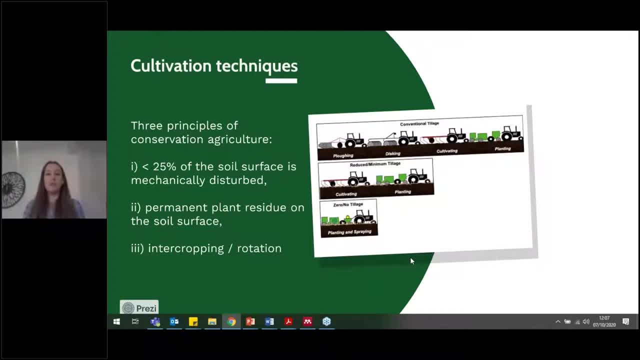 will pass over the field Maybe once or twice, and not disturbing the soil at all and just directly drilling into the previous crop residue. So there are quite a few things that we know about zero tillage already, Because you're only passing over the field maybe once instead of several times. there's 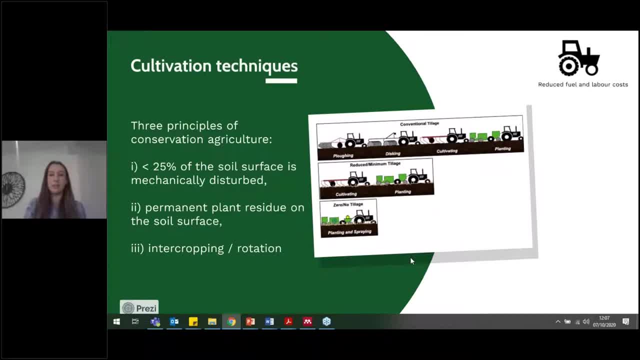 a reduced fuel and labour cost associated with zero tillage. You leave a permanent crop residue on the surface, so that gives your soil some protection from wind erosion and at the same time it helps with soil moisture conservation as well, because that crop residue on the soil surface it 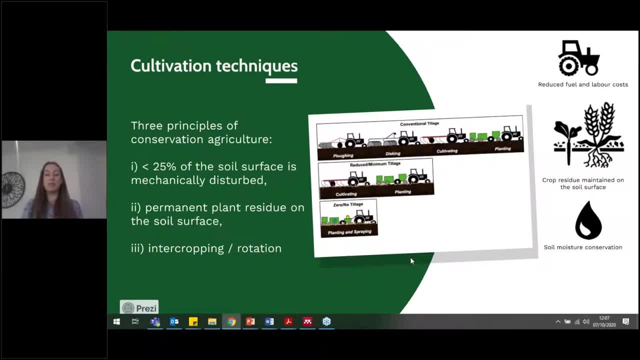 really retains that water, which will slowly infiltrate down through your soil profile, which is really important in the summer months. And lastly, you get an increase in biological activity as well. So some recent work done by Jackie Stroud at Rothensted showed the increase in earthworm. 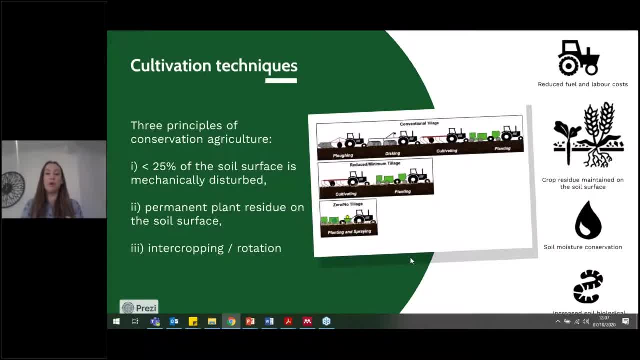 populations associated with zero tillage. There's special earthworms which are really deep burrowing earthworms which are really deep burrowing earthworms. So that's a really important thing. It's a really important thing to know about zero tillage and there's special earthworms which are 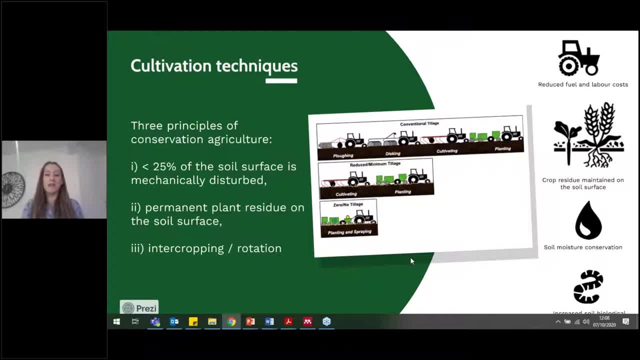 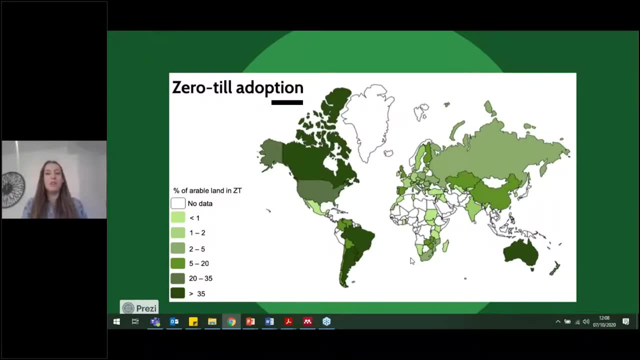 which are important in zero tillage And they can go down to two meters and their earthworm channels can be left to develop. So zero-till adoption across the world. you can see there's been a variety in uptake since it was introduced. 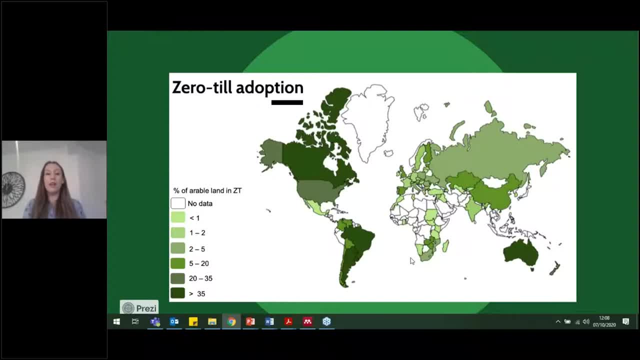 In North and South America and Canada you can see there has been quite a high uptake in adoption. So, for example, in Argentina, at least 70% of the arable land available is in some form of conservation agriculture, And this is primarily due to the policy implications. 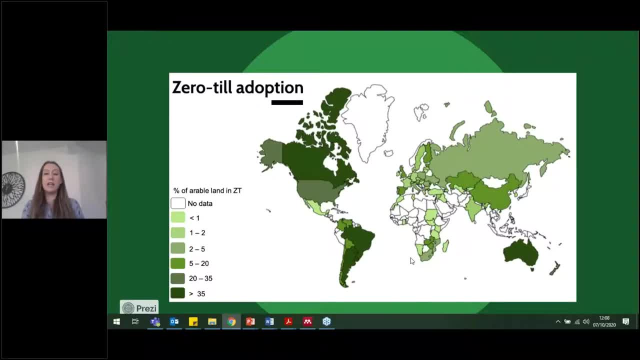 So there's subsidies for farmers, there's meetings every year where at least 2000 farmers meet, So there's good dissemination of information. However, if you look at the other extent- so on the African continent, where data is available- the uptake hasn't been quite so high. 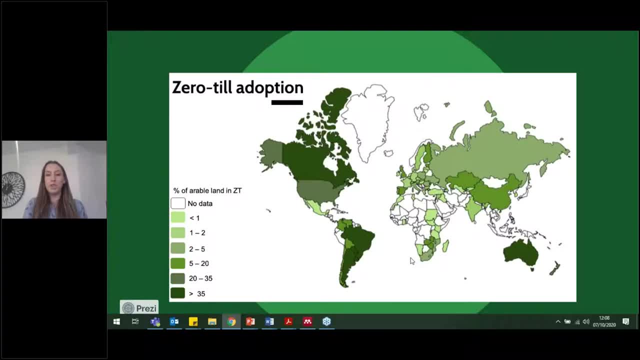 And this is primarily due to the completely different types of farming out there. So a lot of the farming is subsistence farming, So the farmers need the crop residue at the end for animal feed or for fuel. So uptake has been relatively lower across Africa. 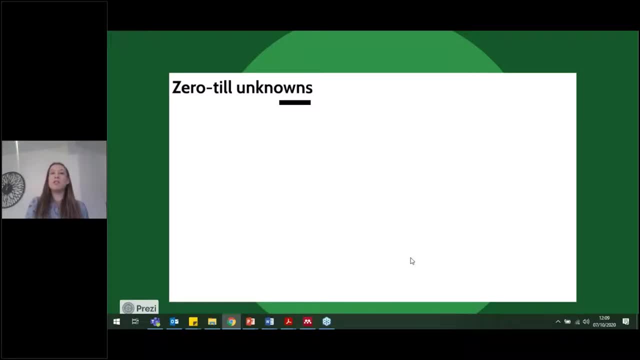 So there's quite a few benefits that we know about zero-tillage. Generally it's good for soil health, but there's still quite a few things that we don't know when it comes to zero-tillage. So, firstly, nitrous oxide emissions. 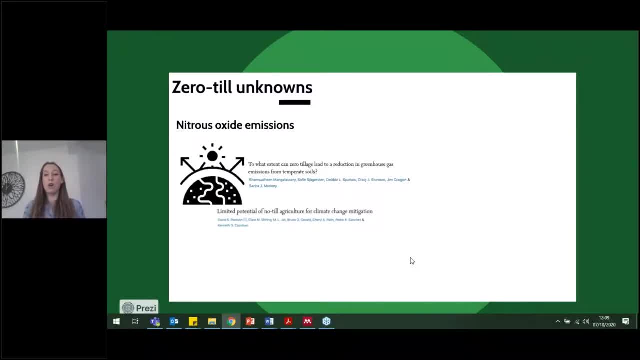 or N2O. So we know zero-tillage can reduce your carbon dioxide emissions Because it's not being mechanically disturbed. it doesn't the oxygen doesn't get into the profile and oxidize the carbon into carbon dioxide. However, zero-tillage does also create a perfect environment. for an increase in nitrous oxide emissions. Now, nitrous oxide is about 300 times more potent than carbon dioxide, So in terms of your greenhouse gas balance, which management is better? Zero-tillage, which may reduce CO2, but increase N2O. 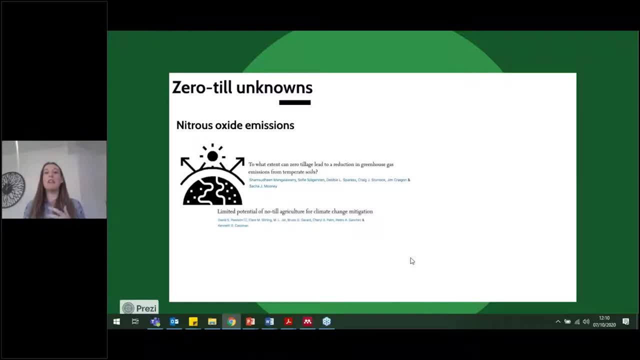 or conventional tillage, which has a lot of CO2, but less N2O. Heavily debated in the literature as well is carbon sequestration. So some studies only go down and measure to 30 centimeters, But we all know that root systems do go below 30 centimeters. 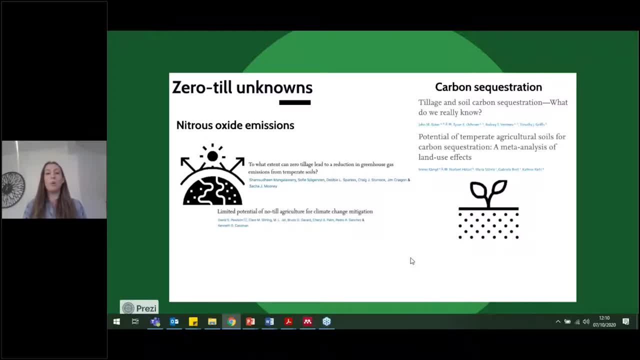 to store carbon and release root exudates and things Also. some studies don't take into account the bulk density changes that you get associated zero-tillage and conventional tillage. So some studies may have a very overestimated the potential of zero tillage to store carbon. And also a crop yield. This is a big one in terms of a lot of this. literature suggests that maybe crop yield declines within the first five years of converting to zero tillage. and in terms of crop yield in double estimates- global food security and economy for the farmers. this just isn't feasible. 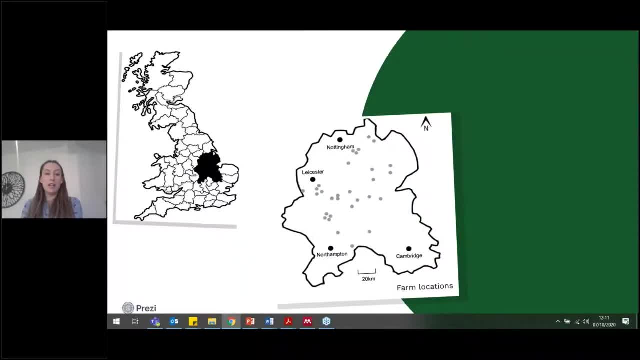 So the first experiment of my PhD was based in the East Midlands and I went to 160 fields. So within these fields were 80 pairs of conventional and zero-tilled fields, and this image here on the right is what I mean by a pair. So you've got a zero-tilled field right next door. 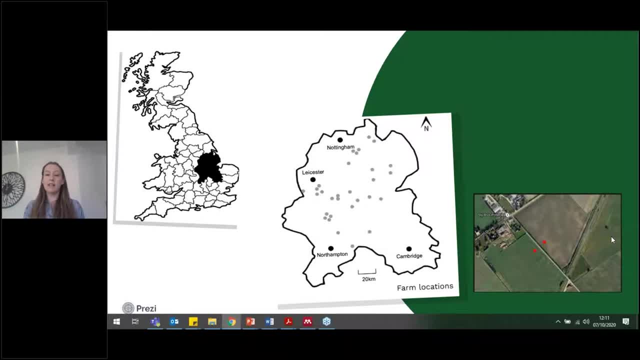 to a conventionally tilled field. so everything is exactly the same: the soil texture, the amount of rainfall, the air temperature, but the only difference is the management in which the soil is under and the image in the middle you can see here I went to. I never took more than three pairs. 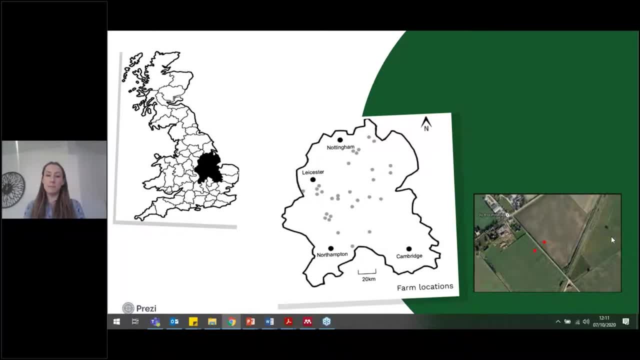 from each farm. so these are the locations of the different farms, and I went to 32 farms in total. Sampling took place across November, December time, so that was lovely and warm. and then this was when, one to two months after, sowing had been completed, so the structural changes associated with root growth were at a minimum. 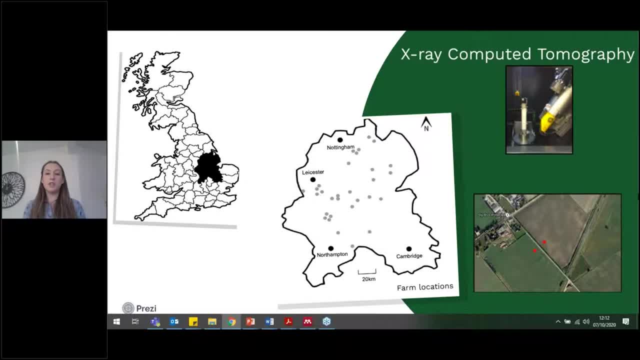 Some of the sampling and methods involved. I took an intact soil core, so that goes down to about 30 centimeters, five centimeters wide- and then these are carefully taken back to the lab and measured using x-ray computed tomography. so if anyone's ever broken a bone and gone to hospital, it's basically the same principle. 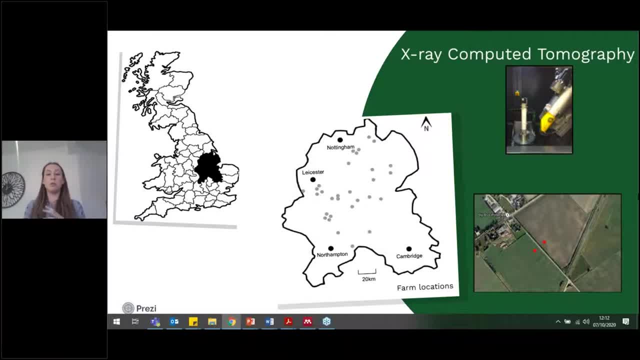 in that x-rays go through the sample and there's a detector at the end to see what's been absorbed or where the x-rays have gone straight through From these same cores. I could then incubate them at 5,, 10 and 15 degrees to get greenhouse gas emission potentials. 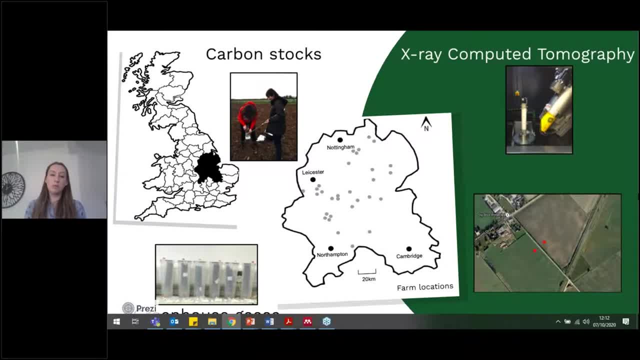 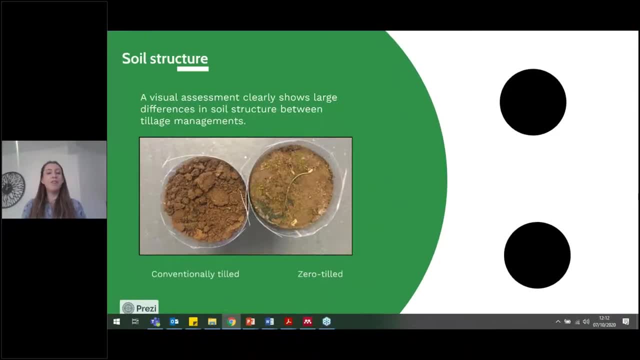 and we also measured carbon stocks, taking into account the changes in bulk density and down to 50 centimeters. So here we've got some examples of some results. so, firstly, soil structure. So on this image here, this is an example of a pair of cores, so they're taking no more than 10 meters. 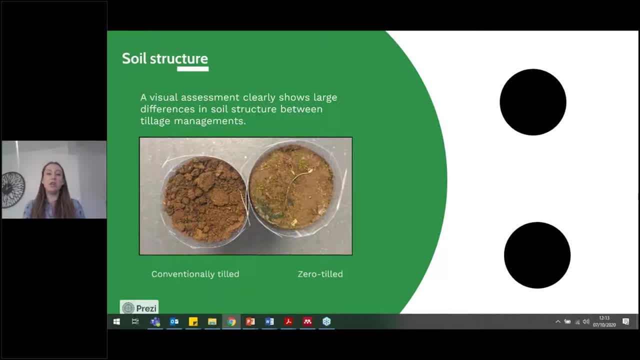 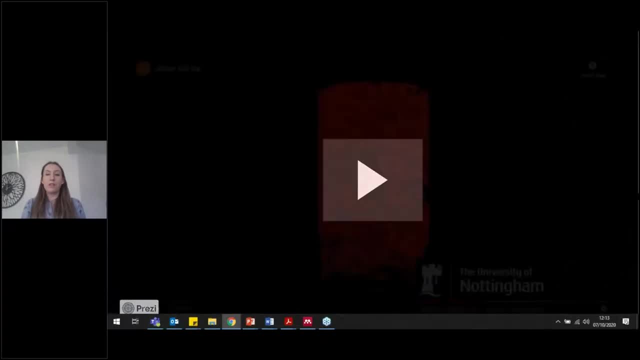 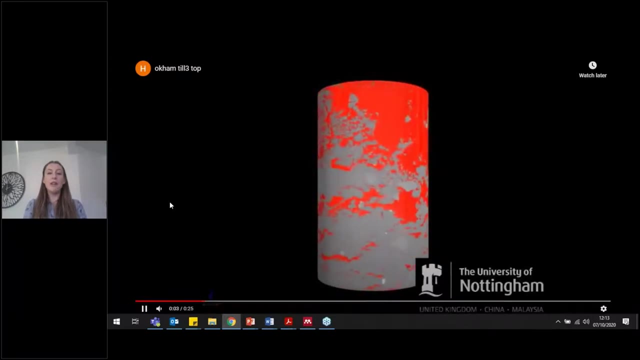 apart. but even with the naked eye you can see there's going to be huge structural changes associated with the two managements And through x-ray CT we can see the different structural changes. So the grey material is the soil material and then the red is the soil pore. 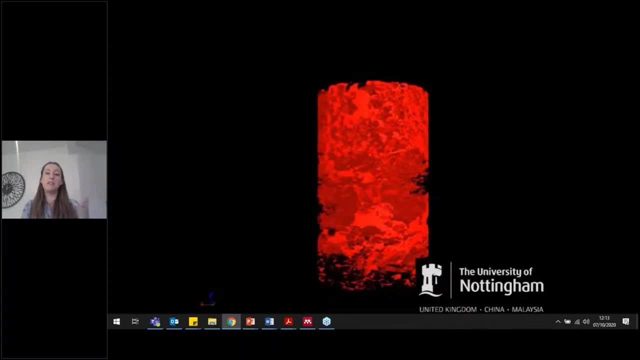 And you can see here. this is a conventionally tilled soil. where it's been mechanically disturbed and turned over, it's mainly full of pore spaces, which are going to be a problem when it comes to soil erosion. there's nothing holding the soil together. We then look at zero tilled soils again. this is a pair, so, taken just a few meters away, you can see. 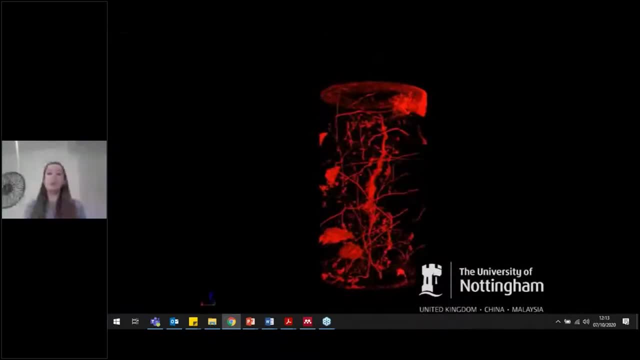 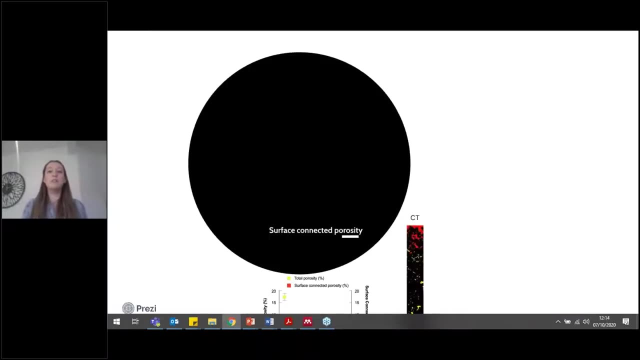 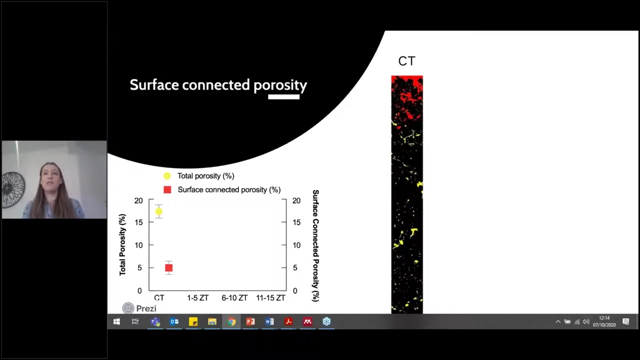 a huge difference. You've got your root channels and your biopore channels here, which have been left to develop over time, But what does this mean in terms of implications for farmers? So I also measured something called surface connected porosity. So say, for example, you have a root channel which starts at the surface and goes halfway down your core. 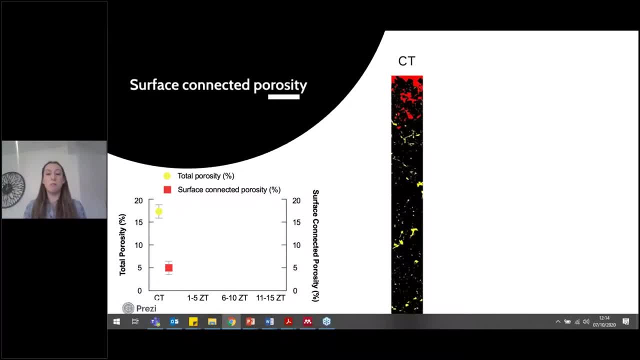 This pore is connected to the surface in some form, so that's what it measures. This is an example of a conventionally tilled core. You can see the total porosity is quite high, about 17 percent, and the surface connected porosity is limited to maybe the top four centimeters. 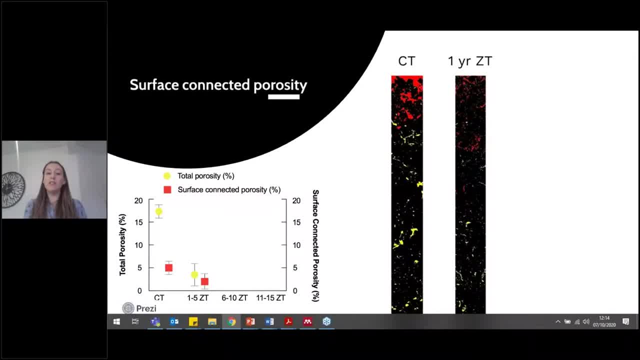 One year under zero tillage and the story actually looks a little bit worse. You've got soil which has been consolidated for a year. it's not had that mechanical turnover. the total porosity actually declines. But give the soil a second look. You've got soil seven years under zero tillage and you start to see a kind of regeneration of the soil structure. 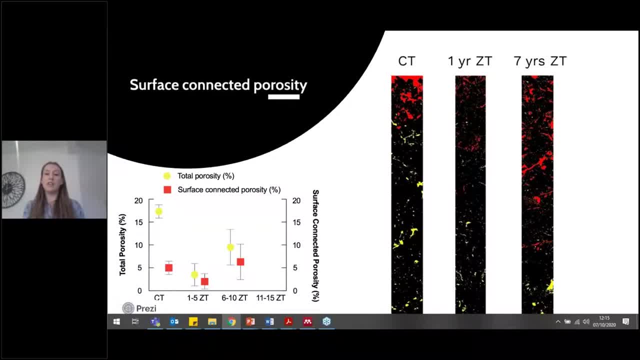 And the surface connected, porosity increases and you can see it moving further down the soil core. And then again give it 15 years under zero tillage and you can see a huge improvement. and this is going to have implications for farmers in terms of infiltration and gas exchange. 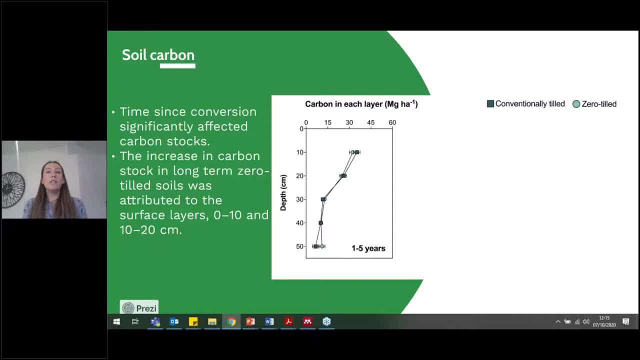 I also measured soil carbon. So one thing that was fortunate in terms of sampling so many fields, I was able to get a range of soils which had been in zero tillage for a different length of time. So some had been in zero tillage for one year, some had been in zero tillage for 15 years. 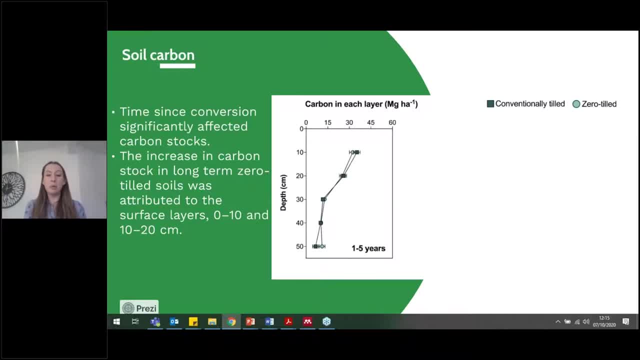 And this is often a discussion that's not had- is the temporal effect, because obviously soil changes are slow processes to happen. So if we have a look here at soil carbon, you can see after one to five years there's no real difference between the two managements. 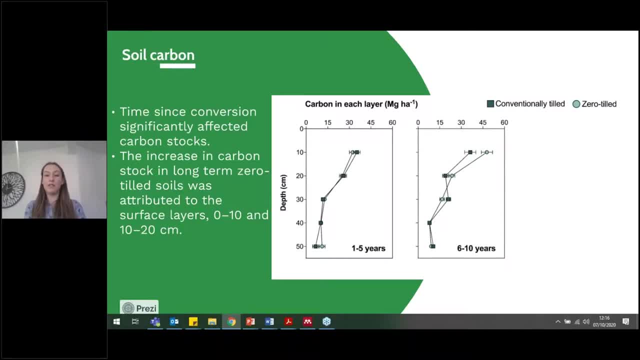 But give it six to ten years and because you've got that crop residue left on the soil surface, there was a significant difference in the surface carbon content between the two managements. Give it 11 to 15 years and there was a significant difference between 0 to 10 centimeters and 10 to 20 centimeters. 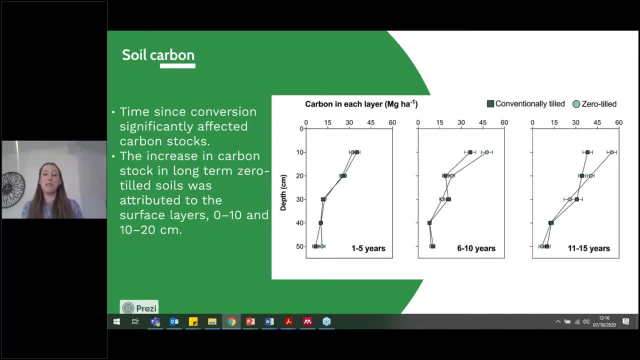 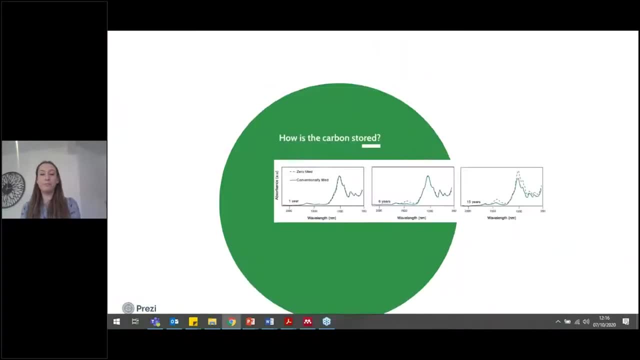 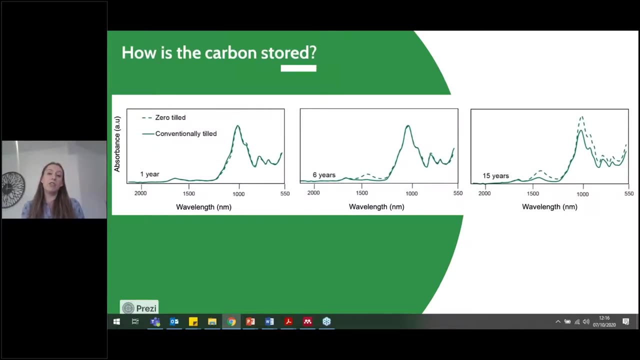 Overall, throughout the whole profile, down to 50 centimetres. it meant that zero tillage did actually store more carbon than the conventionally tilled soils. But how was the carbon stored in the soil? So some literature suggests that even though zero tillage may store more carbon in the surface, is that going to be readily oxidised and turned into CO2 after a heavy rainfall event or something like that? 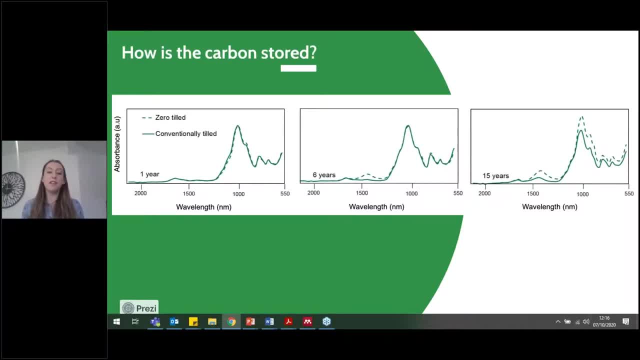 So a quick and easy analysis I undertook was FTIR, and this looked at the organic chemistry of the carbon stored within the soil profile. So if you look at this image here on the left, this is the pairs which have been in zero tillage for one to five years. 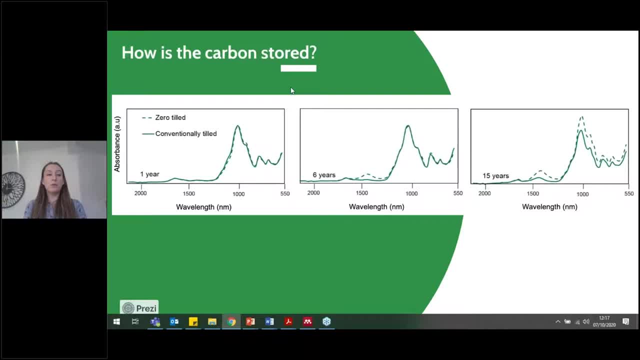 Zero tilled soils have got the dashed line and conventionally tilled soils have got the solid line And you can see that there's no difference between the different types of carbon that's stored in the soil. After six years- the pairs of zero and conventionally tilled soils- you can see a bump here and there was an increase in the aliphatics. 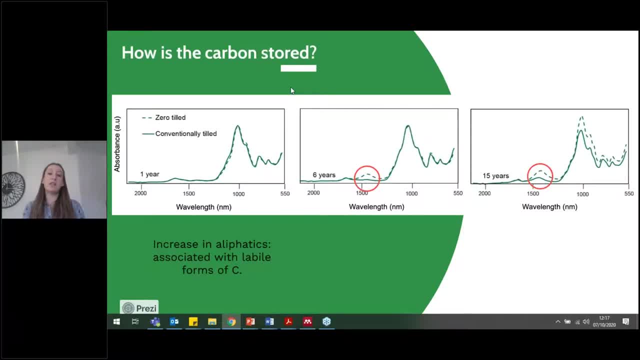 And these are associated with labile forms of carbon, So these are readily available to your earthworms and microbial organisms to use. And then, moving over to this side, you can see an increase in ethers, which are compounds of intermediate recalcitrance. 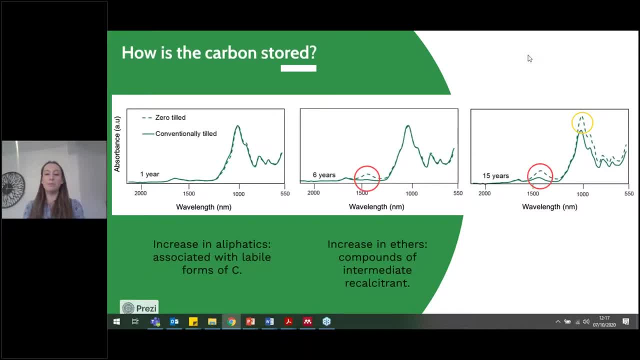 So the soil is starting to hold on to that carbon a little bit more And again, after 15 years, you can also see an increase in aromatics, which are enhanced microbial stabilisation of organic materials. So it's going to take a lot of movement or a lot of activity for that carbon to be accessed and turned into carbon dioxide. 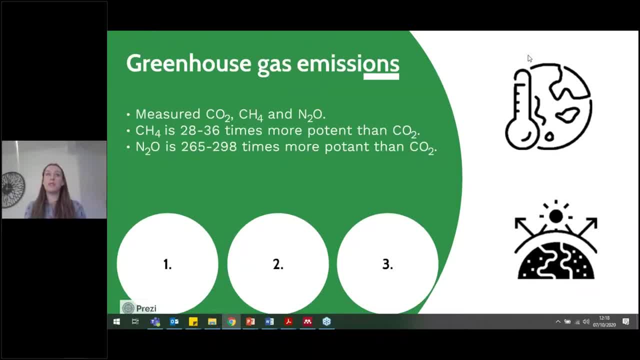 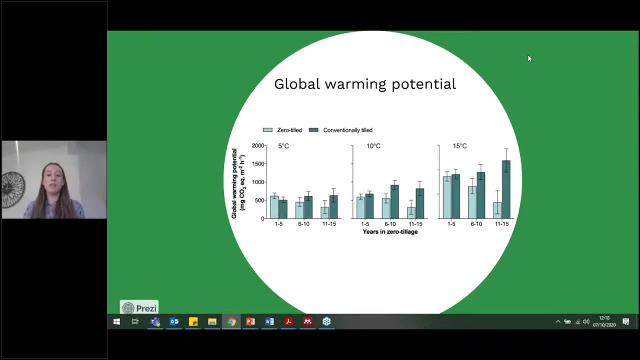 So then I also looked at greenhouse gas emissions, because if the overall carbon content was increasing in the samples that I measured what's happening to the greenhouse gas emissions. So I measured carbon dioxide, methane and nitrous oxide, And using those three you can create something called the global warming potential. 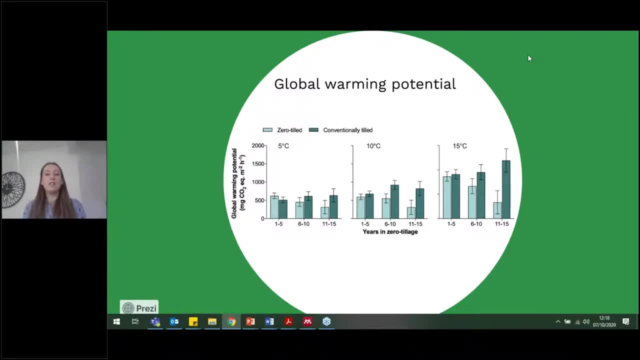 So it takes into account the potency of each gas And you can see a really interesting trend that's been driven out through doing this. So if we take an example of 15 degrees, 1 to 5 years, there's no real difference between the two treatments. So if we take an example of 15 degrees, 1 to 5 years, there's no real difference between the two treatments. So if we take an example of 15 degrees, 1 to 5 years, there's no real difference between the two treatments. 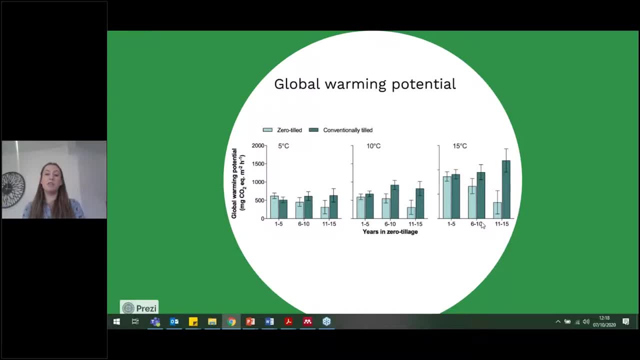 After six to ten years, the zero-till soils had a 30% lower global warming potential than their paired conventionally tilled soils. So the larger a global warming potential, the worse that is for your environment. And again, after 11 to 15 years, there's now a huge difference and the global 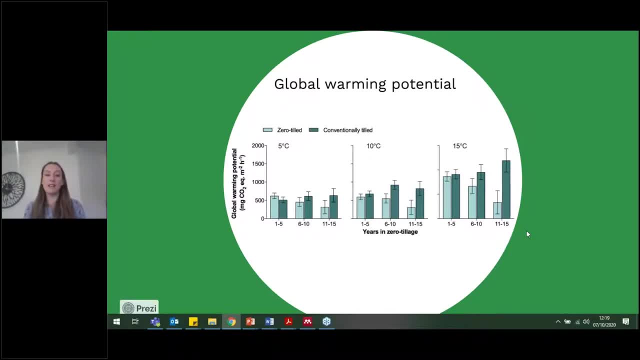 warming potential coming from the zero-tilled soils is actually 70% less than those paired conventionally tilled soils, And because I've measured them at the increments of 5,, 10 and 15 degrees, we can also look at something called temperature sensitivity and it gives you. 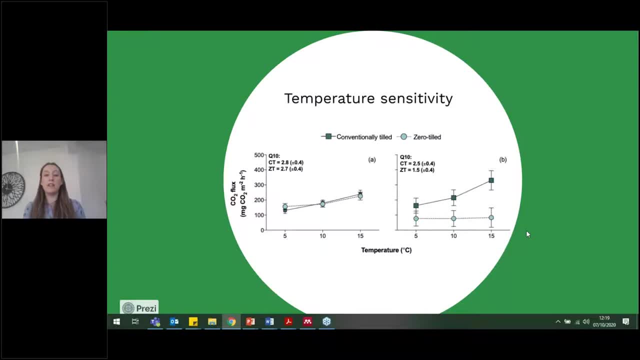 something called a Q10 value, which shows the soil respiration after a 10 degree increase in temperature. So this is starting to look at the future of the soils, So under future climate warming. So how are the soils going to react under these managements? 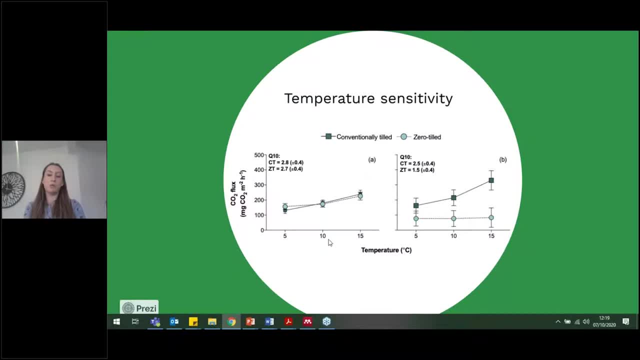 So in the one to five years- here you can see there's no difference in the Q10 value between the soils. But in figure B, here this is again after 11 to 15 years and you can see the conventionally tilled soils are reacting a lot more to an increase in temperature. 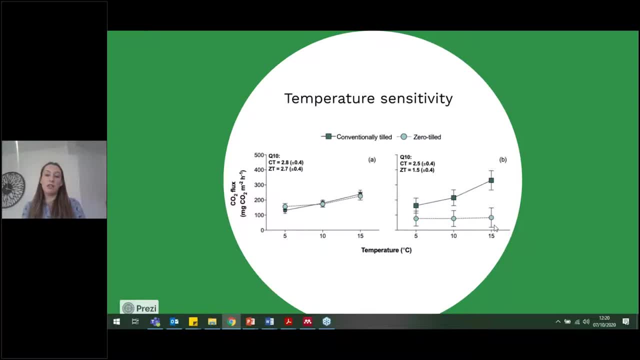 So at 15 degrees. you can see here this zero till Q10 is quite low, So that means an increase in temperature. the amount of greenhouse gases that the soil is going to release isn't to the same magnitude as the conventionally tilled soils here. 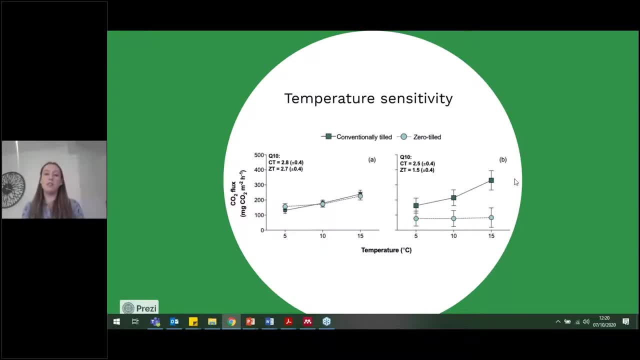 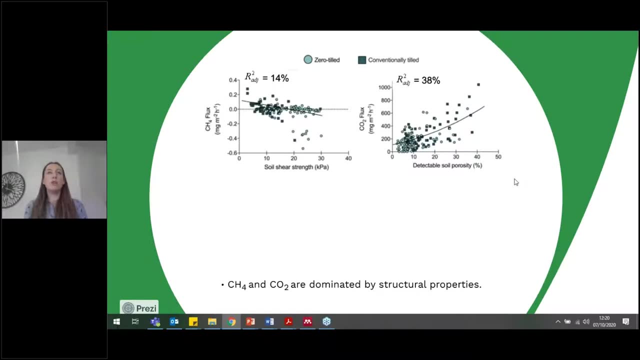 And again that's due to the carbon being held on a little bit tighter than the FTIR data we saw earlier. But then I also looked at what is driving these gases in these soil columns. So because we were able to scan the columns and do green gas analysis, we were able to get a better impression of the soil. 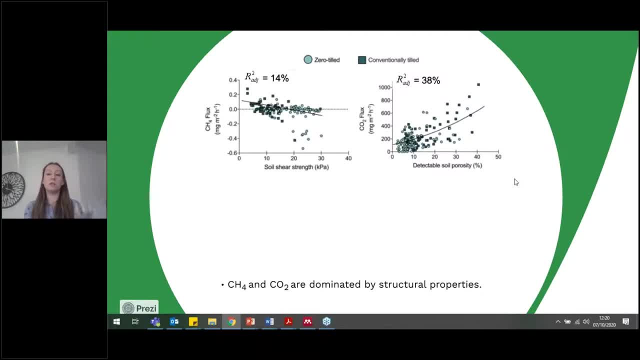 greenhouse gases. on exactly the same sample, we can link the soil structure and other properties to the gas emissions. so you can see here the methane and carbon dioxide are dominated mainly by structural properties, and you can see here that the detectable soil porosity measured using x-ray ct accounted for 38 percent of the carbon dioxide fluxes, whereas on the other hand, n2o. 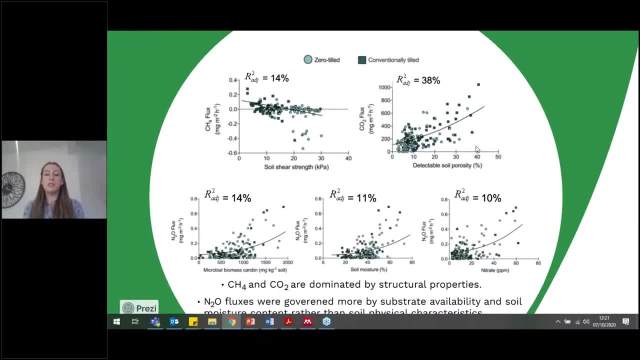 fluxes were governed more by substrate availability and soil moisture content rather than the soil physical characteristics, so this could be something quite interesting in terms of future management of zero tillage. so, yes, n2o might be a little bit higher from zero tilled soils, but in this example here, from my results, nitrate 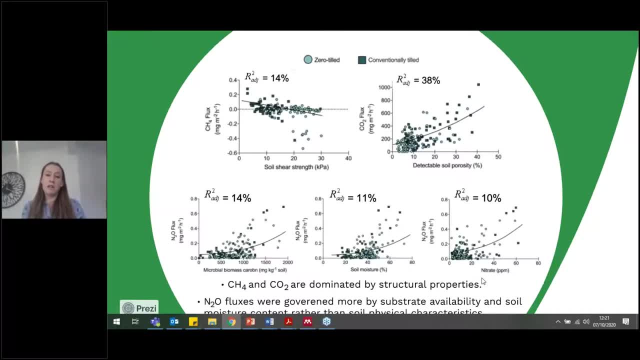 accounted for 10 percent of n2o fluxes. so if we have maybe slightly better management of nitrate in terms of timing of inputting fertilizers, the right amount etc. we might be able to bring the end fluxes down even further from zero tilled soils. so that was a little snapshot of what 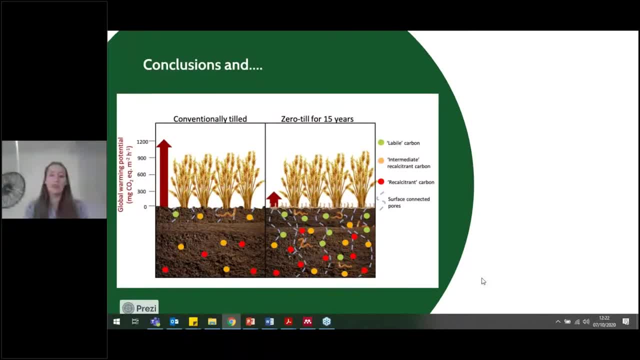 i got up to during my phd, and here's a graphical abstract. um so we know already that zero tillage increases your earthworm population and these are really beneficial in creating your surface connected pores here, which also help break through the plow pan that's been established. 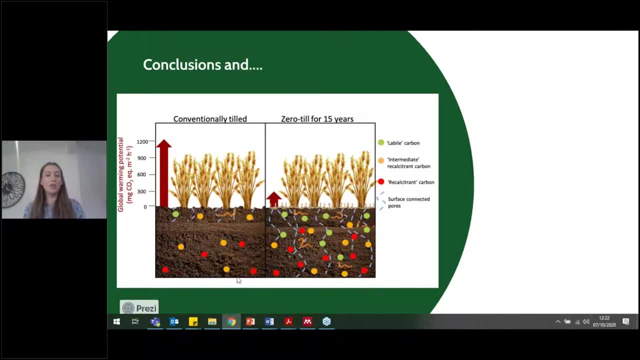 through conventional methods. you've got a different range and more of the carbon stored in your soil here, and the global warming potential is significantly greater from the conventionally tilled fields. so the higher global warming potential, the worse that is for your environment. but after 15 years this 10.5 percent of n2o fluxes are going to increase your earthworm population. 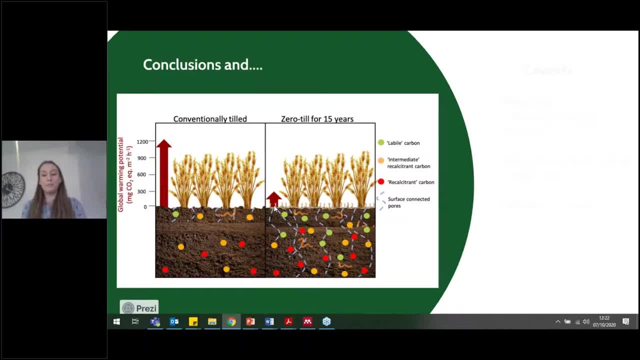 and you're going to be able to bring the n2o fluxes down even further from zero tillage. and you're going to be able to bring the n2o fluxes down even further from zero tillage. and you're going to be able to bring the n2o fluxes down even further from zero tillage. 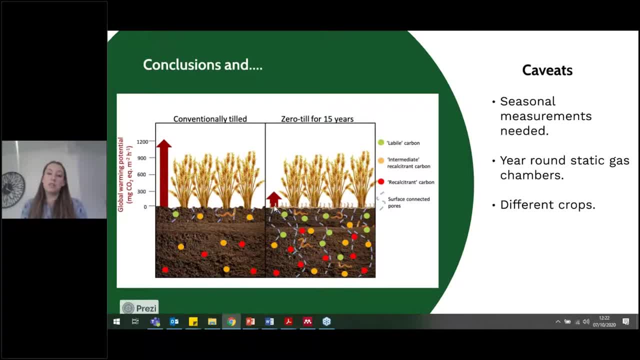 now, of course, with any experiment there's caveats. so i was able to carry this experiment out over november, december, because our question was to look at the soil structure. however, for the gases, of course, you need seasonal measurements as well in year-round static gas chambers and, unfortunately, 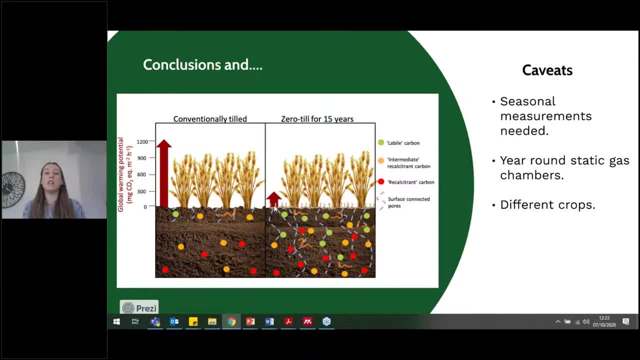 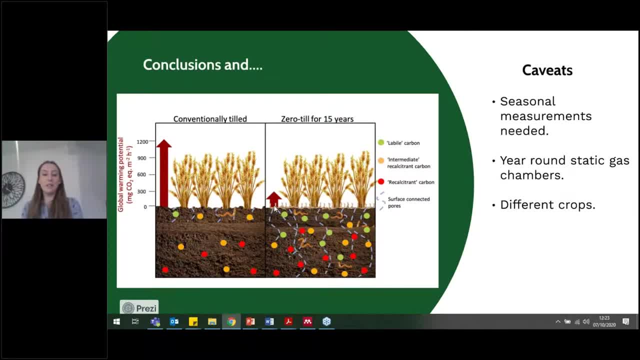 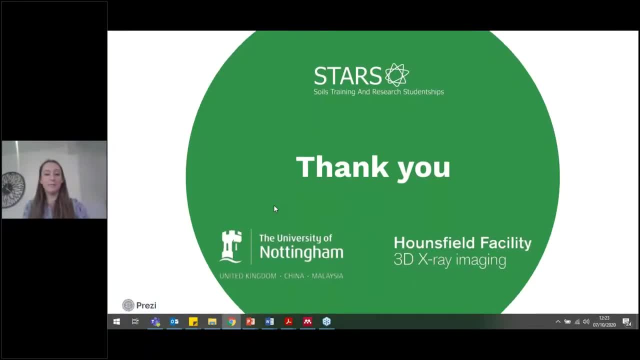 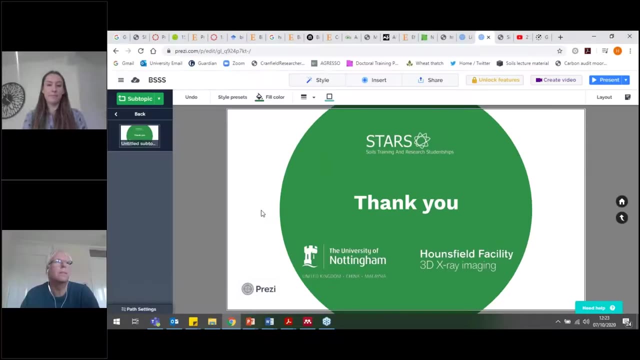 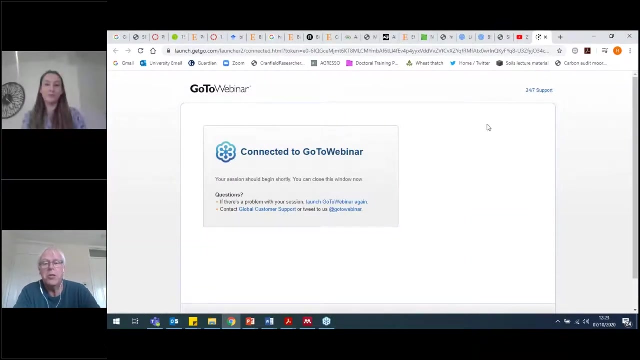 important component that needs to be looked at with zero tillage. so thank you for your time. i'll hand you back to wilfred and look forward to your questions. okay, hannah, thank you very much for, i think, a very interesting and nice presentation, and thank you also for literally showing us the inside of soil. that was very 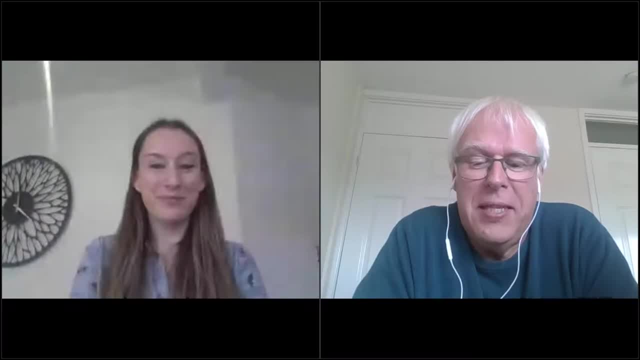 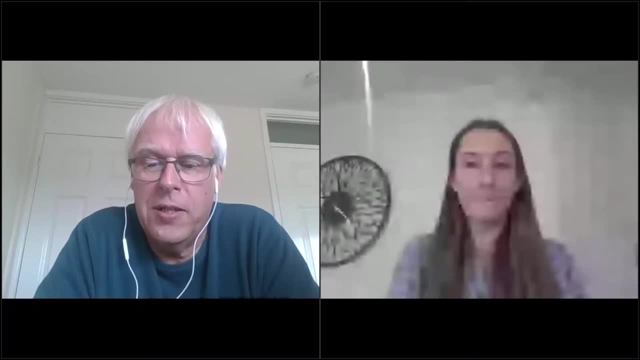 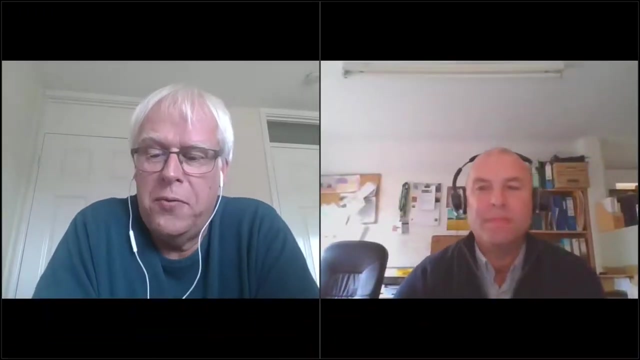 nice and very spectacular differences. so we'll be taking questions at the end of both speakers, as mentioned before, but please start typing your questions so we can start identifying the most common questions that are being asked by you. i'm very pleased now introduce our next speaker, russell mckenzie. russell is a farm manager for john's here farms on the cambridgeshire. 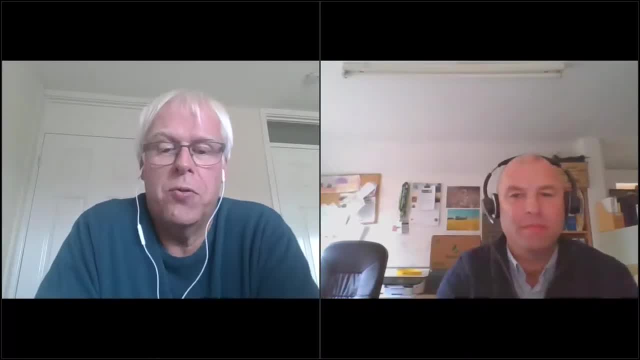 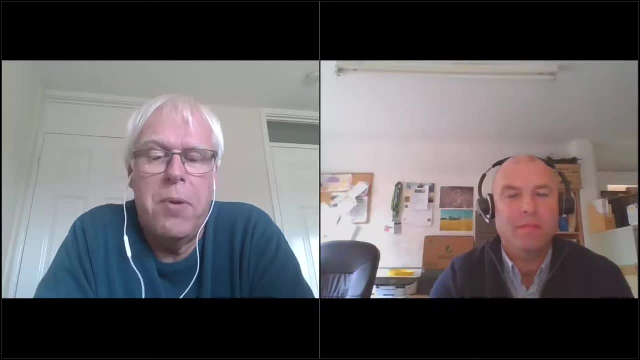 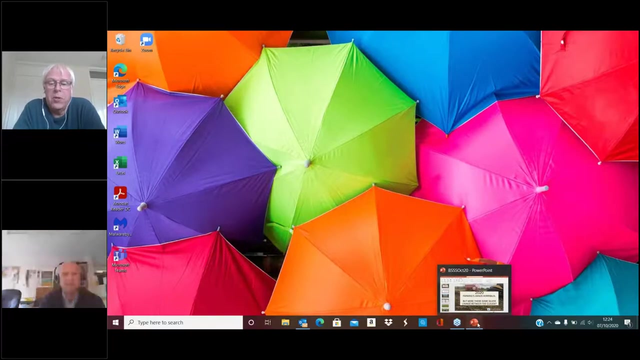 bedfordshire border, a predominantly heavy clay soil type across 995 hectares, four units of cropping including winter wheat, oil seed rape, winter beans, spring wheat, spring barley and spring oats. a 2040 northfield scholar researching success with no till under any conditions saw him travel to australia new. 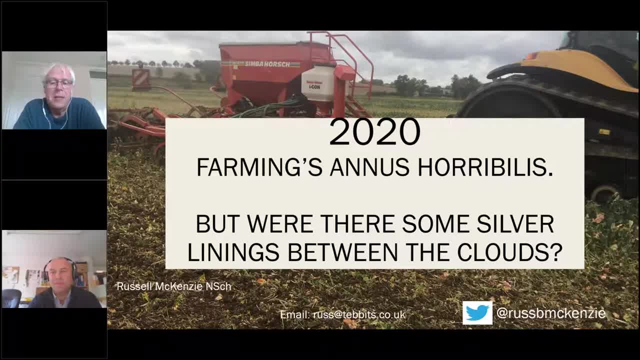 zealand, united states, brazil, argentina- to visit some of the best no-till practitioners in varying extreme climates across the arid climates to gain a better understanding of how to make no tillage work in both wet and arid climates. following his scholarship, russell has been introducing no-till. 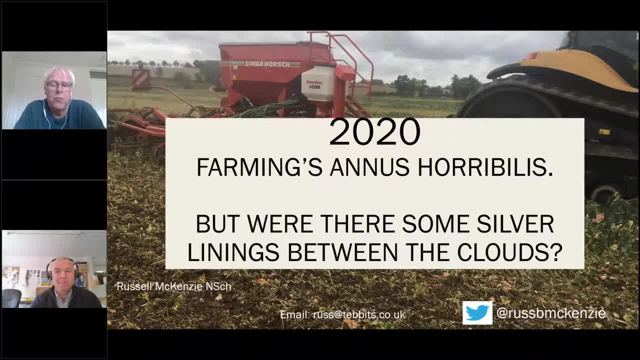 practices across the farms he manages. russell also sits on the cereal and oil seat board for ahdb as a grower member and attended the no-till on the plains conference in wichita kansas back in january to further research the benefits of conservation. 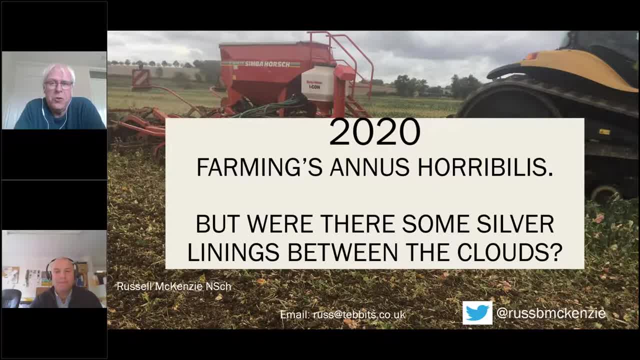 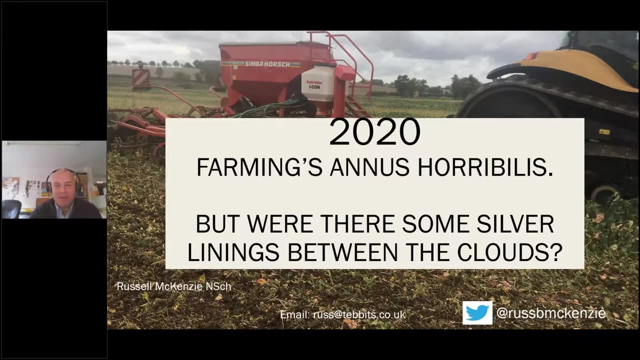 in agriculture Be very interesting to hear your side of the story, Russell, over to you. Thank you very much, Wilfred, for that introduction. it's a pleasure to come and speak to you today, but also equally, it was great to listen to Hannah, who did come and do a study on our farm as well. so 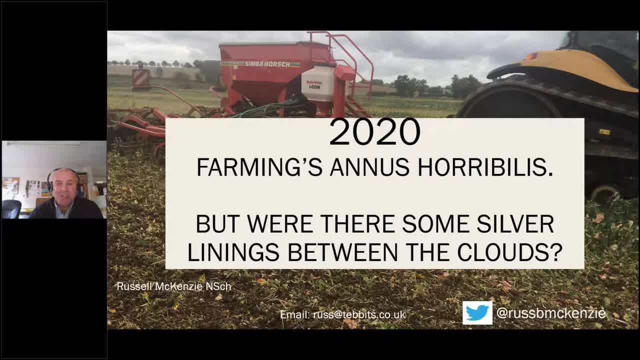 it was great to see her results off the back of it and some really interesting stuff. So mine's going to be slightly different. so I'm going to sort of do a bit of a review of what I describe as farming and as horribleness from last year. So a really, really difficult season. we had a very 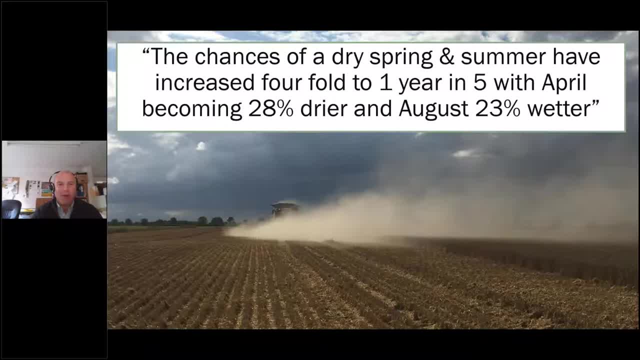 wet autumn last year and then a very dry spring, and I found it quite ironic that I spoke at a few meetings last spring in sort of January- February time. I was reflecting on where we were with the weather and how we've seen things change and something's really sort of flagged up in terms 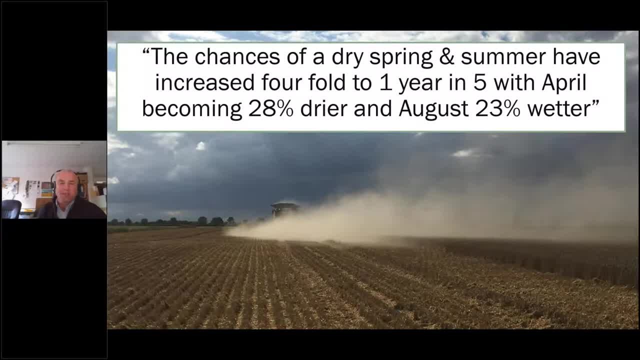 of what we've seen changing from a period of 1961 to 1990, and then the weather recordings from 2000 to 2015 onwards, And at the time, in January, after that wet autumn we'd sort of experienced- I was talking about- the chance of a dry spring, and 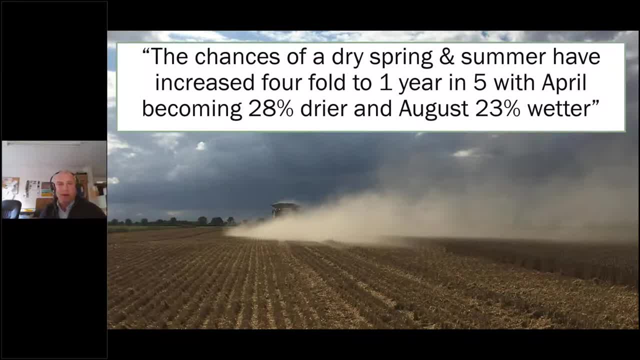 summer increasing fourfold from perhaps one year in 20 to one year in five. and also during that period of time we'd seen August getting sort of 23 percent wetter and April nearly 28 percent drier. so two really key months in the farming calendar. So in the spring you're looking to get crops. 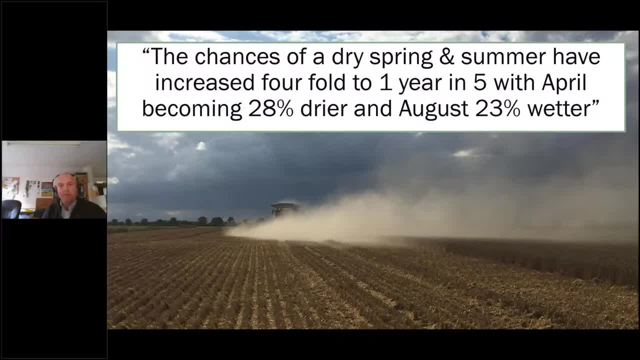 established well and growing well, trying to maximise growth time and then trying to get the crop in. I think it was quite ironic when I was standing in the meeting and people were looking quite quizzically when I was talking about the possibility of a dry April, when we're. 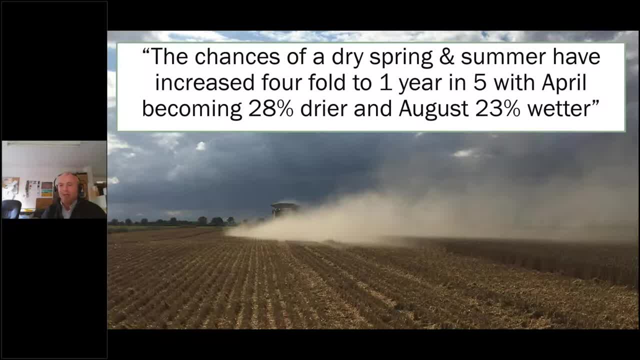 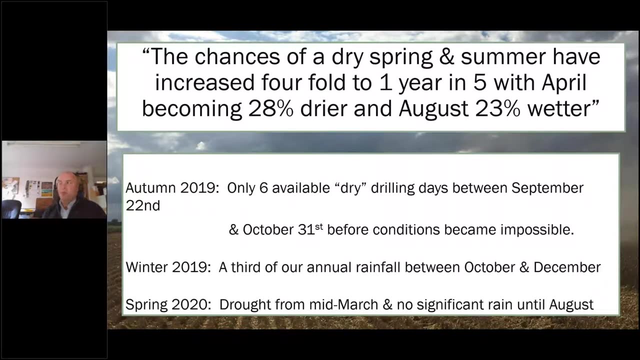 looking at waterlogged fields, lots of fields at field capacity, I'd say I was a bit of a prophet. I don't think I am. I had no idea how true those words would become, and so if we sort of reflect on sort of what happened during that season- I think back to last autumn- I would only describe 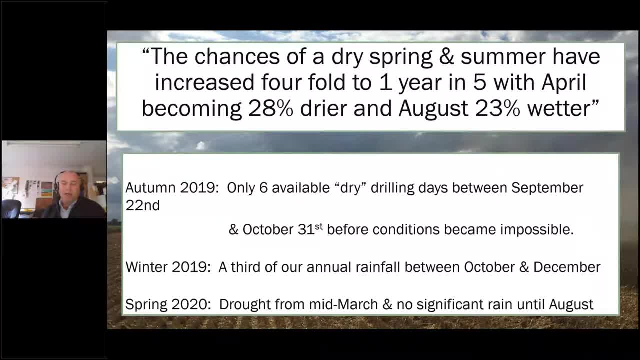 we probably had in our area available dry drilling windows for winter wheat and winter barley between sort of September the 22nd and October the 23rd, 31st, and when we're talking about available dry drilling days, that's was allowing the soil to. 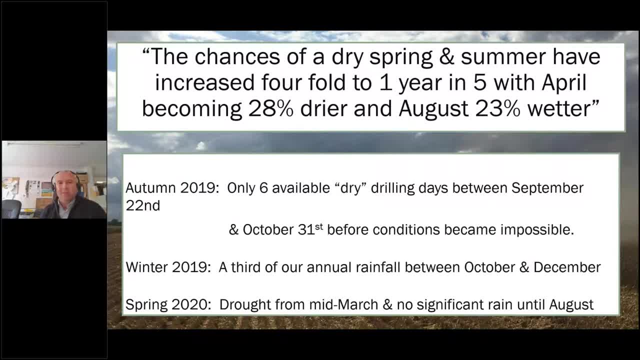 become dry enough to travel on in the first place and then by the time we got to the 31st of October, that would pretty much shut the doors at that point then and there was no windows really for us to try and get on. So really quite challenging and obviously that had a knock-on effect in 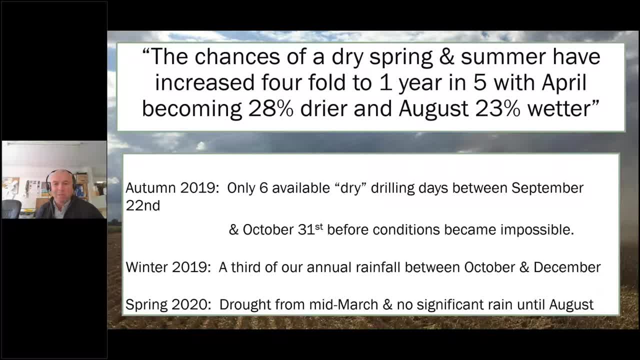 in terms of our cropping, we were probably 62 percent drilled on our winter wheat area and then obviously that the rest was made up with with more spring cropping than we'd like. but you can't help the season and, ironically, if you look at our rainfall records, if you look to the 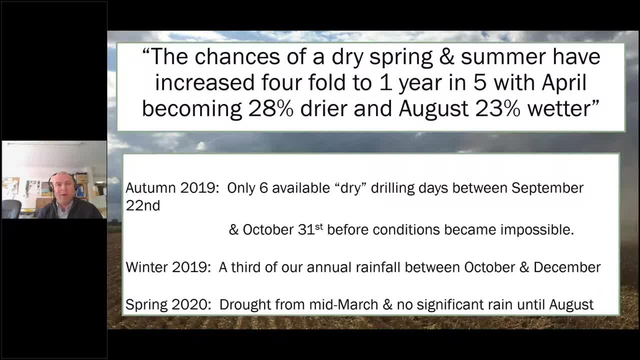 winter wheat area and you look at those in isolation, we probably averaged somewhere around about 160 millimetres last year. normally would be somewhere between 480 to 560. so the actual total rainfall didn't look too different, but the problem with it really was is that a third of that came. 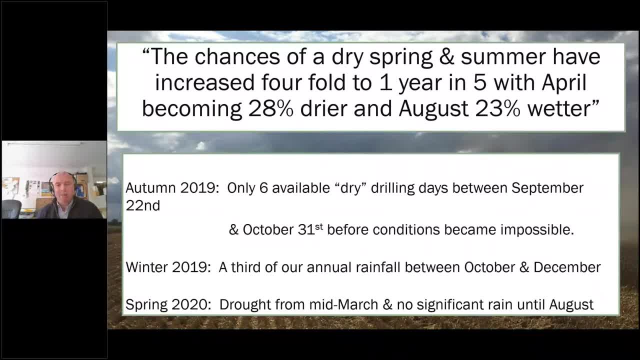 between October and December, so a lot of our very short period of time. and then the ironic bit about it was was the drought we had then from mid-March, so we were fairly wet through to February, got into middle of March. So real, proper, significant rainfall again until harvest. so pretty much mirroring what 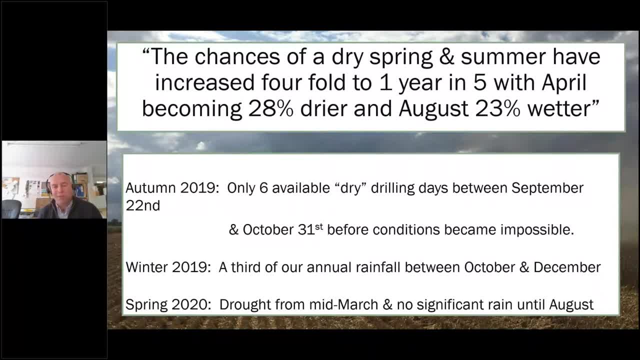 I'd expected to, or what I've been talking about during the winter. I didn't think it would come true, but I have heard it said that sometimes you can. you can get sort of two years of drought in a row, but it's been a difficult year this year for crop establishment and crop growth and on the 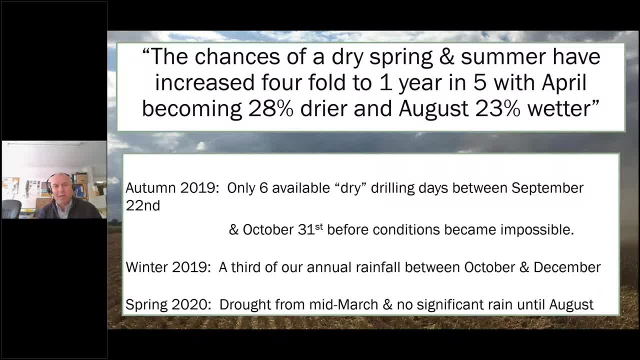 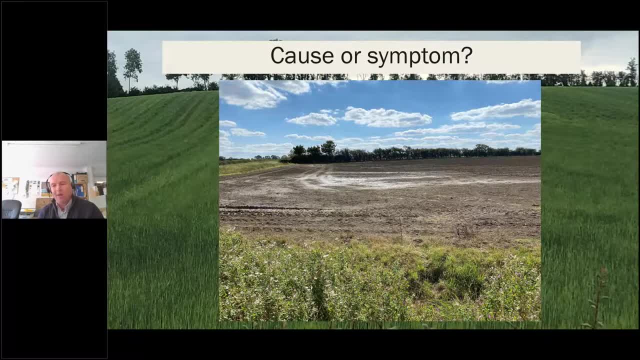 whole. it's challenging but hopefully there's been some interesting bits that have really come out of that during that period as well, and sometimes it really does come down to what's in your soil and certainly with with sort of no tillage, and I think it's really interesting Hannah's presentation where you can see that difference in soil going. 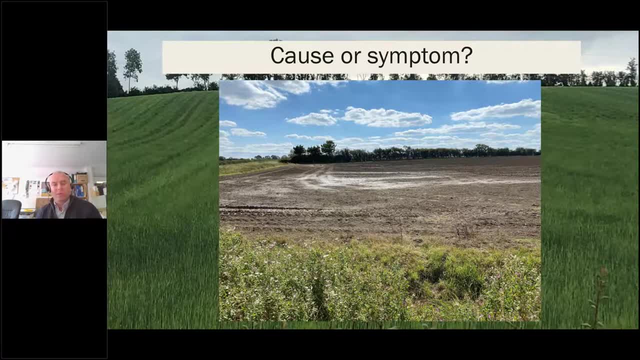 forward over that period of time is that you can do get your soils in a really good condition with a good bit of attention to detail. but it's understanding what the problems are with it and this is a great couple of pictures here which illustrates probably what you're talking. 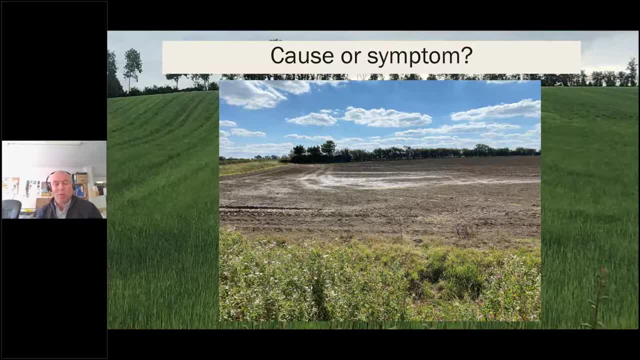 about in terms of how you react to. you know where the problems are in soil. so we've had a lot of like in which we see on the front screen here, water sitting on the surface. now this is really interesting. this one, this is- this isn't my field, but one next door to one of ours- and what? 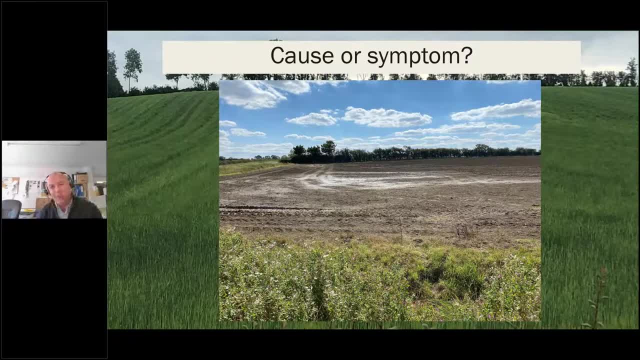 they've done is they've they've cultivated the soil. it's really really fine on the top. we have those heavy rainfall periods in August and the water sitting on the top- see where it's consolidated together, run together. probably too fine material at that point there which blocks those soil pores. 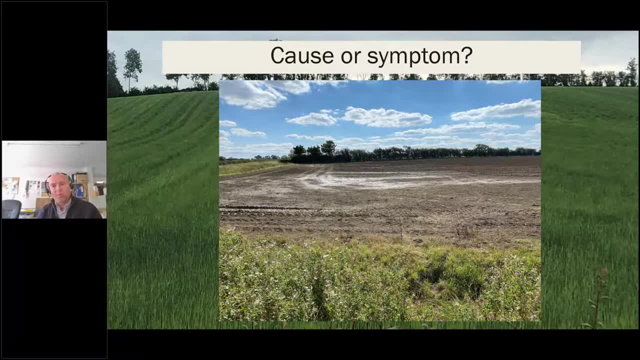 and I could find going around in a lot of positions that any problem areas weren't too deep. so once you dug through into the soil profile- anything below somewhere- depending on where they were- seven to ten centimeters- the structure was pretty good. so the problems have been in the in. 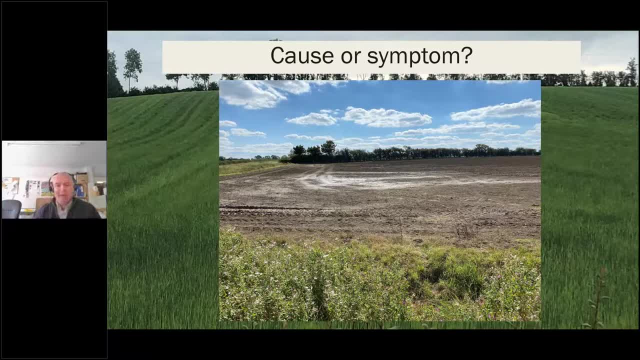 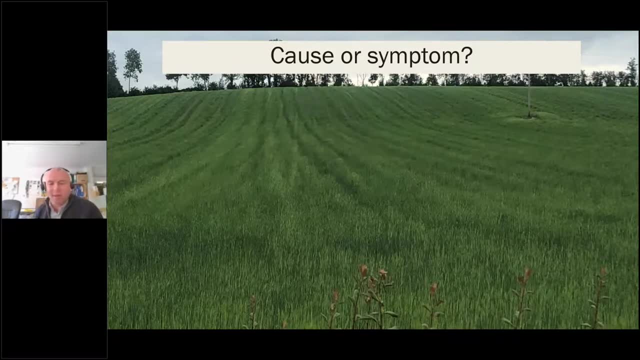 the soil surface and sometimes it can be man-made, and this next picture is a good example here. this is a spring barley field. now that the problem here you can see there's plenty of wheel marks. you know they're virtually attracted with going all the way across. you know spring barley is. 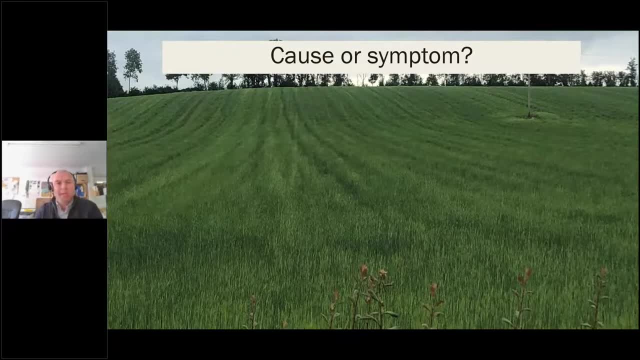 pretty sensitive to compaction, as are other crops, but it really shows that there's there's problems in that field. but the interesting thing for this reflection of last autumn, where you know the opportunity to cultivate and drill wasn't there on this particular field, this is a contract farm which we went on to and what they've done? they just start drilled in the spring. 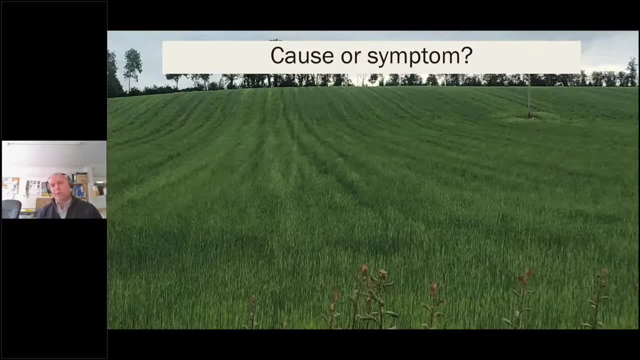 now with direct drilling. it's not a cure to if your soil isn't in the right condition in the first place, and sometimes you've got to build up to that level to allow yourself to. interesting thing with this one. the problem with this field goes back to two years beforehand, where there was 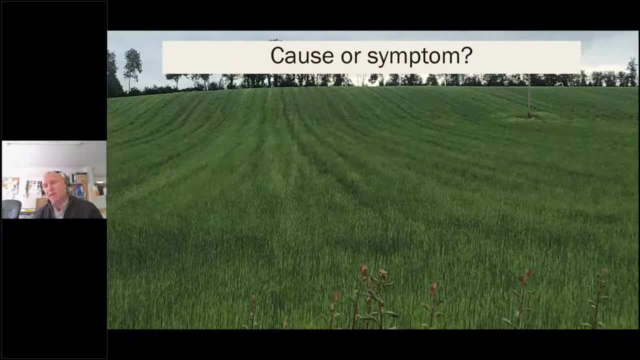 a wet period in the autumn, cultivating with a sort of a disc and packer type combination when the soil is at a really plasticky level and what it's done? it's got that shallow level of compact. so when the roots are hitting that point they can't get through. but it just goes to illustrate. sometimes 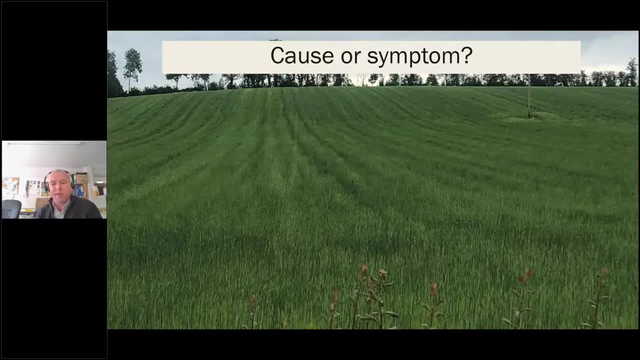 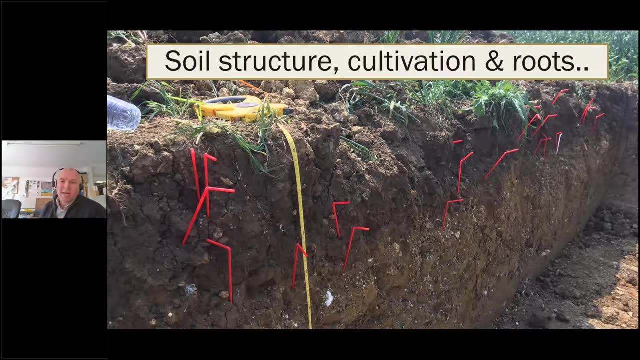 just no till on its own isn't a cure for soil problems and sometimes you have to maybe look at it and do a bit more remedial action in situations. this is a really great picture and this was a saw pit which we many of you probably heard me speak before. i've shown this a number of times. 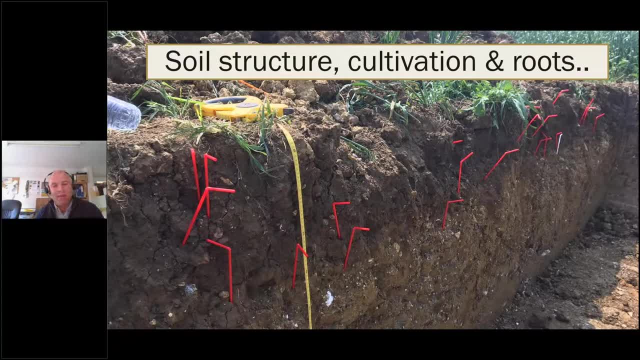 i think it's a great picture. rob simmons from crownfield came out and we had a look at our soils. back in 2017 we were part of the monitor farm program. you can see here classic heavy clay on that bit underneath, on. that's a layer there and then we've 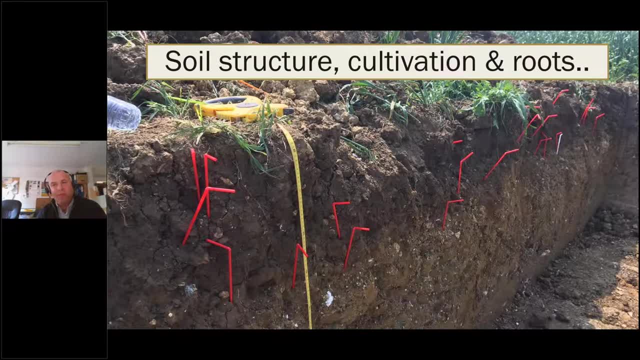 got that nice structure on the top surface, the really the the red straws are the deep burrowing wormholes, and so what we're looking to try and do is we want to try and maintain that structure. um, we see that worm numbers increase again, something that hannah's highlighted. um, and you 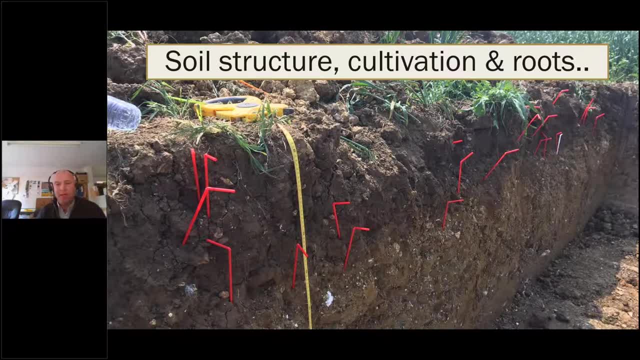 do see those numbers that build up quite nicely so the further you go through the process. but you know there is a case for sometimes do you need to cultivate, sometimes as a case of remedial action we've had to sometimes. you know a couple of situations this year after, after that last. 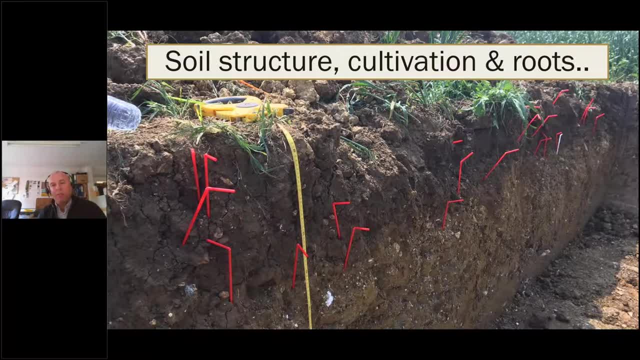 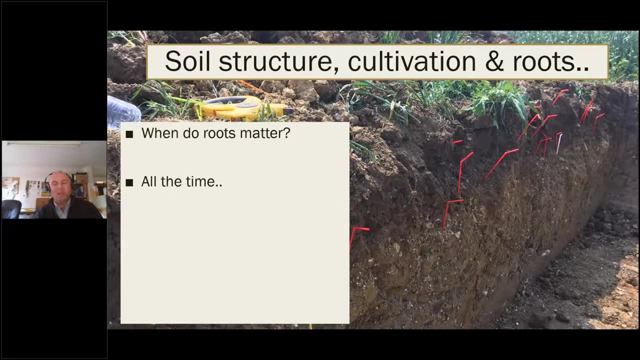 autumn, have had to maybe cultivate, you know, not terribly deep, but just alleviate where you've had a bit of a problem. so i guess the question is, you know, when do roots really matter in a rotation? well, all the time. if you're in an otil situation, they natural water pumps, you know, in these wetter. 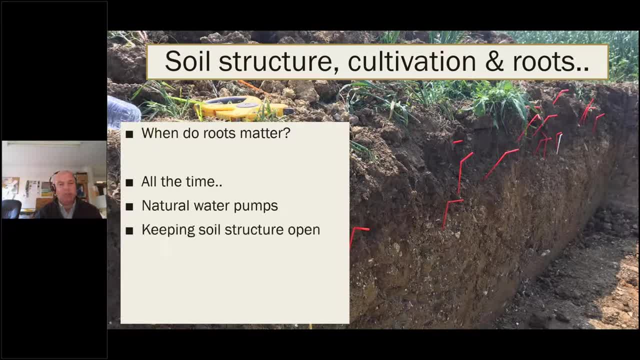 conditions. they're moving water all the time. they're keeping that soil structure in place, keep it nice, and keeping those worm channel opens helps maintain biology. there's an awful lot going on with reduced soil structure, and so i think that's a really good question, um, and i think that's. 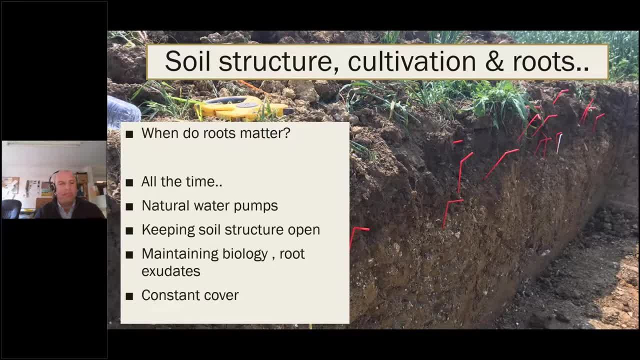 root exudates, and having that interaction with within roots within a system and trying to have a form of constant cover isn't a bad thing. I mean, there's often a term that's that you don't want to sort of naked, but I think it's sort of quite appropriate where you're trying to keep soils. 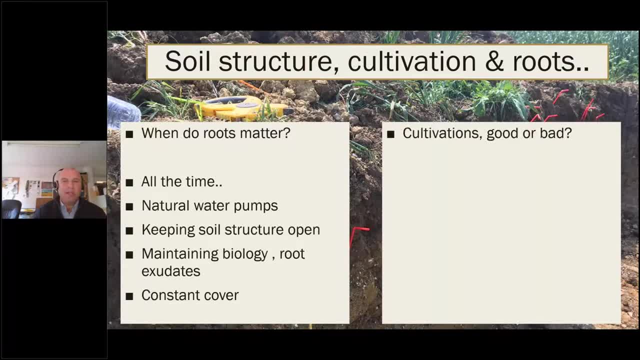 in good order as well, but other situations that you need to cultivate. I think it's being dramatic about what you've got. you know there are extreme situations. some of this sometimes can be man-made compaction, like we spoke about in that previous picture where you put in a cold space. 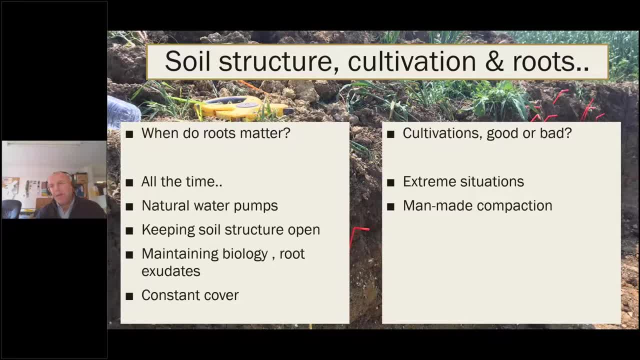 layer in the wrong conditions. sometimes it may be forced upon you if you're in a difficult situation, if you've got root crops, for example. but cultivations do not create soil structure on their own. they can change aggregation, but they don't sort of really influence soil structure. 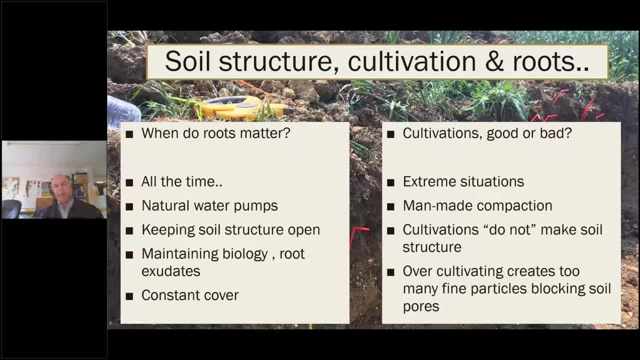 and again coming back to that picture we looked at over cultivating creates too many of these sort of fine particles which block the soil pores and sometimes, if you've got it to find that surface, you can see where they've blocked the soil pores. you'll almost have that, what I describe as. 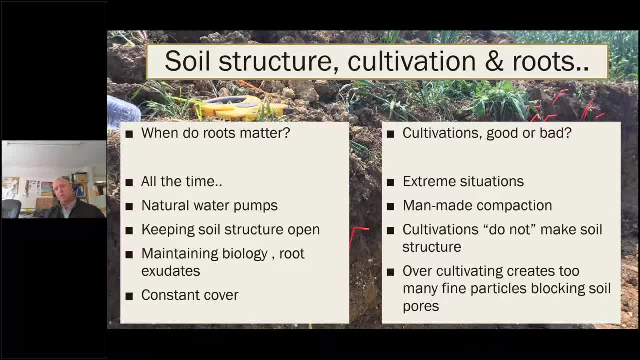 that sort of sort of sponge layer where it'll be really really wet in that top sort of surface where you've cultivated to and dry underneath. so it's really understanding sometimes, sort of where the problem is. I thought this would be a good time to have a look at a poll, not a poll like that just out of. 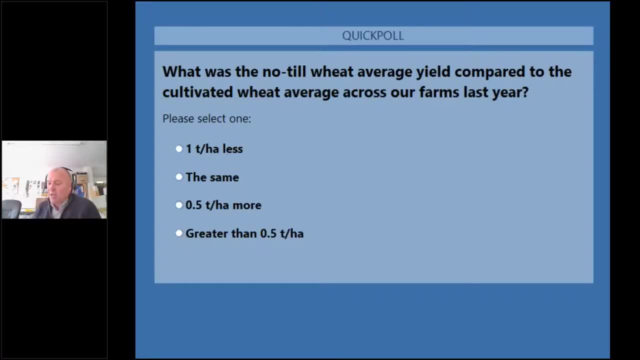 interest and you know you'll get the answer sort of later on. just have a look how you think crops may have performed last year. did our no-till crops, for example? were they one ton a hectare less than our cultivated crops? were they about the same? 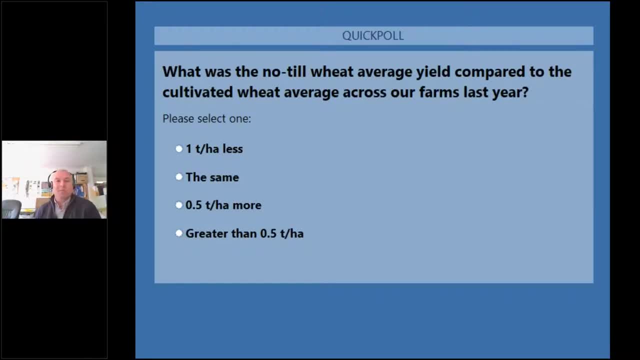 well, they're half a ton a hectare more, or was the response, you know, grace? and half a ton a hectare more. you know we may have had some cost savings there, but we didn't always have the yields. you know there is a balance between two, but it'd be quite interesting to see, you know what do you think? 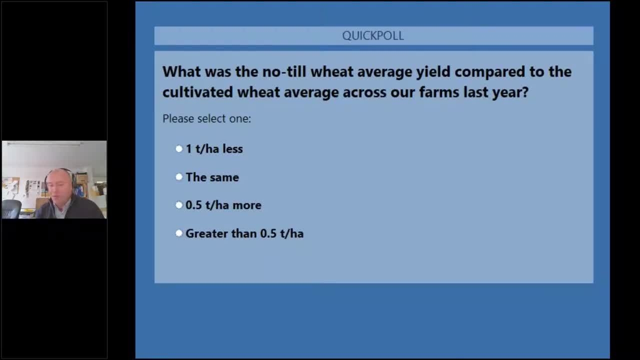 maybe the difference, and you know how it may have panned out. so I'll leave that poll to run. we'll see what the answers come out like. and so, just reflecting on last autumn, if I look at where we were- so bear in mind the amount of rainfall we're talking about- we had a lot of, you know, sort of 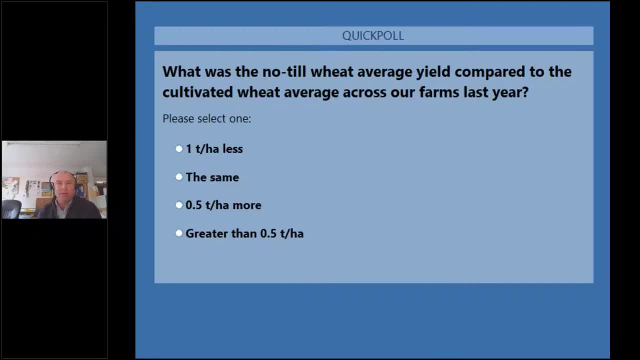 pretty wet soils at one point, very limited drilling window. this is a good example of of what we really learned about what we're doing. so we established a catch crop here after an all seed rape crop, so we've got a very good root systems going on. we've got the all seed rape um volunteer. 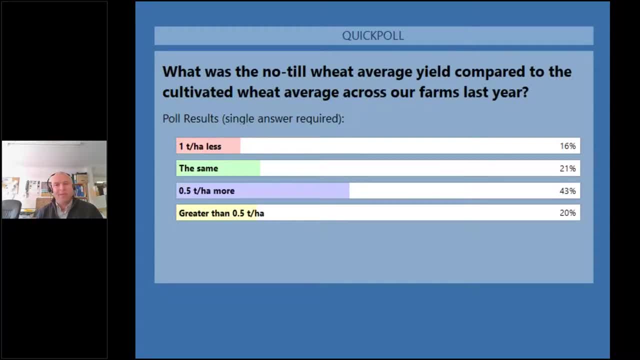 result: um, all seed rape volunteers, we've got, uh, phacelia in there, we've got some oats, we've got some mustard as well, and the idea being with that is that we like to try and drill a little bit later for black grass control, and especially with no tiller. i found that you need to have good. 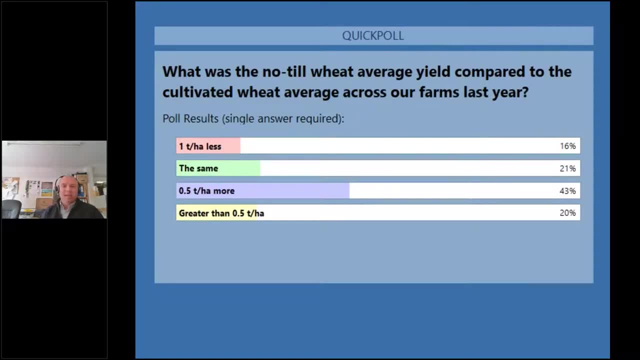 conditions to to drill into. and this really helps with those laced drilling, especially if it, if it turns, turns wet, that it keeps the moisture pumping out, keeps the soil structure nice and open and gives you machinery such travel on. so this was our last day of drilling. uh, last autumn, on the 31st. 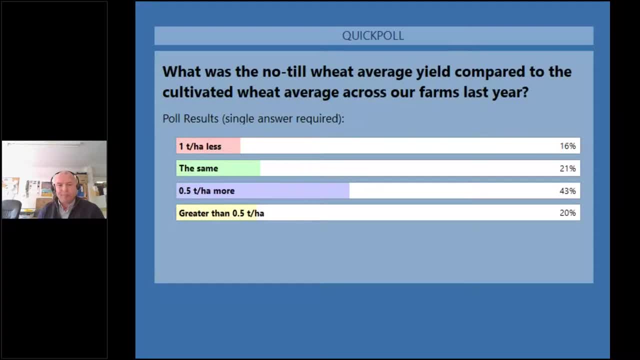 of october- um, you know drilling into this sort of cover, and i was amazed how well it really went. my father-in-law thought i was nuts doing what we're doing, but this is into, so it's really wet. you can see they've got some nice structure. 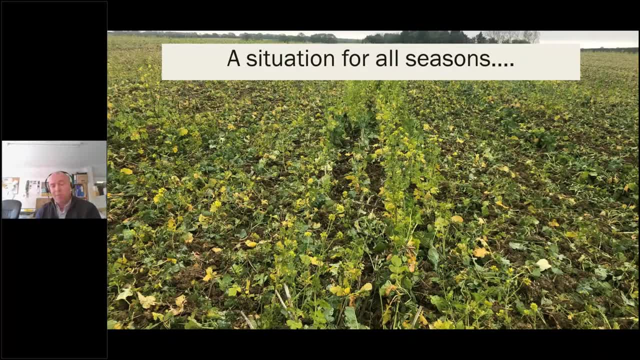 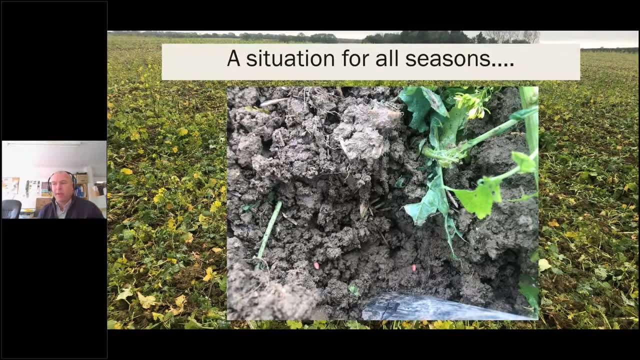 and this is a field that's in year four of no till and i thought we were really pushing the boundaries, especially with the weather conditions afterwards, of how it was going to go, and it's going to be a real test of whether we were doing the right thing and how things were going to pan. 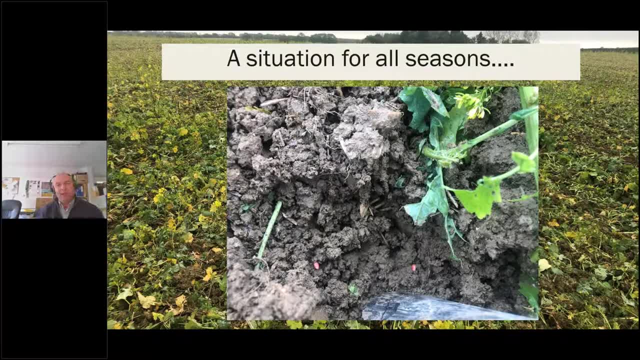 out. so if we look at how it went through the season, um, and as a grow, there's nothing more satisfying than seeing a new crop emerging, and this is that crop then emerging towards, uh, the back end of november, early december, you can see the, the residue from the previous catch. 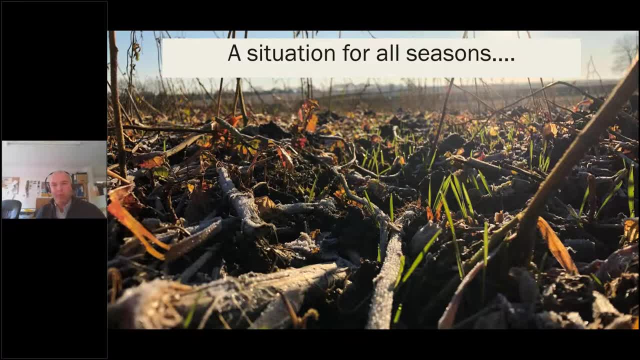 crop and the volunteer will see rape dying away in the background and we've got the wheat popping through and this is what it looked just going into january, so that the rows are up- you can see the residue is still in there- and by june- um, this is the crop we had and this is. 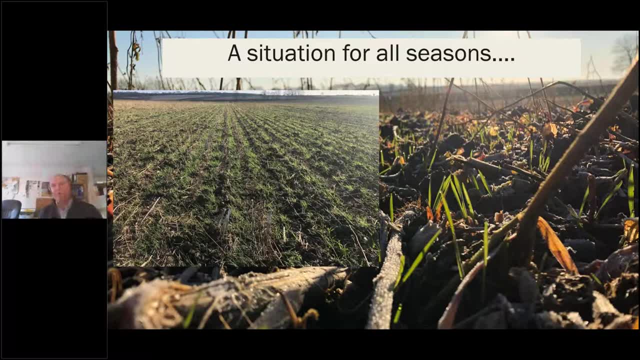 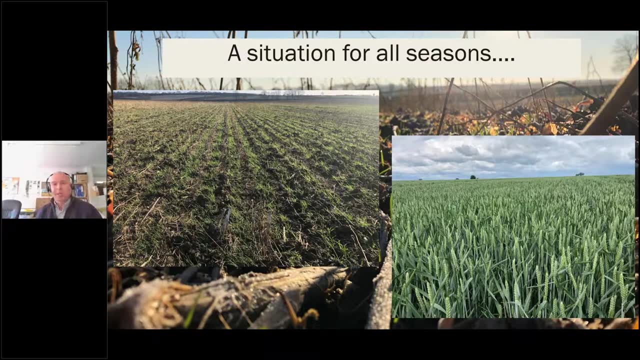 probably, i think, one of the the most reassuring things we've had about what we're trying to do was the right thing and the ability to to get on in a difficult season and get and get crops established. but that particular field went on to yield so just about 9.3 per hectare- our wheat. 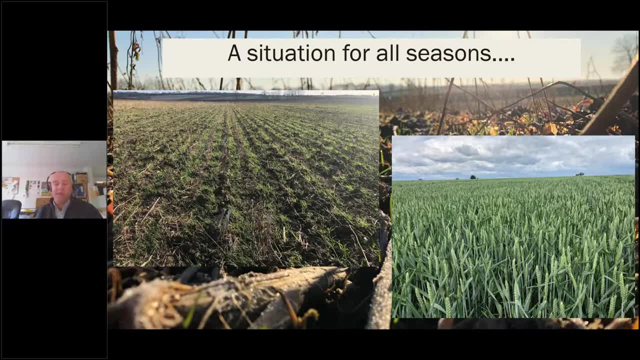 performance on whole was was down probably about 25 percent, uh this year and on a reflection this season. but we did see in those those situations that where we were actually doing less invasive techniques that actually were able to get on better and the crops coped pretty well at the 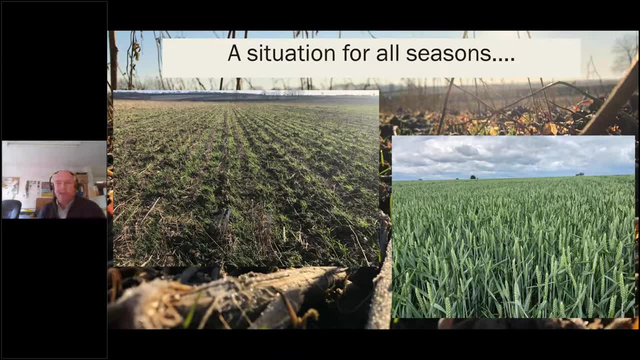 same time again. this is another interesting one. so this was a direct drill wheat crop after spring oats. i put a brief catch crop in here as well, so we've got oat volunteers. we'd also got um a catch up with a mixture of buckwheat and some clover in it as well. 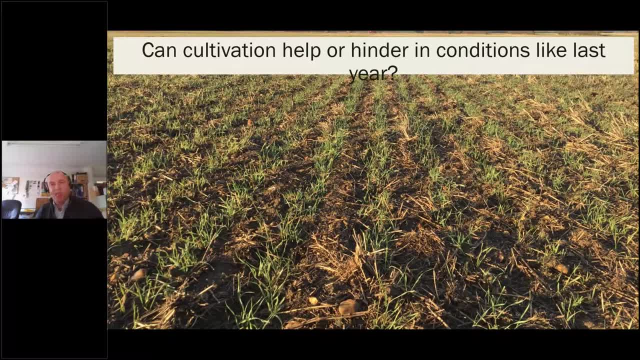 and drilled into it and established pretty well. and i guess the question is: did it make it? would the difference if we cultivated well? this is the result on a field on that same block. so we had three fields within there on a 30 hectare block, this particular field with mold drain, so we had 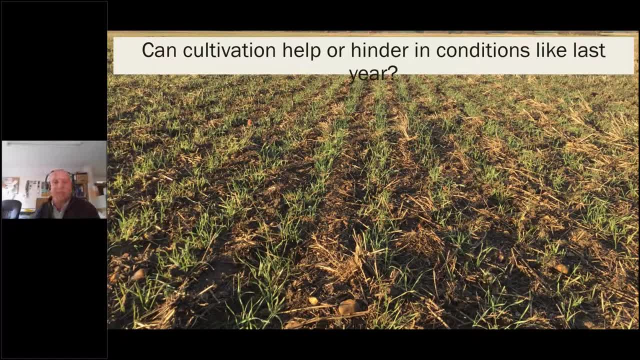 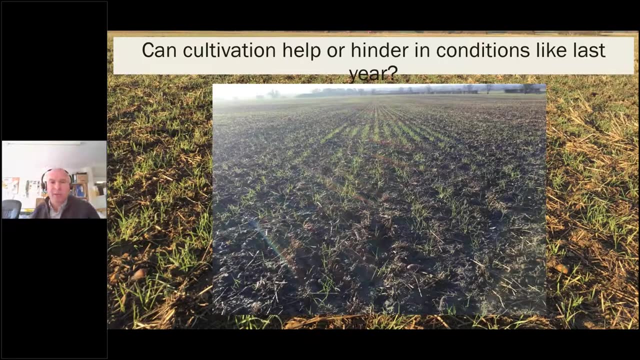 to cultivate afterwards. to level out again: um, not over cultivated, not particularly fine, but for all intents and purposes our establishment was really, really compromised in this area, with water just being probably held up in upper surface layer a bit more compared to where we're direct drilling. you can see the patchy nature of of that crop. and then the difference between the two fields was. 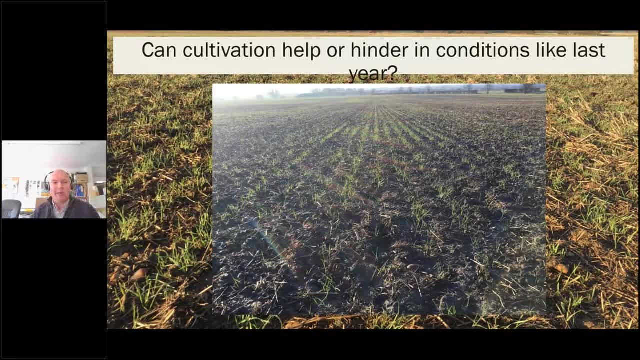 about 0.75 tons per hectare. um now, if i hadn't known we've mold drained it, i said we probably you know we've got a wet layer but mold draining there. we put the the channel into trying to get water away. but cultivations in that particular situation for us there hadn't really helped. so 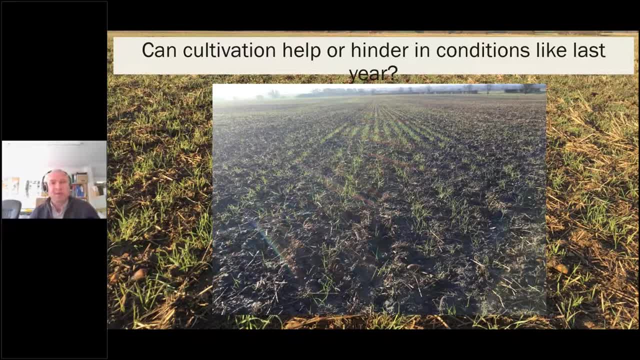 quite, you know, quite challenging, and you can see the difference between the two different farms, different situations. but what we were seeing last year, that we were getting a positive result and almost less, meant a bit more really, when you sort of roll those uh results forward. and coming back to what we've seen on the poll, 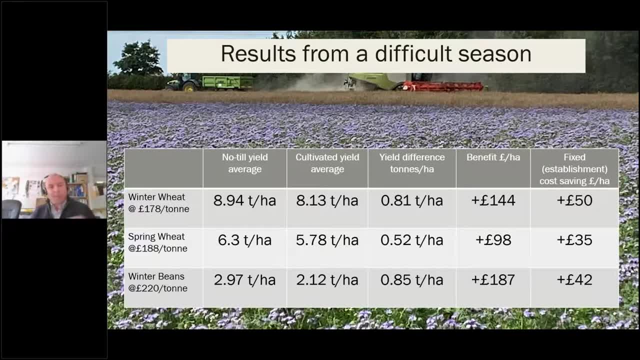 um, this is looking at our results from last year on the last column we've got, when we've got winter wheat, spring wheat and winter beans and that's the selling price with them as well, i know. so all wheat yield averages were just under nine tons per hectare. 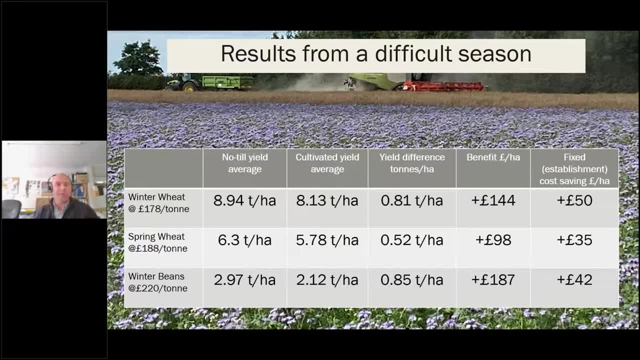 so, although we're down performance wise, we had a good result compared to our cultivation areas, by sort of about 0.81 tons per hectare, and when you multiply that up in terms that yield difference as of 144 pounds per hectare, um, and then the other bonus is, so we've got our saving in establishment. 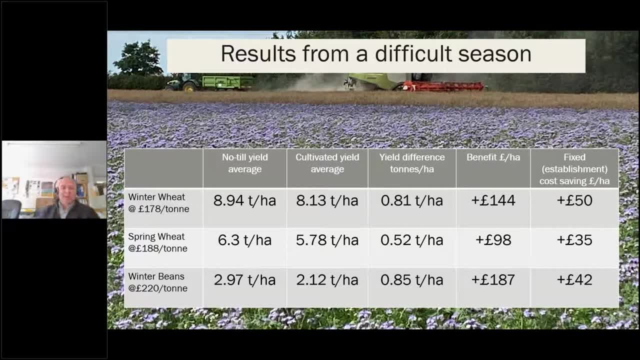 costs and operational costs on there as well, so you can see some, some real benefits. so coming from that point there- and i always felt, certainly when it comes to snow till- is that the focus shouldn't be purely on um cost saving from machinery etc. that's the bonus that really comes from you know. 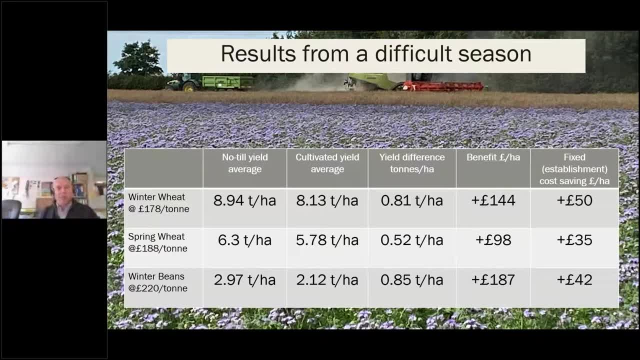 going down the road of trying to disturb less and improve your soils as well and merely gaining spring wheat. obviously the the advantage wasn't quite so big, but again we saw a yield increase on spring water and quite a big jump on winter beans, and the winter beans was really interesting. so 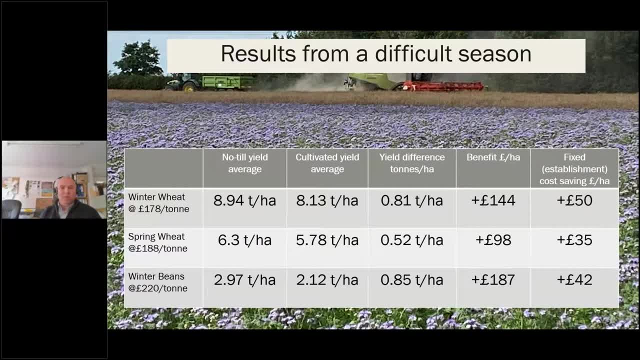 we'd run a, a sub sort of, through those fields in the autumn and then direct drilled into the spring, whereas the direct drilled area- with direct drilled only, and had a more positive yield result. so you get another season. um, you might not see those differences and i'm probably expecting it in a 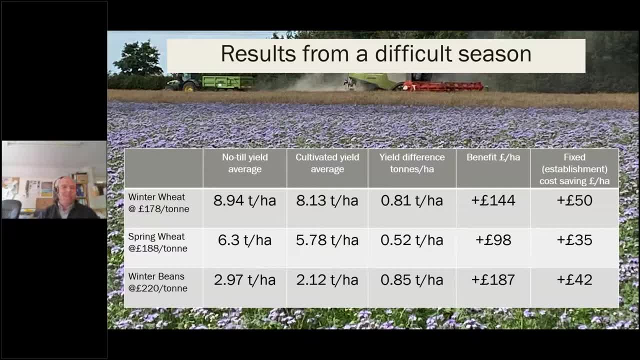 more normal autumn, where conditions are more kind to both systems, that those differences probably would be would be less than are not too different. but i think the key bit here really is that there's often a lot of talk about yield penalties with no till, and i guess that's a balance really in terms of if you're 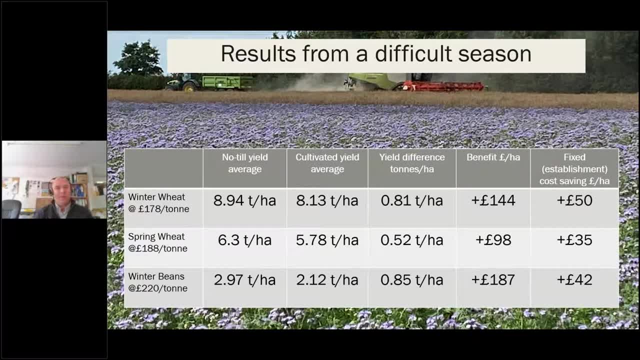 sacrificing a lot of yield. you probably have to question whether it's the right thing, but certainly from our experiences that it was either on a par um or better um, and if they are slightly below it's not by an awful lot. so some really good sort of positives to to take out of that one um and i had. 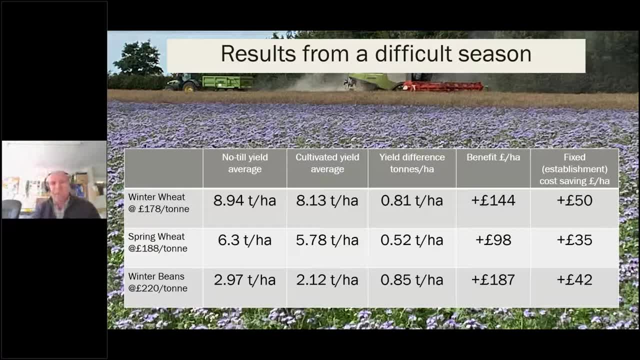 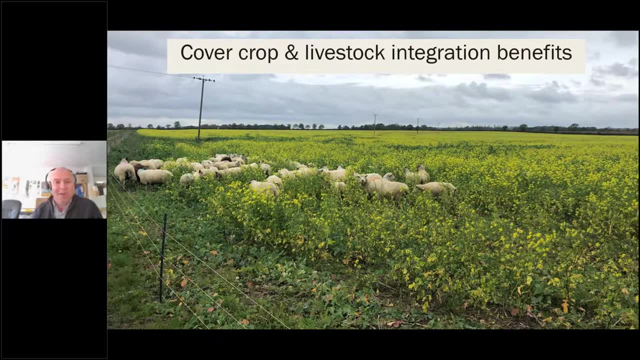 cover crops and livestock for a number of years now and we've got sheep going in here. this is a mixture, got some mustard in it. um, some of this suggests to me that i was trying to have mustard infused lamb going forward. i think theory. i don't think it probably. 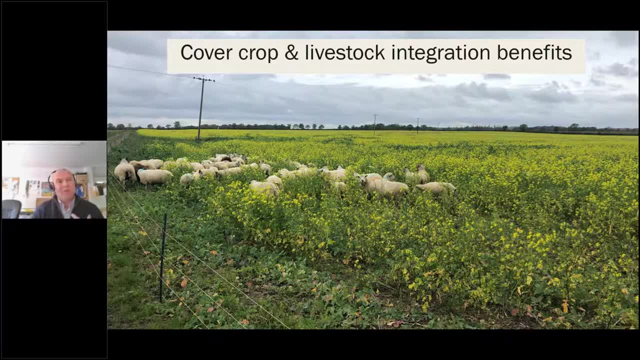 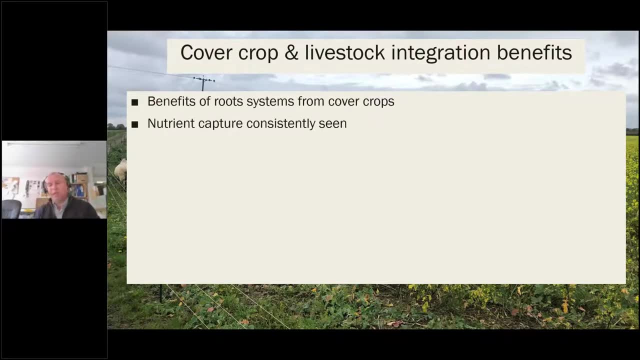 works out in reality. we've done this before as well. we've looked at cover crops, which we know they work pretty well. we know the benefits of the roots in the system. we know we're capturing nutrients. we're seeing circa 35 to 40 kilograms of nitrogen captured quite consistently. we're 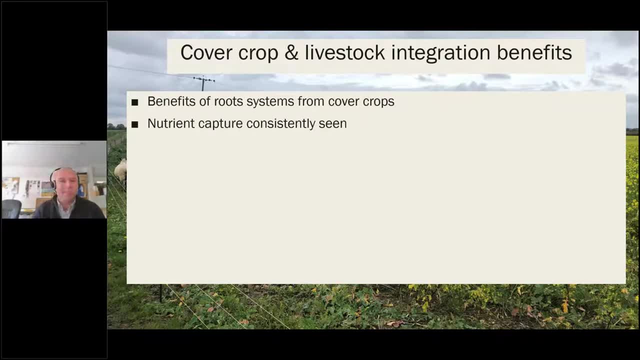 tending to discover that's coming back in, sometimes two to three years later in the system. um, the question: is there an advantage to grazing covers or terminating in, uh, mechanically? um, i think it inflows, sometimes difficult to really see a result from it, but this year we did see some. 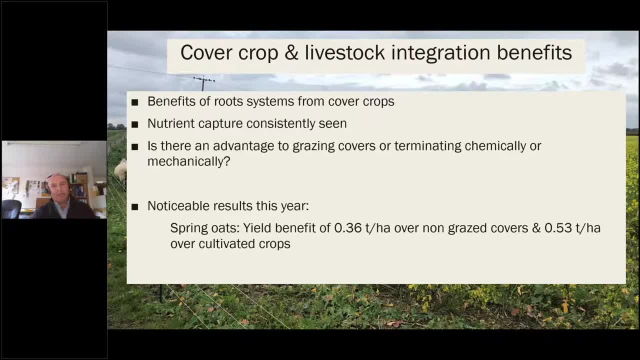 noticeable results on those ones. um, certainly in our spring oats we saw a yield benefit of 0.3 tonne of hectare over our non-grace covered uh cover crops, where we just spray them off. um, and then a greater one where we hadn't uh, where we just cultivated. and again in spring balding we saw 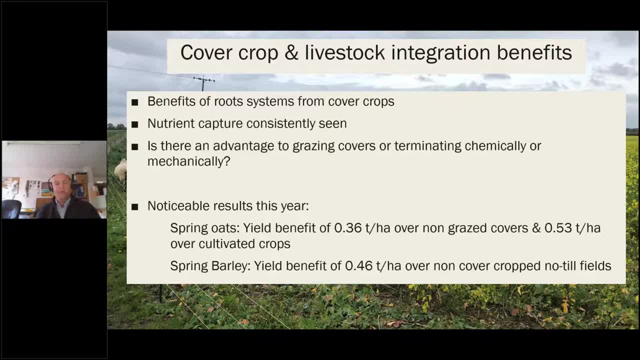 a yield benefit of 0.3 tonne of hectare over our just purely um non-cover crop field. so i don't always see this result. we've seen this result this year, so it can vary year to year, but it's nice to see some some positive results in uh in in those terms as well. so really just to bring it all. 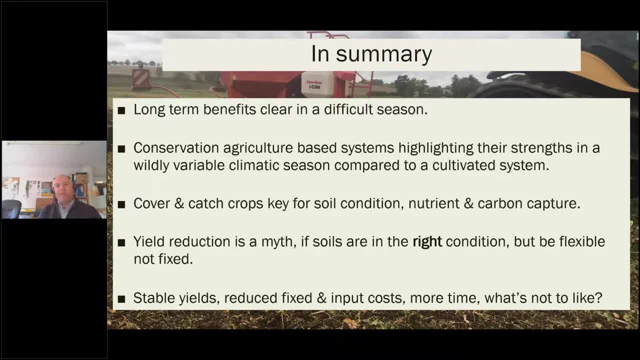 together and a bit of a summary, i think it's. it's good in a really difficult season that no soil can really help, um, certainly with catch crops, if you get those right. i think it's important not to get them too thick but help shoot it into difficult conditions almost quite a lot, while 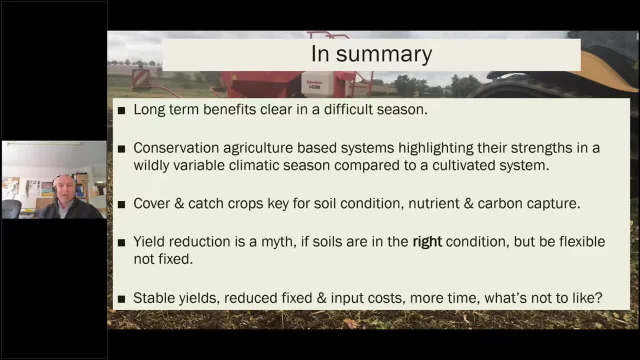 we're seeing now, and i think if you take the road down the conservation ag based system, they really highlight their strengths in these wildly variable seasons. we seem to be guessing now they'll hold on that a little bit more in, in sort of drier conditions. um, but you know, sometimes you may. 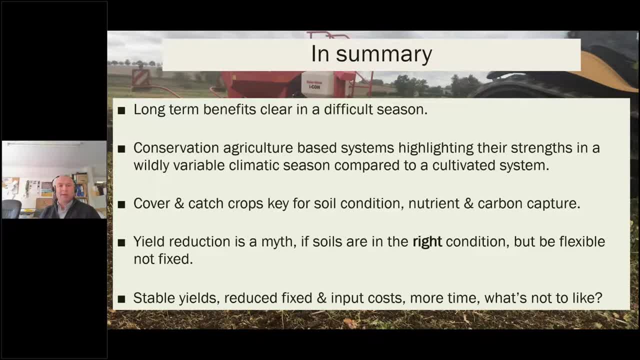 need to cultivate in situations if you need to correct something. uh, i've no doubt that covering catch crops are really helpful for soil condition, nutrients and carbon capture. um hannah's highlighted brilliantly that what happens within those soils- and we've seen their results as well- that you know there's a lot you can do with the. 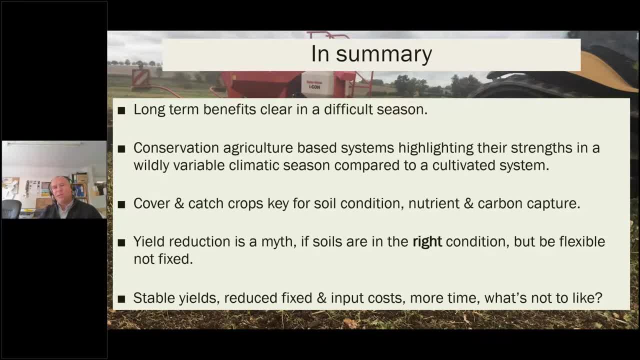 system. uh, and certainly from what i've seen and we've highlighted that, you know that yield reduction is a bit of a myth. if your soils are in the right condition, i think it is important to explore in your approach and not be too fixed on just doing doing one thing and sometimes 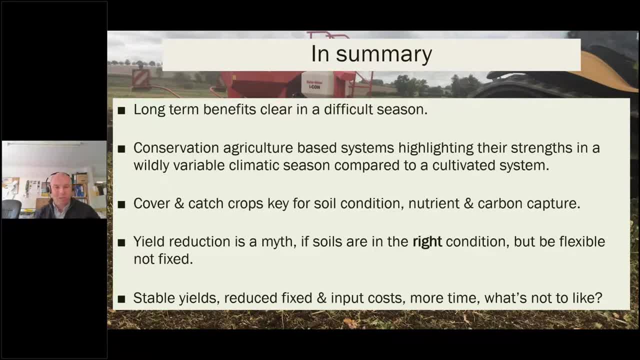 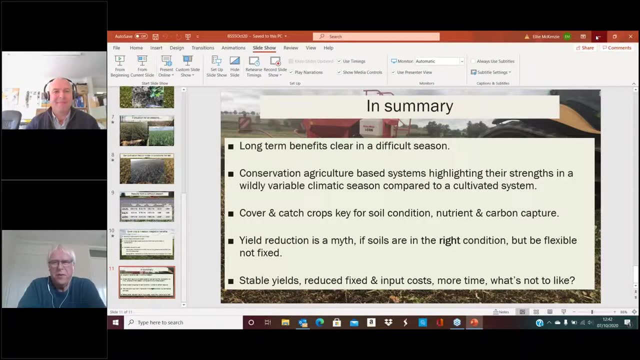 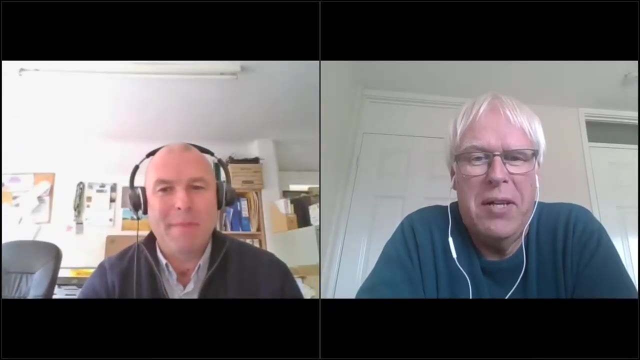 reacting to these and um, but overall really, uh, stable yields, fixed and input cost reduction, more time to spend what's not to and, uh, thank you very much for for listening. thank you, thank you very much, russell, for a very interesting presentation and for giving us a no-till look from a practical perspective and a positive outlook that you can still make it work. 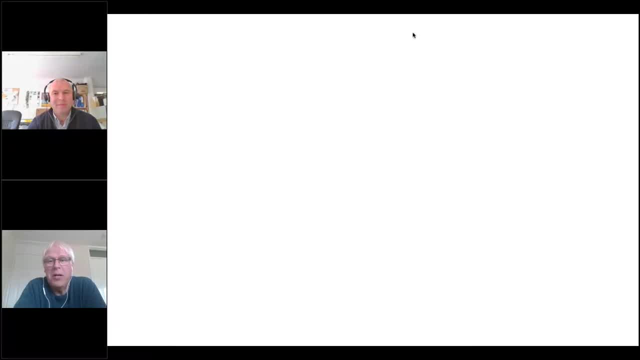 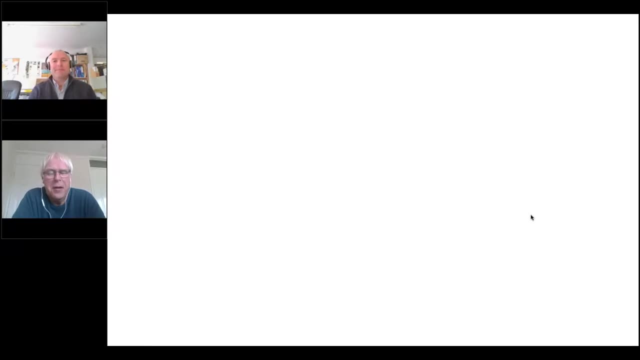 on a very wide range of what will be challenging conditions. so, as i indicated, we will be taking questions now to both russell and um um and and um and um, Hannah, sorry. so for that I'll be handing over to my colleague, Dan, who's been monitoring the 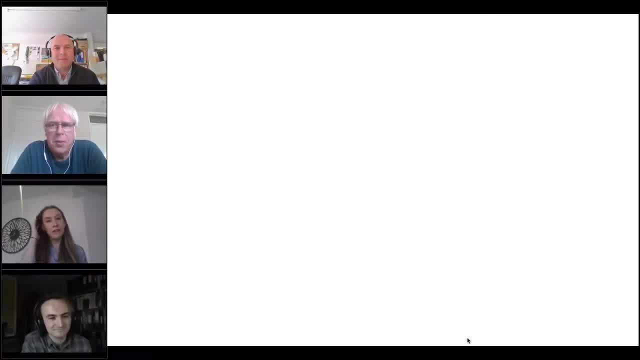 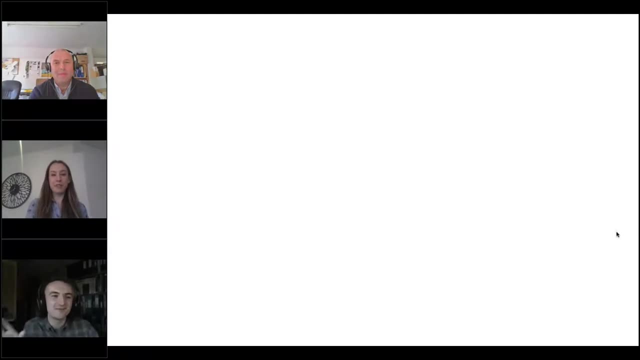 questions, but please, meanwhile, keep your questions coming, type them in. you'll keep on monitoring them. so I would say, Dan, over to you, thank you. thank you, Wilfred, and thank you to Russell and Hannah for stimulating presentations. so I've got a couple of questions for you, both kind of each relating to your particular 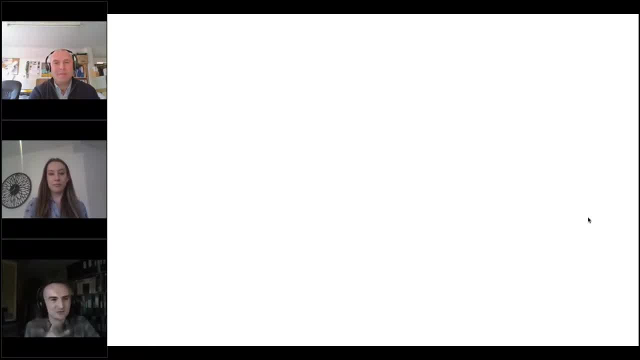 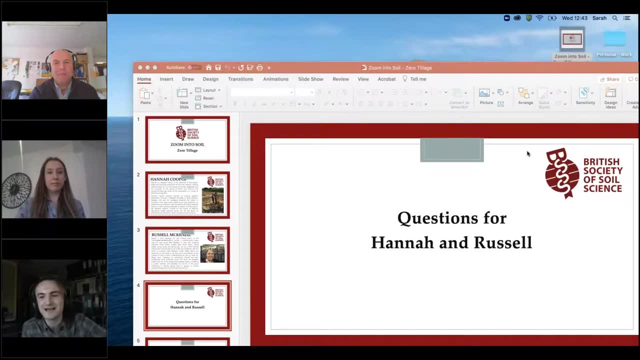 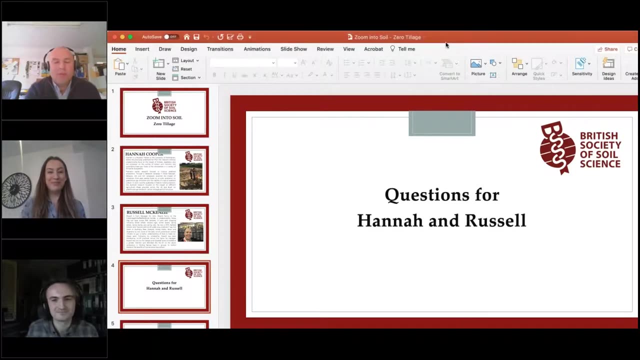 presentations and there may be more of a broad discussion. so just heard from Russell. Russell, in your yield analysis is there any bias that your no-till land may be on better soil? oh, that's a good question. that one, no, there isn't. I mean what? I look at all of our blocks. 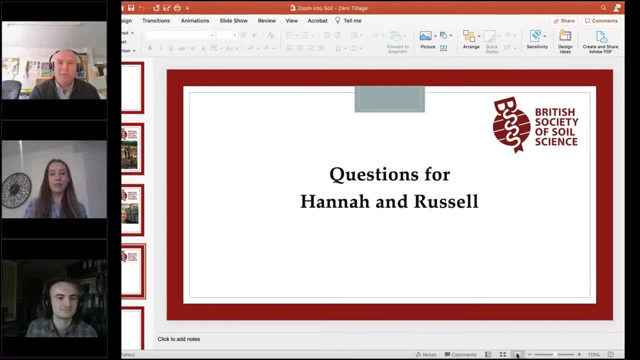 are the same. yeah, we probably have some blocks that may be performed best than others, but when I look at our analysis, that's everything combined, so it's looking. we've got four different blocks. I've been looking where we've got no-till on different blocks. you know, some may perform. 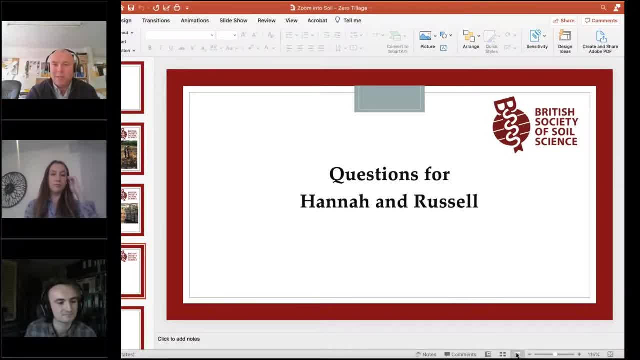 slightly better than others, but that mix is pretty spread and pretty consistent across all of them. so we've got a mixture across all the farms. so what you'll get when I talk about it is a pretty honest opinion in terms of what we see, which I think is really important. you know, we can all show. 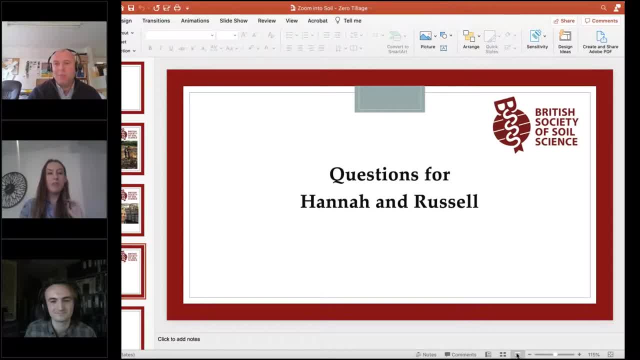 the good results, but I think it's pretty good important to be open and honest about what you're actually doing. yeah, absolutely, of course. and just one more, finally, on Russell, for your particular presentation. we have a question here about mole drains. if you didn't have mole drains, would you not be? 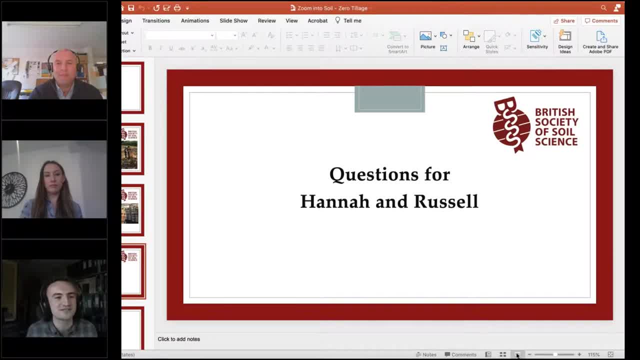 able to get onto the land, and do you think you need them with no-till systems? well, mole drainage is basically. the idea of the operation is: you've got land drainage underneath and what the moles are doing is they're creating a channel for the water to get through down to the drain. so those moles will, even in a good season, will only last probably sort of four to five years at most, and I think, for sometimes it's, you'll get some wet spots appear- and we certainly had some last year- and sometimes, just reacting to what you've, 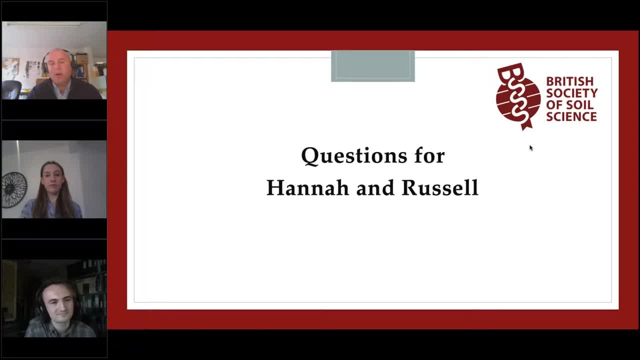 got. so I think, fundamentally, I think it's still quite a key operation, especially if you're on heavy ground and maintain those drains, drainage systems. it is really important. well, fantastic, thank you, Russell. so we've got a couple of questions now, then reflect on Hannah's presentation earlier in the webinar, so we've got one here about the texture, and there's quite a few. 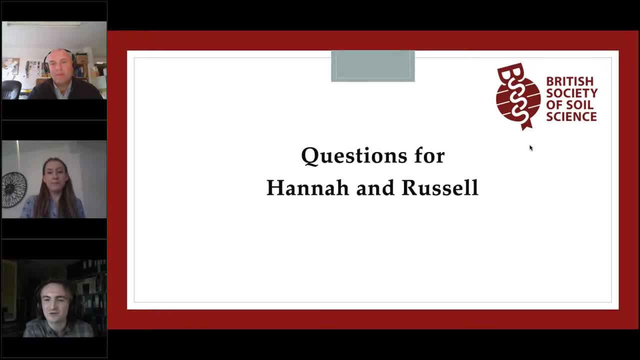 questions about the texture in the panel here. did you see any differences in your results, Hannah, in relation to the soil type, with clay versus sandy soils, particularly in regards to the greenhouse warming potential? yes, so majority of the samples were like heavy clay or clay loam, so that made 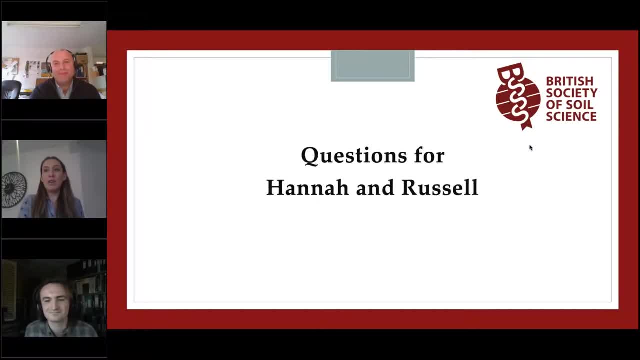 sampling really fun, um, but I did have a look at the differences between the textures. there weren't too many which were predominantly sandy, but it did seem in the sandy soils. so throughout the webinar I talked about the time aspect and the regeneration seemed to happen a bit quicker in the sandy soils. 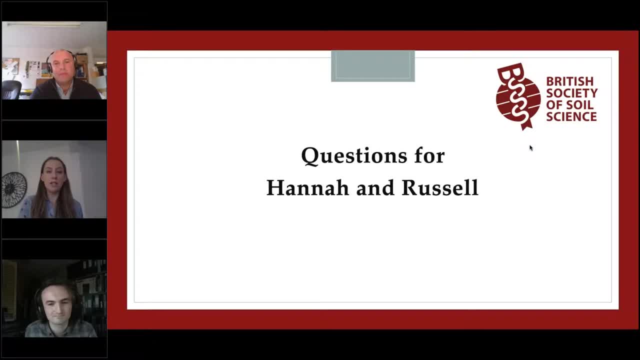 I suppose because you've got those macropores and things naturally developed, it didn't take quite so long for the structure to regenerate. um, I couldn't pull out any significant differences in the global warming potential between the two textures, um, but it did look like sandy soil um. 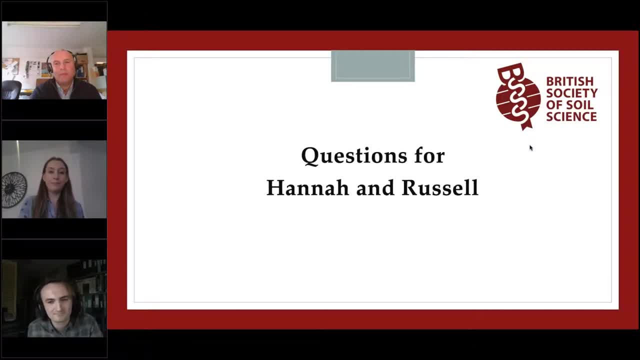 produced more co2, but it wasn't significant, fantastic. so, um, we can now kind of open out, uh, maybe the discussion to uh, to both of you and thinking across your different sites and and your work, uh, so we've got one here about climate and obviously very important, with climate change, how do you think climate will impact? how easy is? 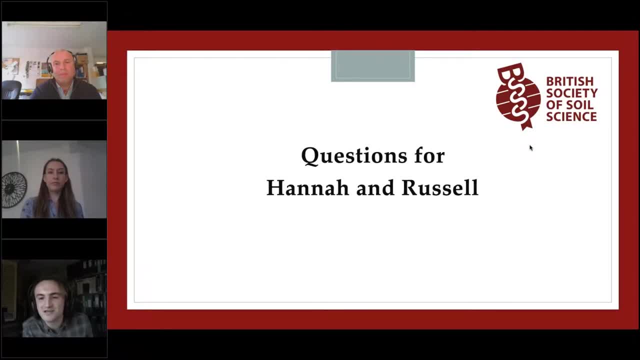 the transfer from conventional to zero tillage when we have such extreme weathers such as that in in 2020? um, I don't mind going first, um, so I think it's going to make it a lot harder in terms of farmers just starting out if they want to experiment converting. 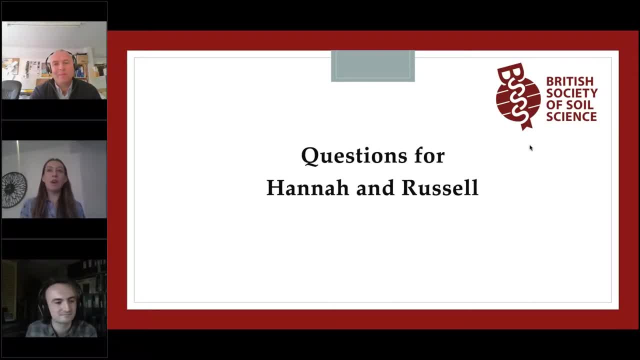 especially because of the erratic behavior of the weather. and what I found as well was in the first few years you do get that surface consolidation, so in terms of water logging, that's going to cause huge problems for the farmers. so, thinking future and climate change, it might also. 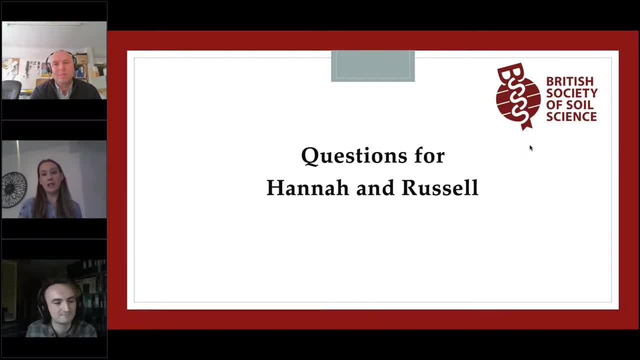 be an option here now for policy to change as well for zero tillage. so in those first few years where farmers are converting, provide subsidies and things to support them and help them in terms of um, it might be a bad season because of the erratic weather, but keep bearing with it and 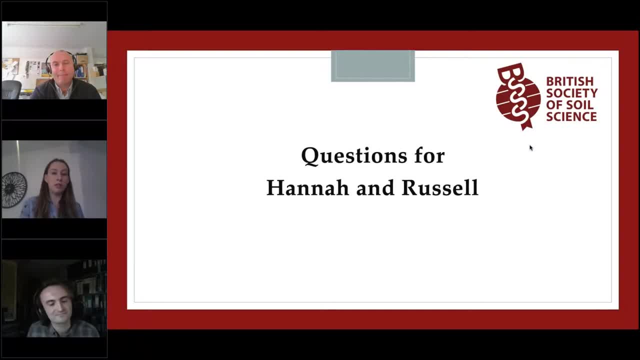 the stuff that I've shown. after about five, six years, the soil structure does regenerate and sugar and heat and and other things that need to be processed and in a way that doesn't offer a lot of energy. and- and that's really the biggest challenge for choice- it's not. 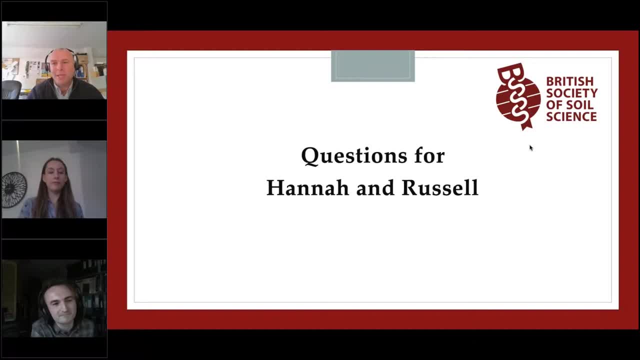 about. you know what you need to do, but I'm not sure that on average it's the same thing. Russell, have you got any added thoughts there? yeah, I mean I think it is a challenge. I mean it's it's you know, sometimes it can be a bit of a leap of faith and, and sometimes sort of when. 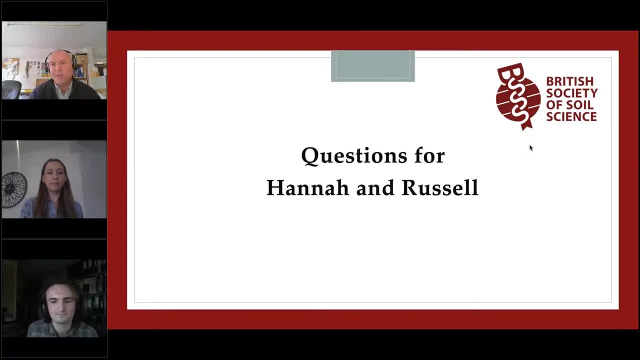 you're thinking about sort of changing it's. you know, trying of trying a bit first and gaining system. it can take a little bit longer for it to settle down, but if you've been bringing your observation depth shallower and shallower, then that that sort of transition can sort of happen. 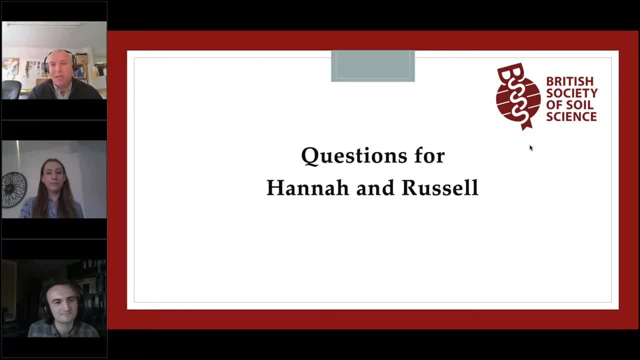 a bit quicker. so, um, you know, i don't think you probably get much more of a challenging season than we've probably just had. um, so i think there's- there was an awful lot to be learned from from this season. um, yeah, i wouldn't profess we got everything right by any means, but, um, i think. 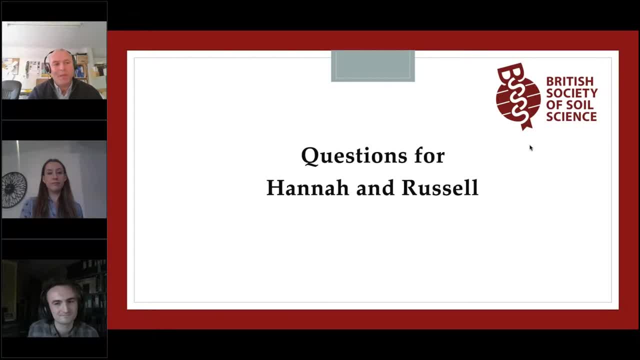 there is scope for it to really help with stuff. but i think if you're just sort of venturing down it um depends how, how brave you are and, i guess, your attitude to risk in terms of how much you want to take on. but i know when. if, looking back, when we started um, it was, uh, you know, a sort of 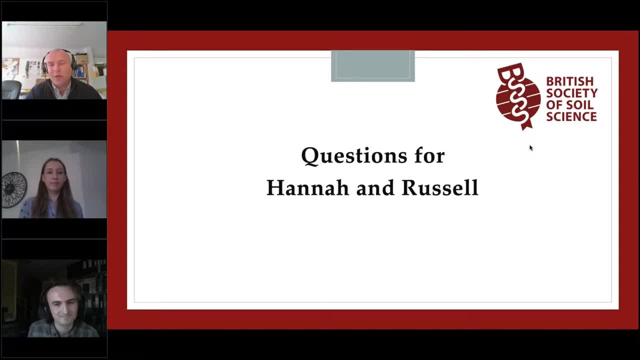 a softly, softly approach to you, gain more confidence in doing the operation. and if i look back at cover crops, the the first year we grew those we only had 40 hectares um for us to learn how best to manage. and then, once you you learn your various techniques, it makes it easier. 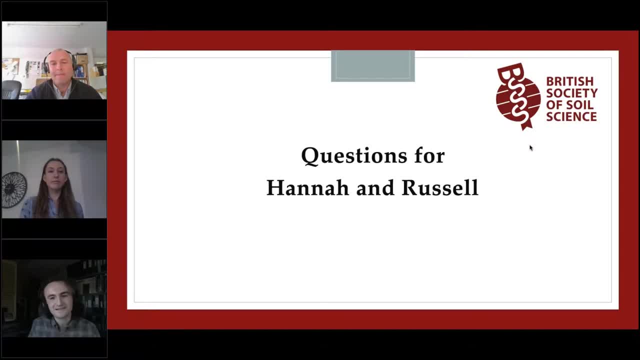 to roll it out into a larger area. thanks, that's it. thank you, uh. thank you, russ for hannah for that. um, so let's think not just about seasons now, but climate change over a longer time period and- and hannah particularly looked at this in her in her work- so, uh, regarding greenhouse gas, 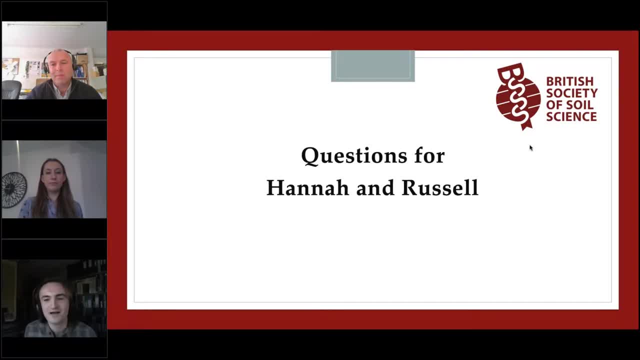 emissions, um and and specifically n2o emissions. have you any thoughts, hannah, on what you might see if you measured n2o emissions throughout the year? yeah, so n2o emissions are quite sporadic anyway, um, and especially throughout the year. it depends on fertilizer inputs and things like that. 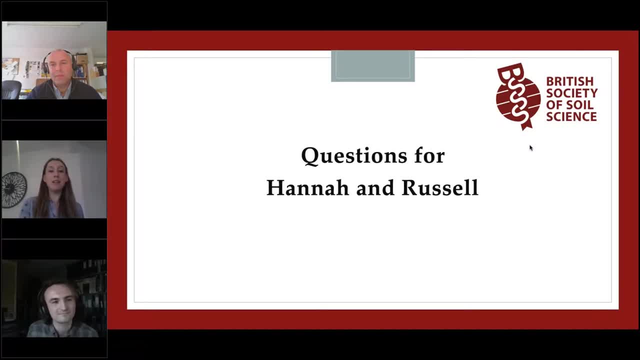 the time at which i sampled um. that would be the least impact of the fertilizers, and again, so n2o. um is released from soils through two processes, so denitrification and nitrification, which are determined by the amount of water in your soil profile. so i imagine you'd get so when i sampled. 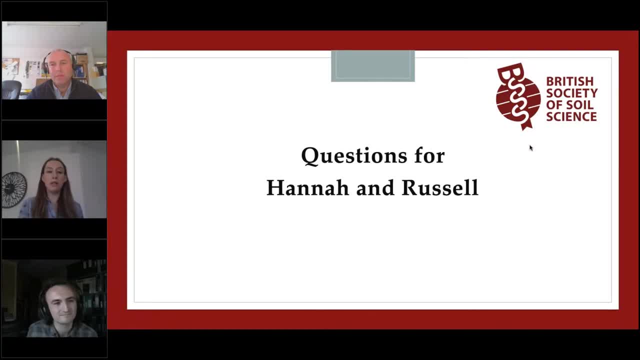 quite a large flux of n2o coming out because the soils are really wet and you've got that substrate availability as well, which is perfect for you, and so i think that's a really good example for the microbes. and then, i'd imagine, probably in the spring and summer, the levels 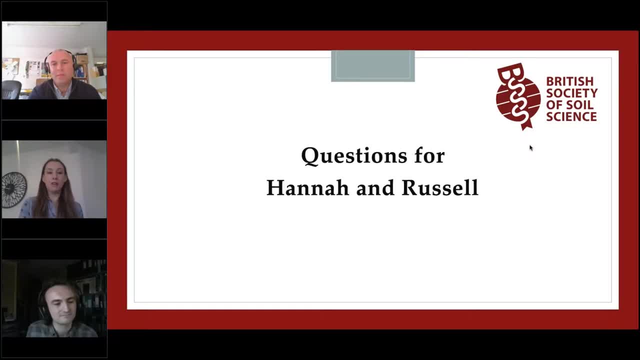 might still, might um go down a bit, but you'd still get n2o production. so that was something i wanted to look at actually in my phd but unfortunately ran out of time. but at rothland stead they've got the dennis system which can separate out those two processes. so throughout the year you can. 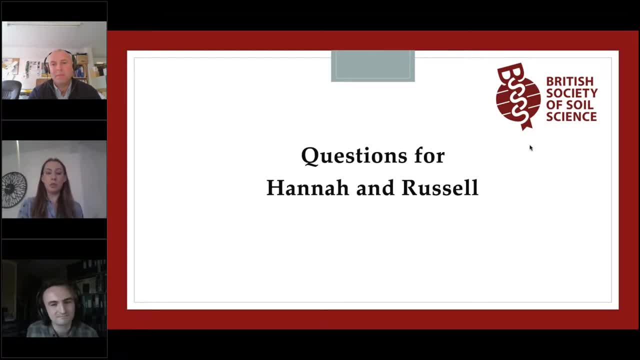 measure um, the dominant factor which is causing that n2o production. so it would be some really interesting future work. yeah, russell, have you had any experience with n2o emissions? uh, in your, in your sites there? uh, well, i mean a lot of. you know some of the information which we've probably seen has. 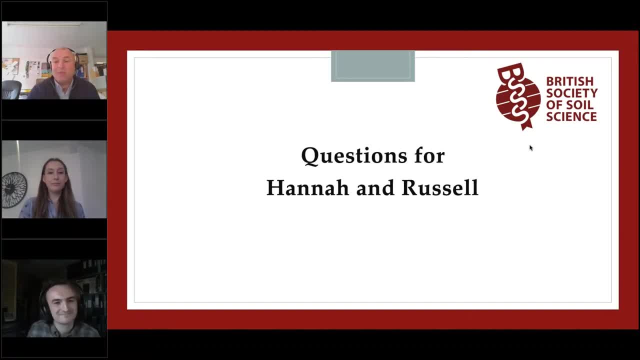 actually been. you know, hannah's been kind enough to to do sort of something, so we've seen some of the stuff which is which is going on, um, and that is quite interesting in terms of what you can physically capture or what you can, what you can reduce, capitalize um. 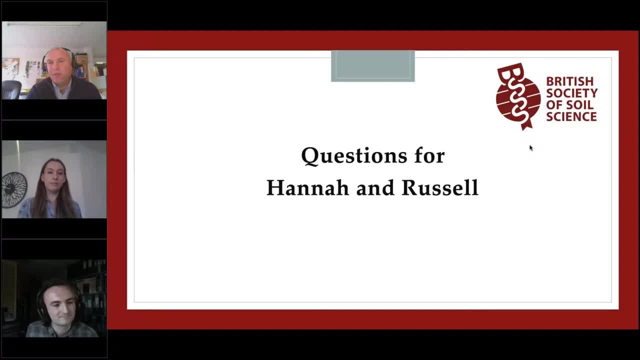 so i think if you can build up a data set for that sort of thing, it's quite a powerful, powerful tool at the end of the day. and it might just be that you know there's lots of talk around carbon etc and if you go across the states you know carbon trading is something. 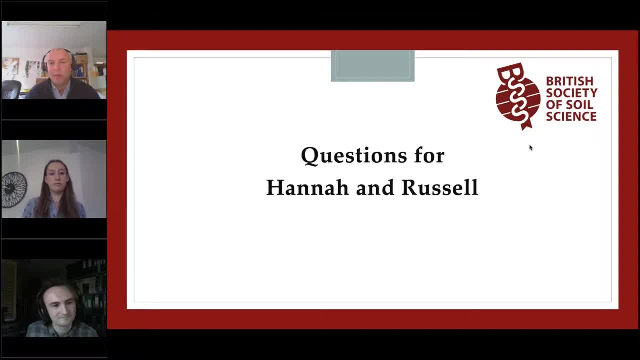 that's spoken about over there and the systems in place and there's talking about it happening here, um, but all those sort of things are- yeah, i think they're starting to come to the fall now, so i think they'll be quite interesting going forward. brilliant, thank you. so, um, we're. 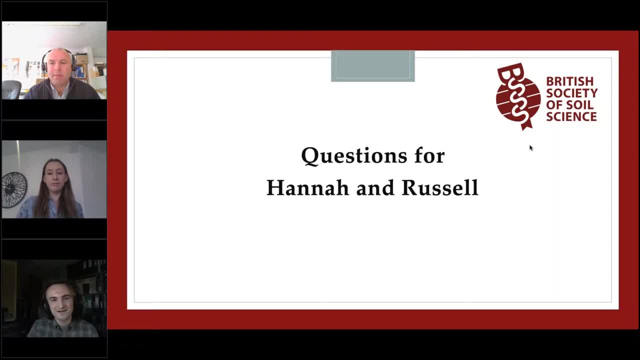 just uh past our 10 to 1 uh slot here. so thank you for your questions and we're just look forward to uh and uh looking forward to learning more about a few of the things that we've got uh coming in uh, so uh at this point in time. so we've got a series of questions about 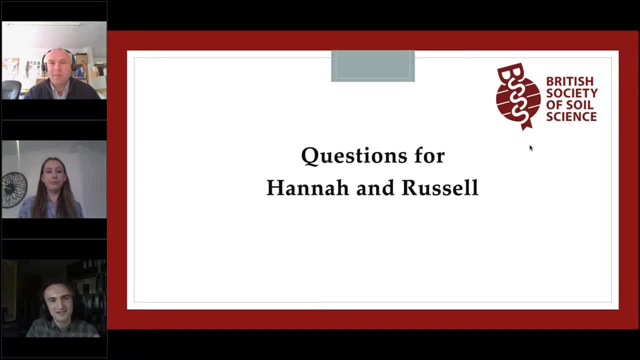 time and, of course, um, as hannah showed in her presentation, it kind of takes some time for some things to happen in in terms of the effects of no-till farming. um, so we've got a question here that: do you think that, given even longer time scales, uh, beyond 15 years? 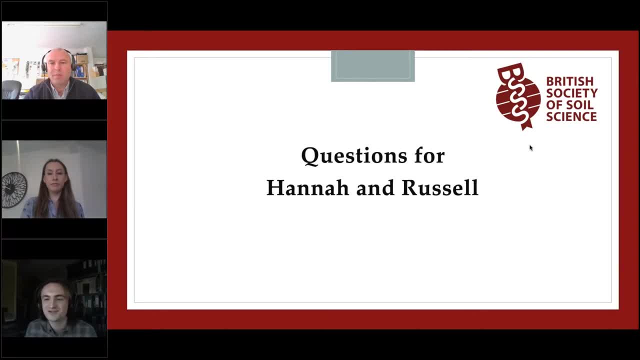 will no-till farming generate even more carbon sequestration, or do you think it reaches a cap at, uh, the next level of carbon sequestration some point? yeah, so there is the term carbon saturation. so the soil can only take in so much carbon, um, so within the uk samples that i sites that i went to, the maximum i could find was a. 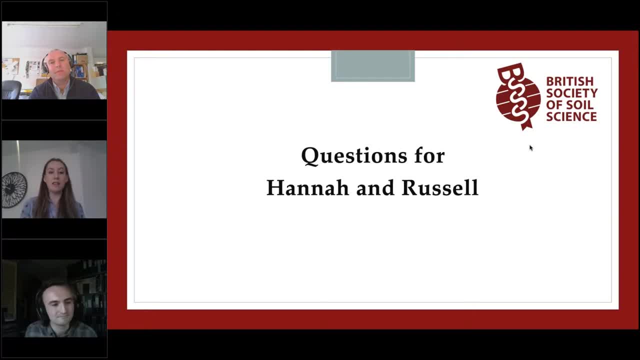 farmer who had been zero tilling for 15 consecutive years. so that was the data there that i had to work with and at that point it didn't show like a carbon saturation point. but i was fortunate enough as well to go over to brazil for a few times through my phd, through funding, through stars and 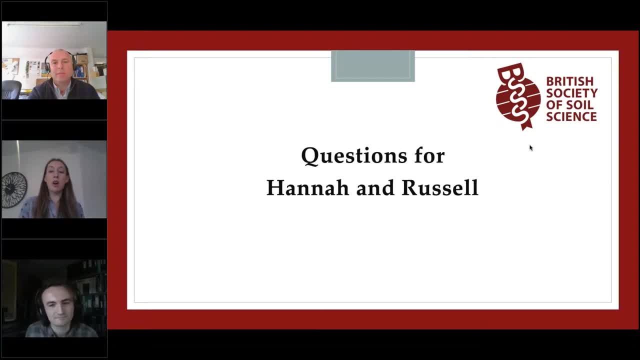 my supervisors project as well, and there are some farms that i was able to sample and they've been in zero tail for 31 years, and so i did again, did the sequential systems where uh from recently converted, and then i did seven years, 16 years, 21 years and then up to 30 years and it did seem in 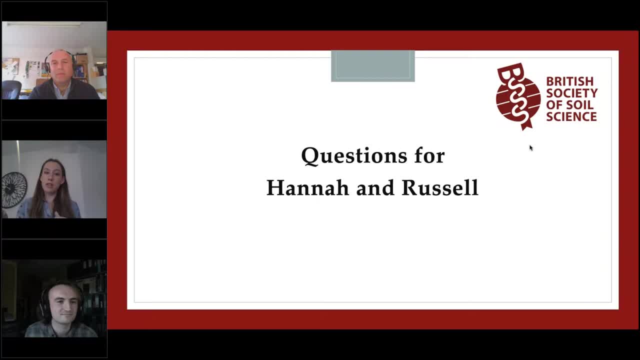 about 18, 20 years. it kind of plateaued um. so that was in those samples but it wasn't possible to measure that in the uk samples because of the availability of long-term zero-tilled fields. that must be a difficulty russell as well. the fact that we may be kind of 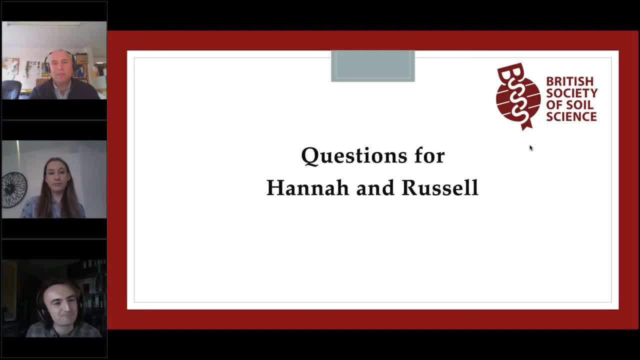 late to the party when it comes to no tool farming here in the uk. uh, well, to a degree, i guess it is. i mean, there has always been a bit of a hangover from what it was originally used in sort of the 1970s and early 80s. is that, you know, some people experience a. 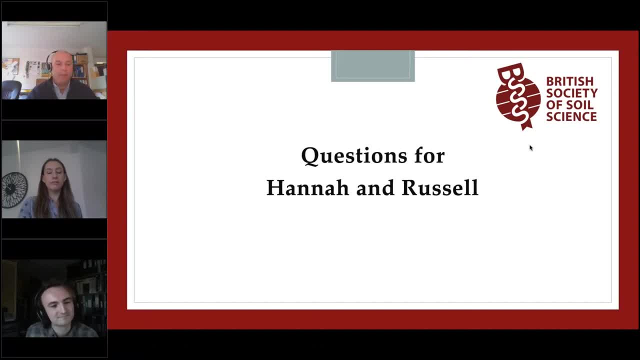 very different approach to what we're doing now, um, but i think that in terms of you know, there's a thirst research in it, um, there's a real generating interest with people wanting to understand. the emphasis is more now on soils, really as well, whereas there's uh, as it's a 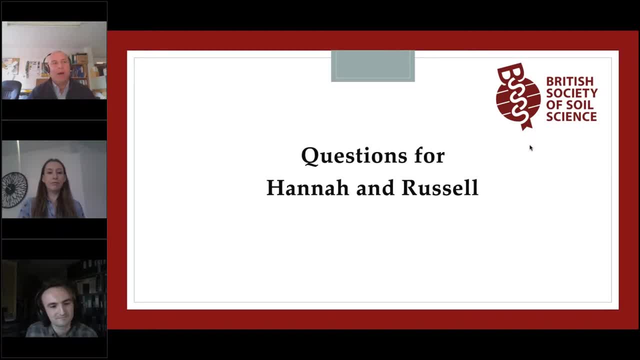 really healthy. it's almost. there's lots of information, um, um, once you can't get enough and it's a, it's a, it's a. really. you know, i know i'm sort of speaking to the right audience, but, um, there is a real healthy obsession with 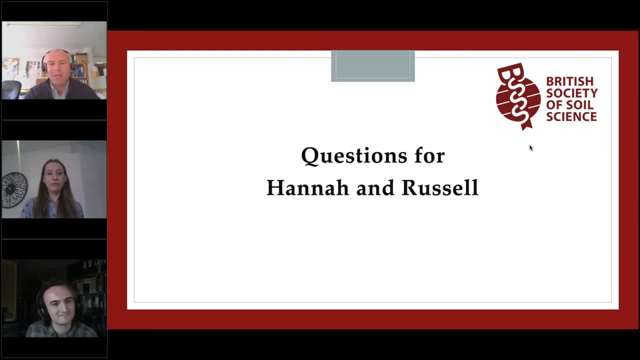 trying to understand what's going on with soils and what they can do, what i can capture, etc. um, are we a bit late to the party? i? i don't know. there's there's certain parts of you know, probably europe is probably more challenging because of the climate than it would be if you. 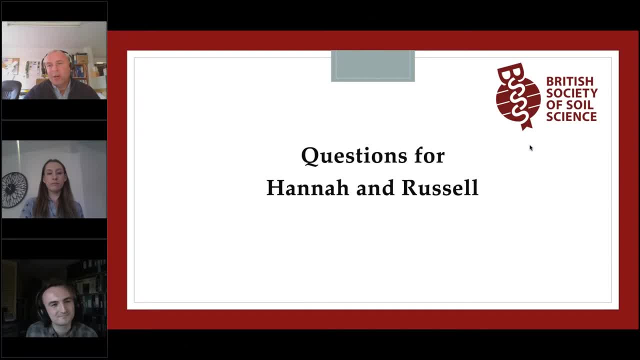 compare it to the south american countries. those are tropical types of systems out there. it's probably maybe a bit easier to adopt out there. um, you know, uk is challenging but there's some- you know some brilliant practitioners. you know guys that are a lot further down the road than me who, uh, have learned a lot, understanding what the limitations are. 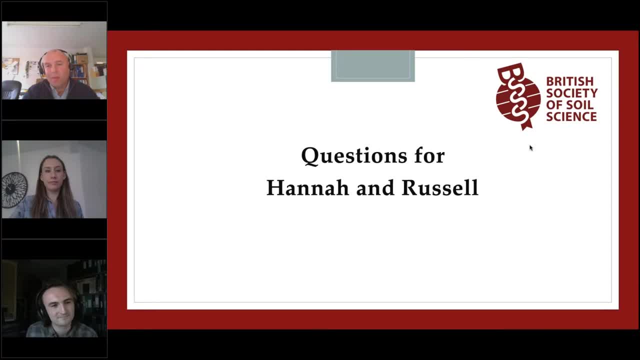 i think that's the key bit is: you know what are your limitations of how far you can push stuff. you know some people would say that actually cover crops- don't, don't see them, so they're not for everyone. um, and i think that's the key bit with it is it's not a one-size-fits-all approach. 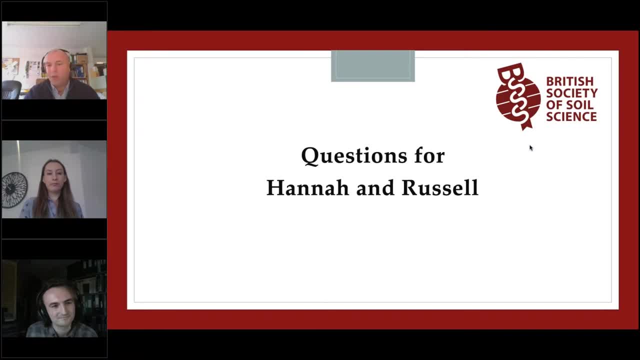 you know there's a different systems for different farms, um, different approaches, stuff and what works for you really, but i think things go in the right direction there's. there's lots of good people doing some really good stuff across the uk. yeah, absolutely of course, and uh, maybe if 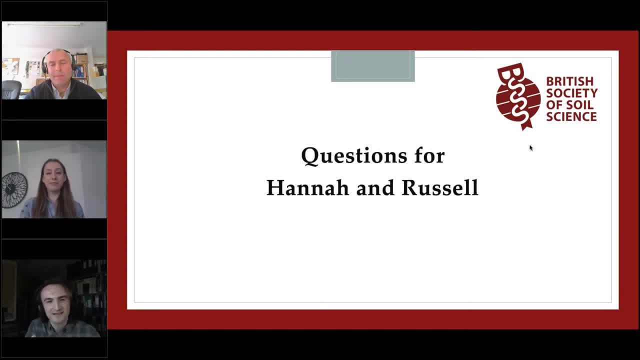 we are late, uh, to this um, and there's a question here particularly about speeding things up with different crops or different practices enhance or speed up the rate of which- uh, in particular with this question- optimum soil connected porosity is achieved. can we speed that process up? um, yes, i definitely imagine so. so that wasn't the particular focus of my study, but 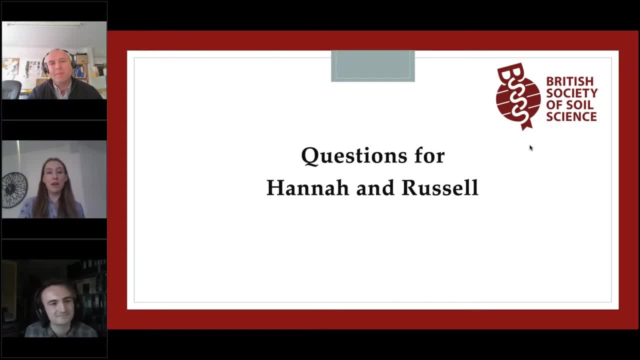 um, i don't know if you guys have watched the documentary on netflix, the kiss the ground, but that was brilliant in terms of showing the effectiveness of the process and i think that's something for everyone to be so inspired and其 want to see: uh in in your kind of applied practices, muscle in in the field. 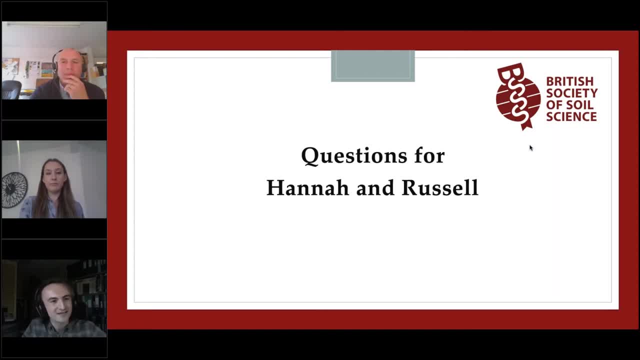 fields. are there ways that you know with your colleagues, of course, ways you can speed up the process or kind of help the process along a bit? Yeah, I think it's. I mean, there isn't a simple sort of well, a simple solution is going have a look with a spade? is understanding what? 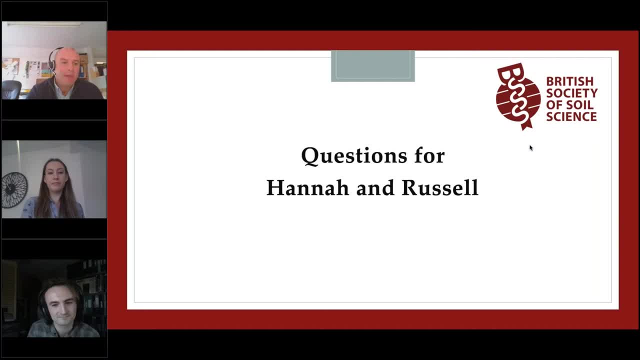 what you've got underneath, I think, is the key bit. you know in terms of how good is your soil structure in the first place, and that gives you a good indication of where to go. a variety of crops, I think, is you know it's really healthy, I know. certainly, when I did my Nuffield there was a 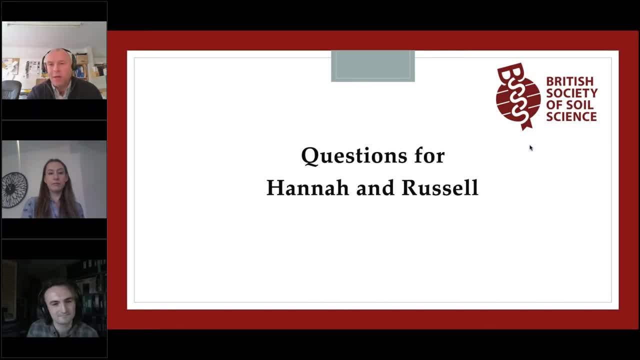 a guy in Argentina spoke about the importance of different root systems, not just within a cover crop but within the growing crops as well. so you you've got that constant mixture of different roots, different associations. I'm probably still thinking about sort of we were rotation wise years ago. it was what I call the non-rotation rotation, which was wheat and all seed rape or 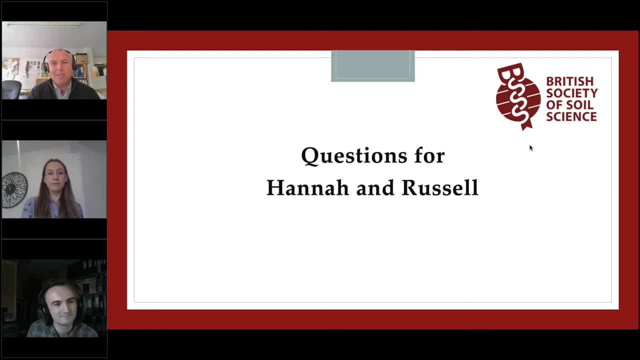 maybe two weeks in all seed rape and the challenge you get with that. when you have rascals in the rotation you can build your mycorrhizae association but there's no association with something like all seed rapes. you can build it and then for that period of time it will drop. so you can possibly understand sometimes if you're 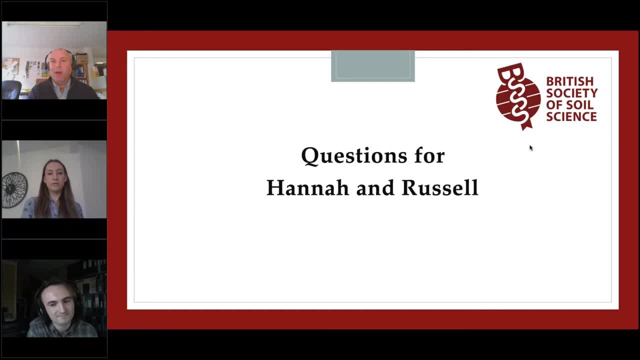 growing a lot of all seed rape in a very short rotation. why something like is not not healthy for mycorrhizal fungi. so yeah, having different root associations. you know we companion crop with with all seed rapes for various reasons you know. see that different root association going on with. 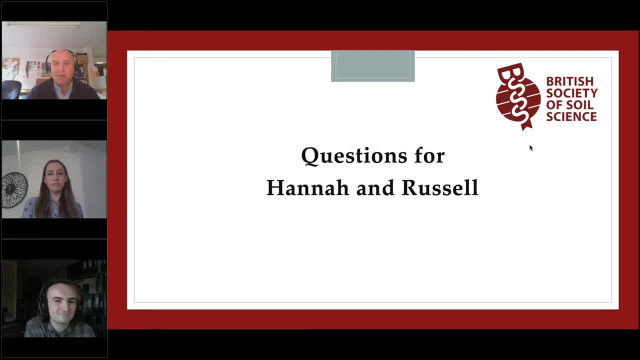 there. I think you know keeping residues cover crops, you can sort of try and move along quickly. I know people talk about soil, organic matter, and that's the hard one is that that you can't sort of build that overnight. that is a slow process, but you can certainly help it. 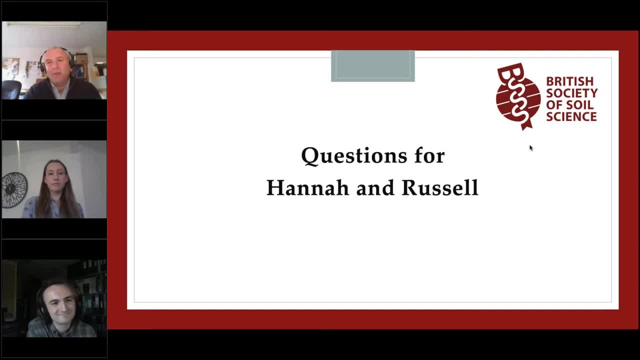 along along its way a bit quicker and sometimes just being being a bit brave and being brave, but but not so not pedantic, I think is quite important when it comes to trying to move things on absolutely well. thank you so much for everyone, for all of your questions. I mean, there's so many. 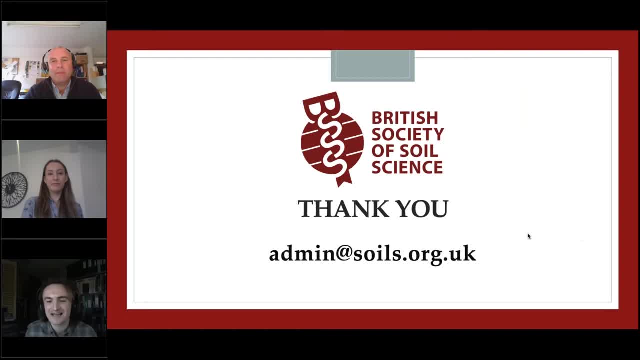 that we can't get through, unfortunately, but I'm sure we can discuss this at a later date in the society. but there is one final question I want to ask and and that's quite an honest one: why is? why? is there no consensus on zero tillage? why is it still a matter of discussion? I think 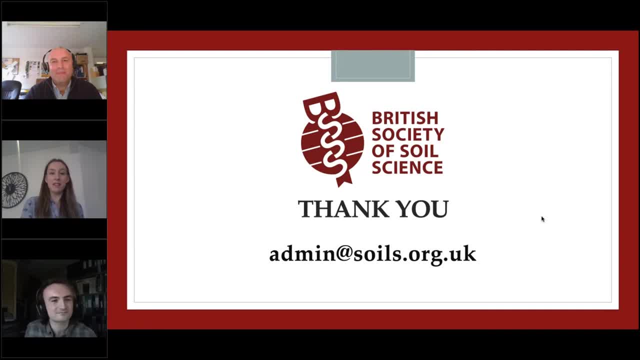 personally what Russell was saying, and that you just need to get a spade and see what you're working with. it can be really site specific in terms of what you've got to work with and in terms of, again, different climates and things. if it's really really waterlogged to start with, you're just not going to be able to get zero till. 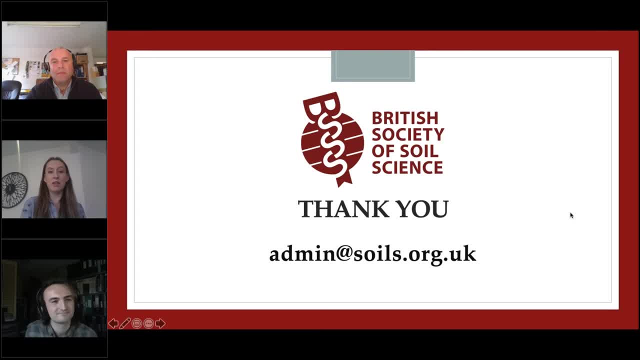 to work. so it is site specific and you just need to see what you've got really. and, Russell, yeah, I'd echo that completely, it really is. I mean, you could have some fields which, for whatever reason, it just doesn't work on sometimes, and it is sometimes the hard, the 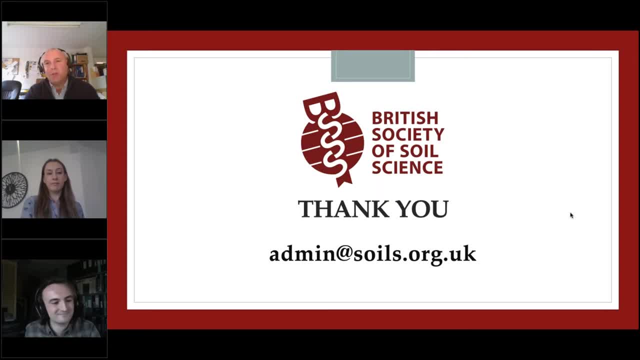 hard bit is if you've been doing a lot of tillage. yeah, once you, once the combine's out the field, you're going out, you're cultivating and working stuff down. it's probably one of the the really the hardest things is to sit there and almost do nothing when everyone else is doing stuff around. 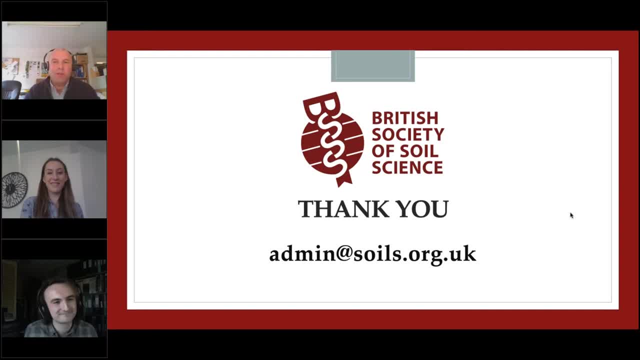 you and wonder what you should be doing, and that's that's quite hard. it can be quite a hard thing sometimes, and having staff on board as well is pretty good to try and understand what you're trying to achieve on the journey, on what you want to do. so, yeah, and let's say again: it's about it. 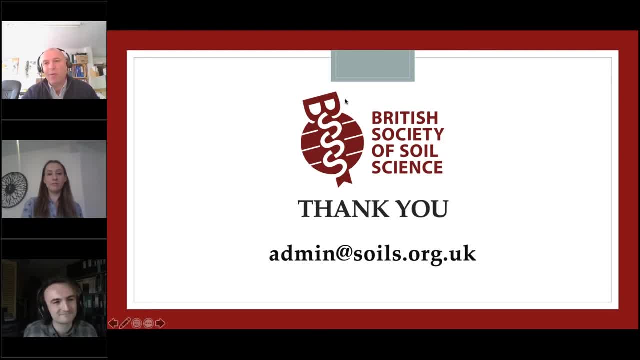 just goes back to just understanding what's going on. you know within your field, what you're kind of know within your fields really, and you get a pretty good picture pretty quickly. um, and you know, certainly when you listen to some people talk about it, they you know i can dig a hole. i can't explain what goes on in a hole as well. 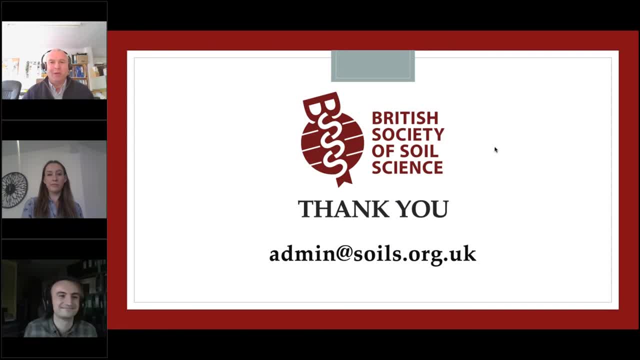 as someone like rob simmons or philip wright will do, and it's quite good if you can go to those events where they point out what's going on. um, you can try and then take it away and understand what's going on in your own fields. 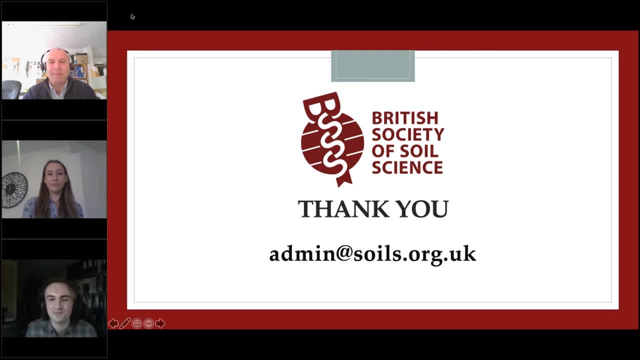 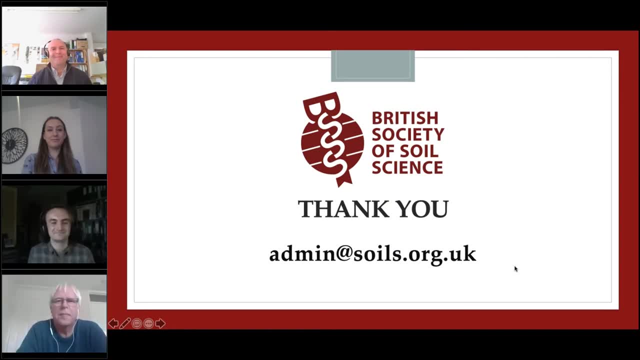 yeah, it just shows the importance of continuing to zoom into soil that little bit more. thank you so much to russell and to hannah and uh hand back now to wilfred. thank you all for very interesting in discussions. so on behalf of the british society of soil science i want to express our thanks to both. 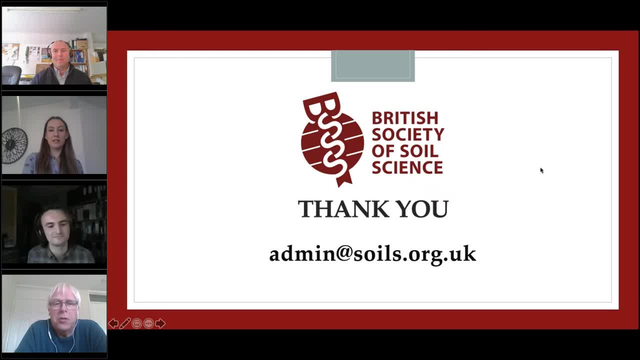 hannah and russell. i've taken a little note, russell, of your forecast. this was probably the worst year that we can have, and i hope that that's as accurate as your first prediction was. further than information on zero tillage, um, there will be a special issue in the european journal of soil science.